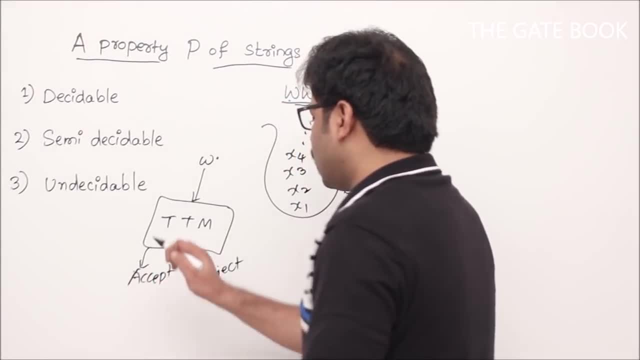 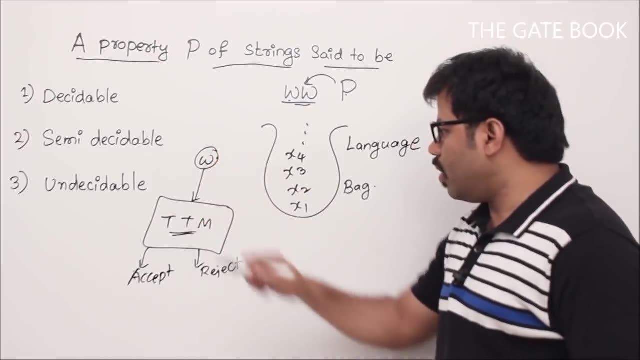 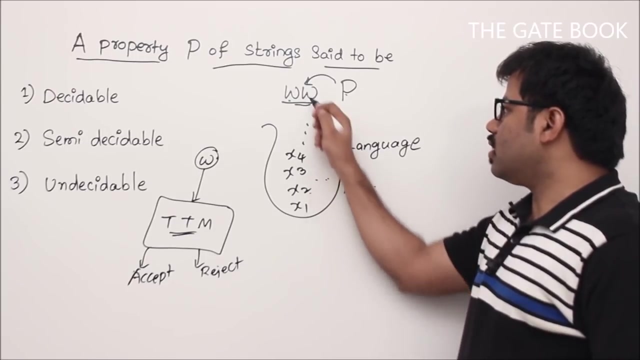 reject. Let us use accept, only Accept and reject. Now example: let us say: this total Turing machine is designed such a way that whenever you give input w, if the w is part of this bag, if this w is a part of this bag, means this string has this property. then it is accepting. Try to understand. 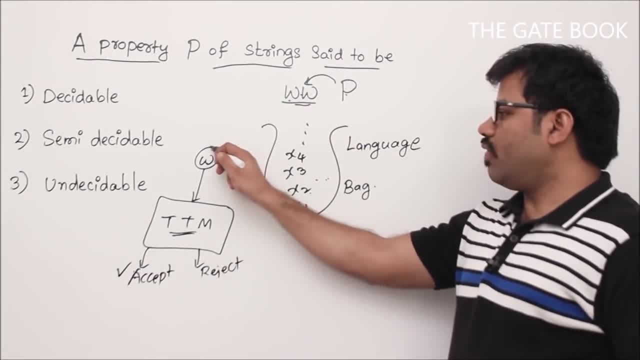 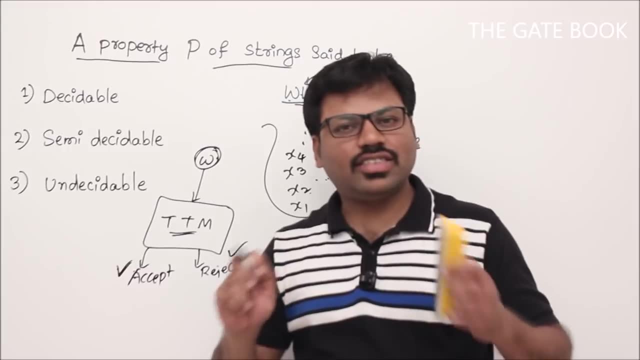 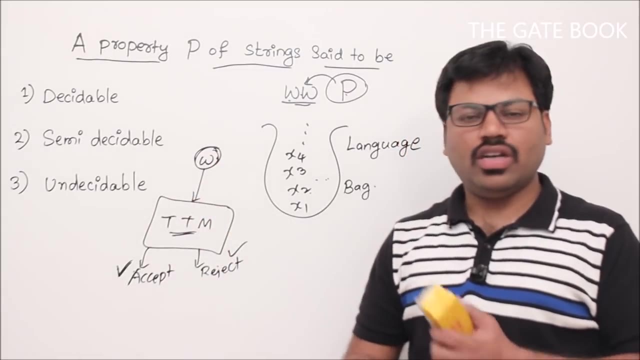 The connection between property and this total Turing machine. Whenever a given input is having a property p it is accepting, Otherwise it is rejecting. Then such total Turing machine if you have, then we say that such language is decidable, Otherwise such property is decidable. 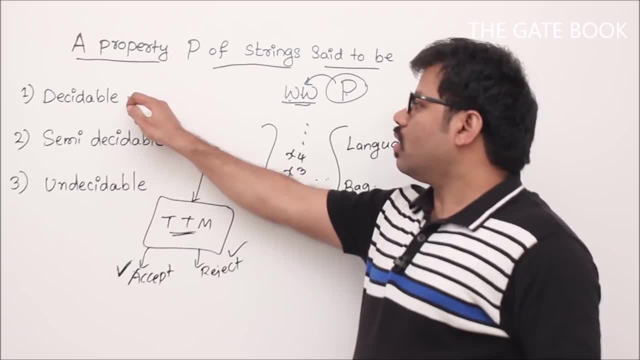 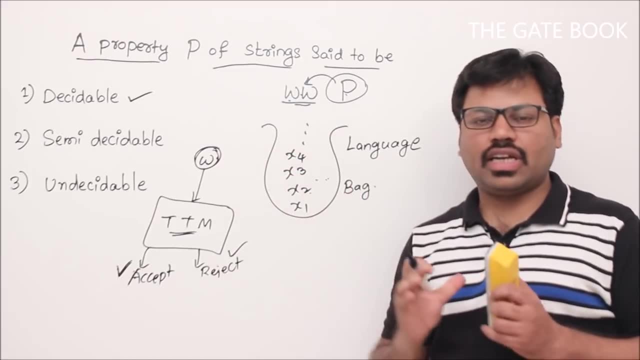 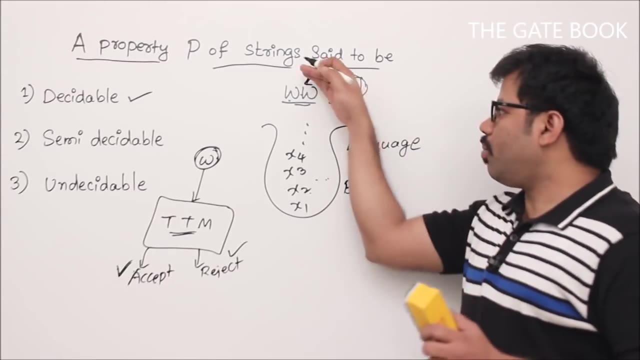 Here property is nothing but language. Finally, decidability is that Recall again, When you have a, let us say you are collecting all the strings which are having a property, They form a language. Here I use language and property interchangeable: Having a property. 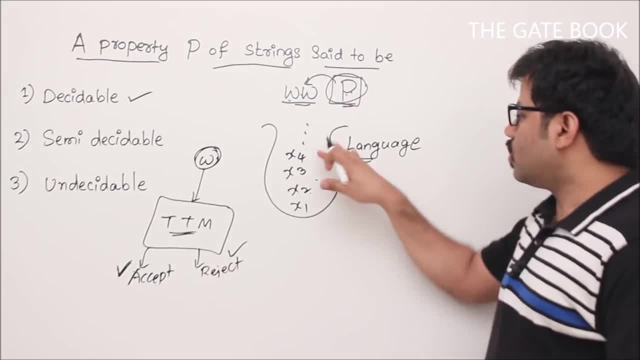 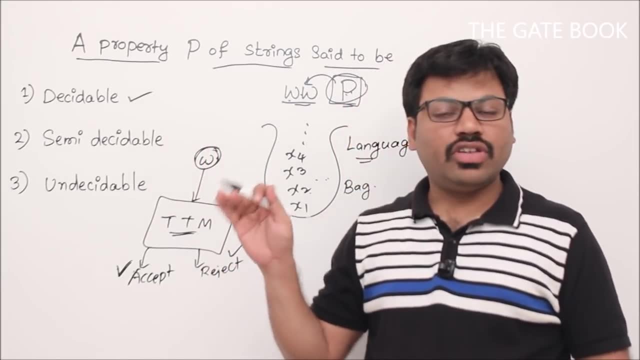 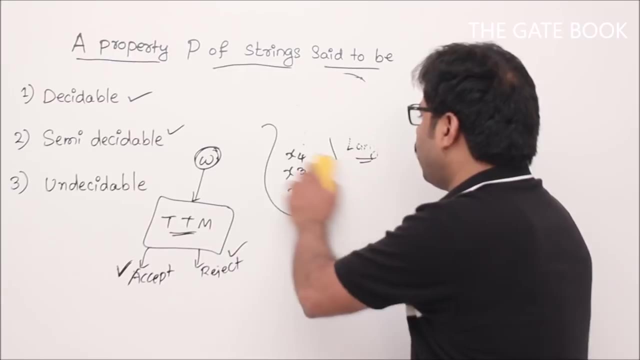 otherwise having a language is same for me. Such language is accepted by some total Turing machine. then we say that it is decidable. which is language? That language is decidable. Now what is semi-decidable? Same problem Example. let us take another property. 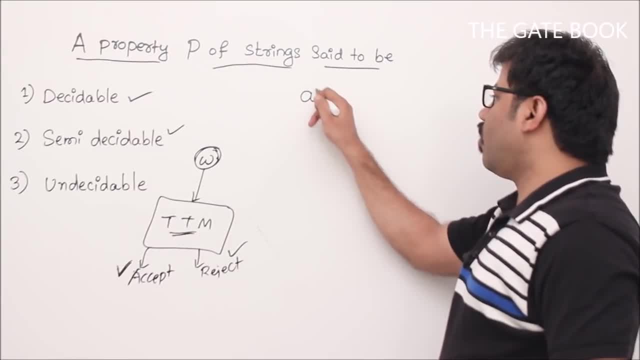 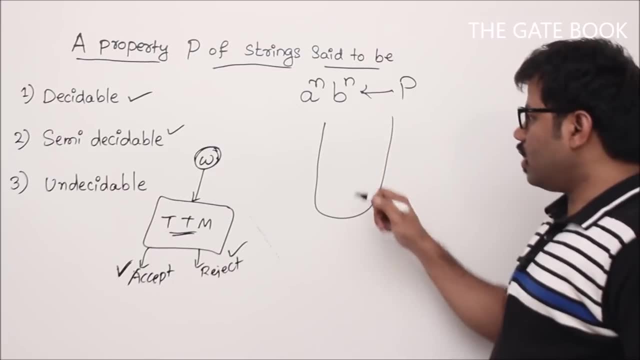 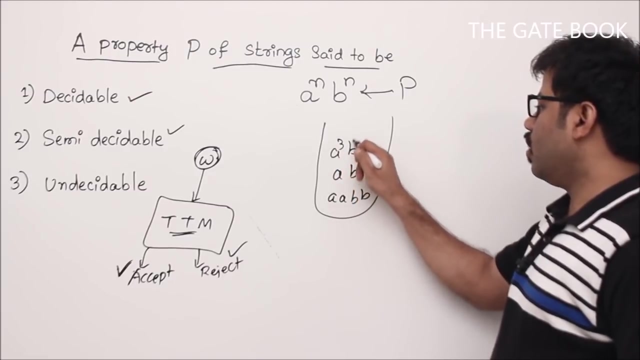 Let us say you have a property that is being in the form of a power n, b power n. So this is your property. Now, collect all strings which are in this form: a power n, b power n. Example: a, a, b, b, a, b, a, cube, b, cube in that way. So collect all such strings. 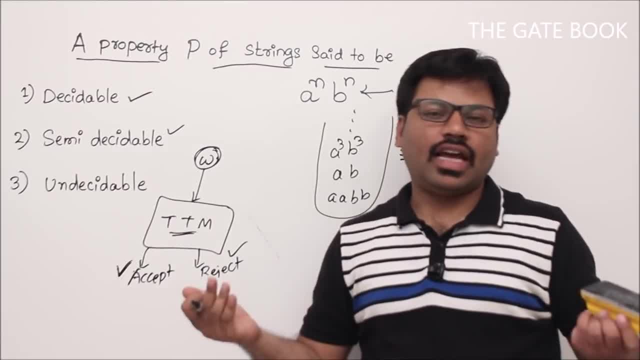 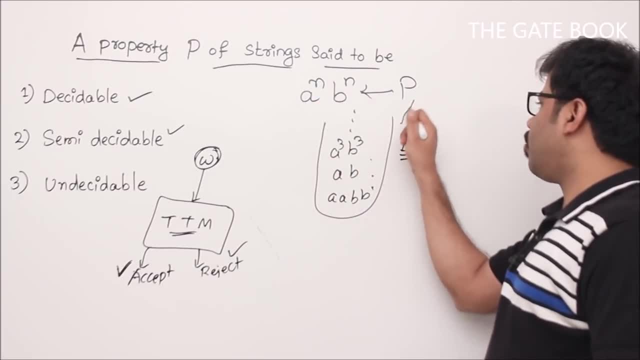 It forms. what A language. We know that That language is nothing but a language in the form of a power n, b power n. Here property is nothing but being in this form. This is the language. That is the relation between property and language. So property and language are almost same, They can be. 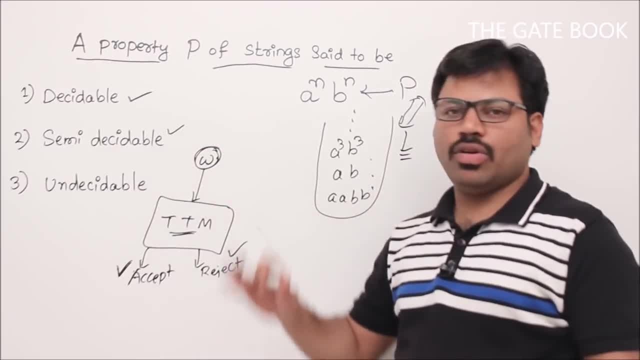 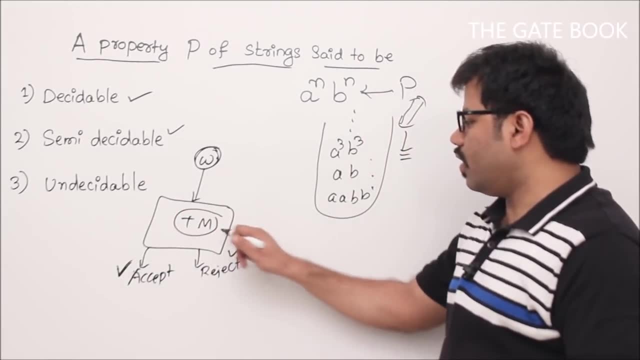 used interchangeably. So property and language are almost same. They can be used interchangeably. Now such language is called semi-decidable. if you can show Turing machine for that, What kind of Turing machine we have to show? If we say that this is a Turing machine for this property, that means 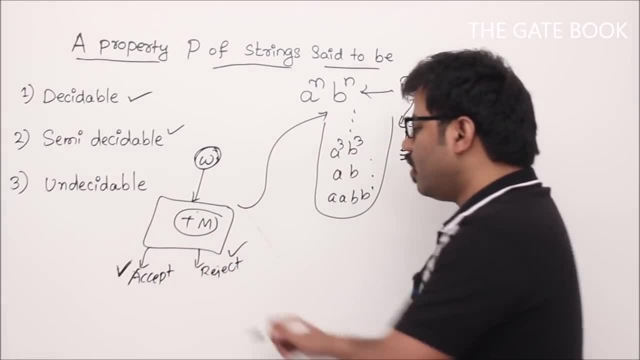 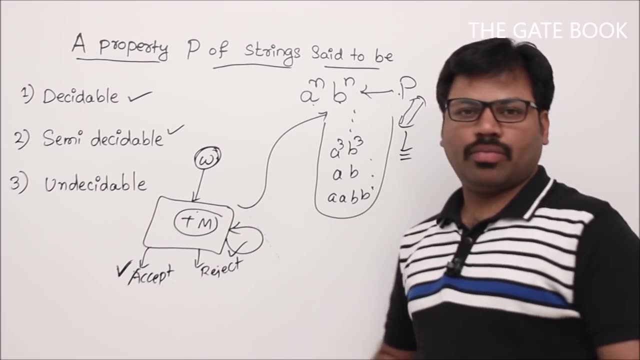 if some input is given, it should accept whenever that input is in the form of a power n, b power n, because that is a property. Otherwise you can loop, Otherwise reject, Not a problem. Such a machine if you have, I do not bother. if you loop, I do not have any problem. But whenever the input 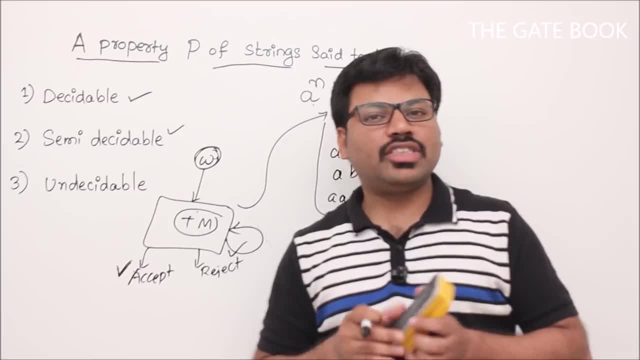 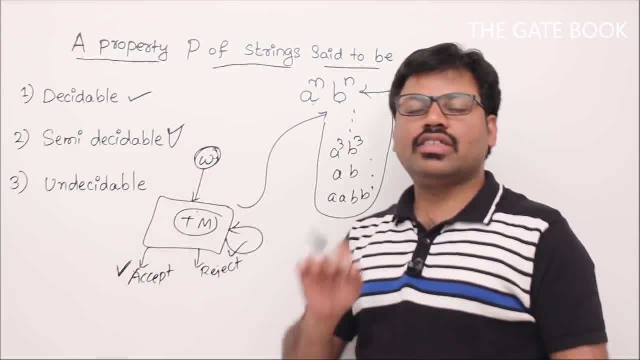 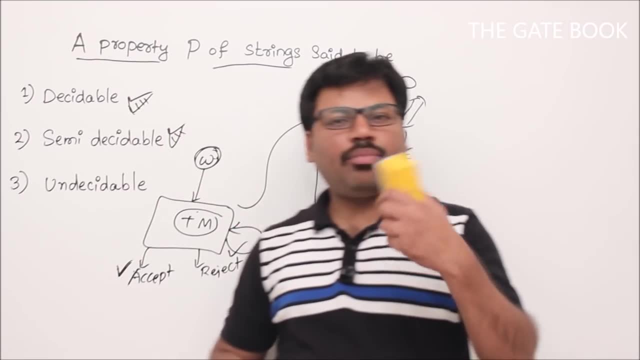 then we say that such language is semi-decidable. That is a fundamental definition of semi-decidability. Now, finally, you understand what is decidability, what is semi-decidability For any property. if you show a total Turing machine, then that is a decidable property. 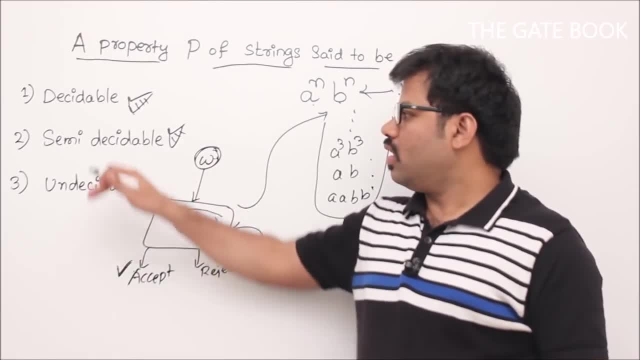 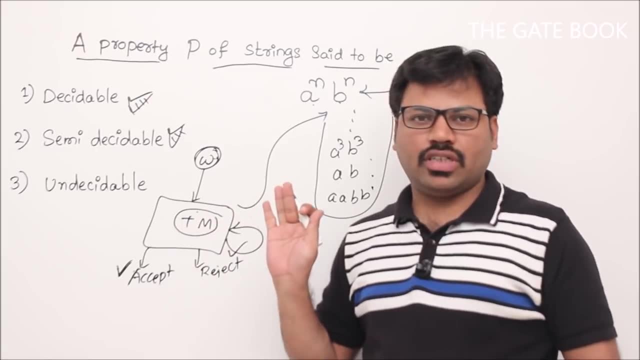 For any property or a language for that property is for that. if you show to just Turing machine- I do not know whether it is a total Turing machine or not, But if you show a Turing machine, then that property is called semi-decidable. Now one more thing is undecidable, So 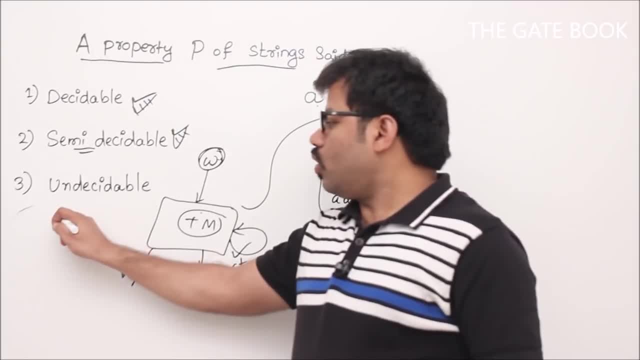 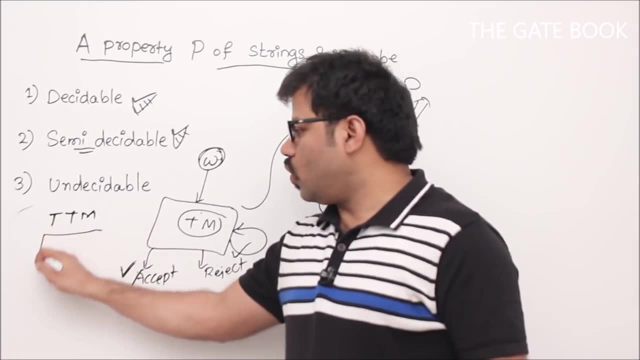 a property is called undecidable, then there is no total Turing machine for such problem. So we know that problem is nothing but a language. now, So for a language, if there is no total Turing machine, then we say that is undecidable. Simply decidable is quite opposite to. 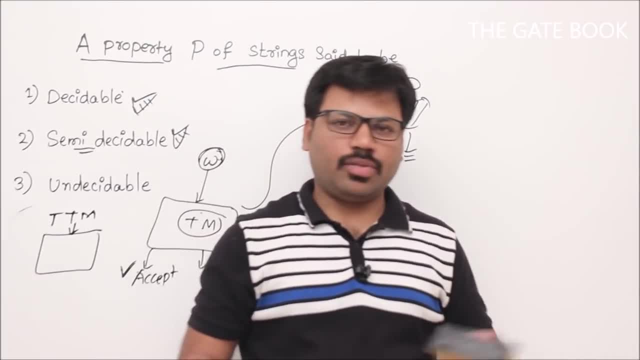 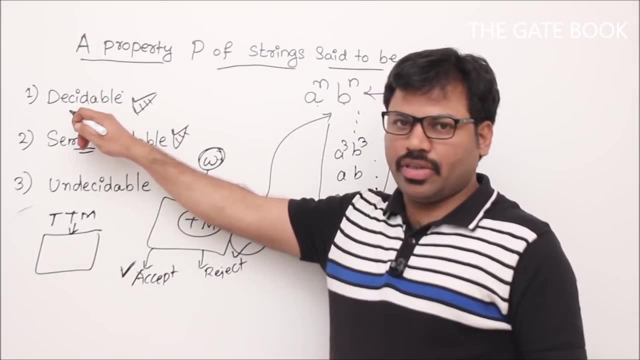 undecidability. If something is not decidable, then it is undecidable. Now let us summarize decidability, semi-decidability and undecidability. If a problem has a total Turing machine, that is decidable problem. If a problem has just Turing machine, I do not know anything else. 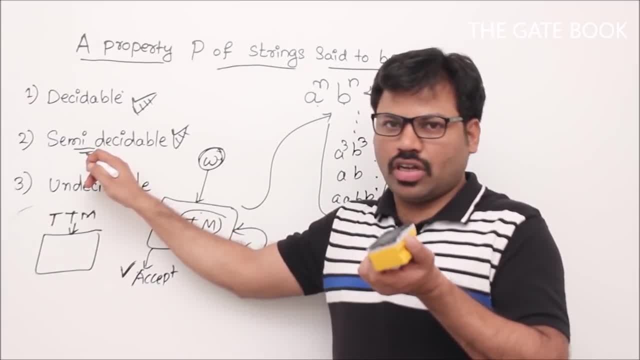 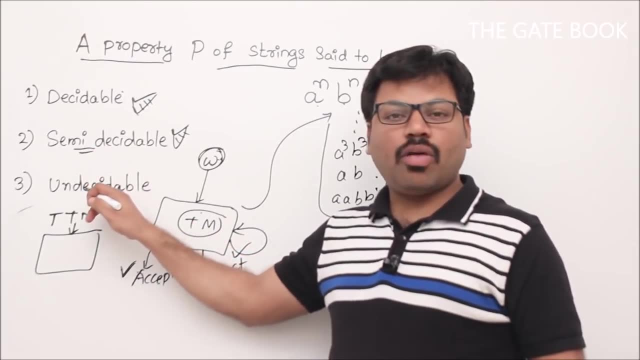 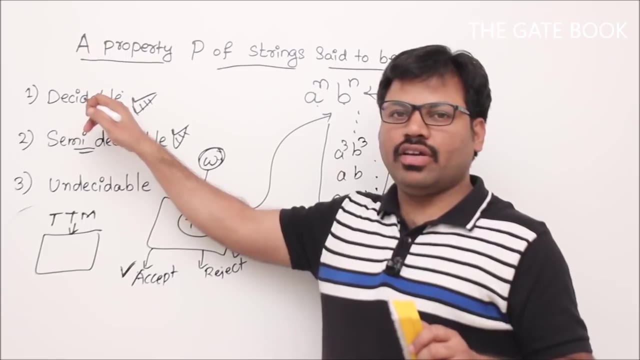 then that is semi-decidable. It might have a total Turing machine also, I do not know, But definitely I got one Turing machine. then that problem is semi-decidable. Now third one: there is a problem which does not have any total Turing machine, then that is undecidable. If it 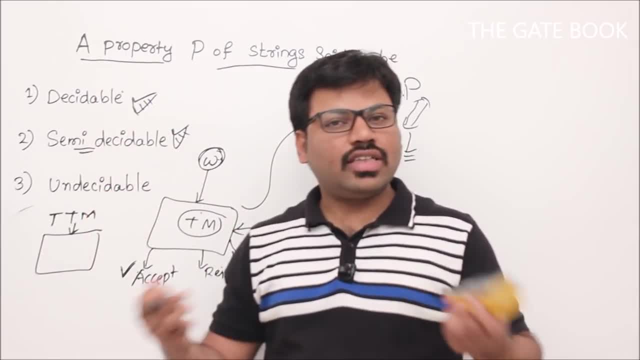 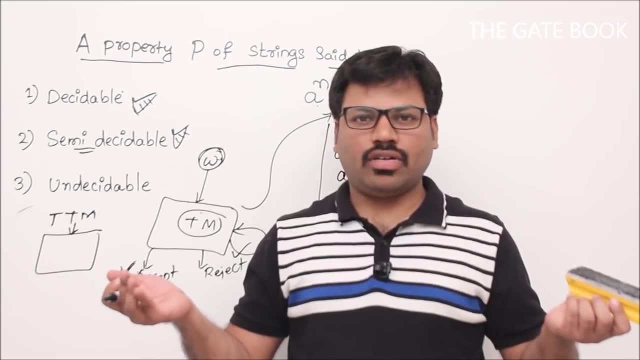 has total Turing machine, that is decidable. If it does not have, then that is undecidable property. So blindly remember: any property is not decidable, that is undecidable. Let us talk about universal Turing machine. To understand universal Turing machine, first of all: 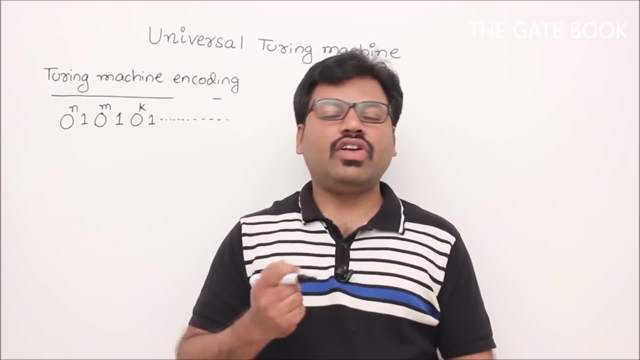 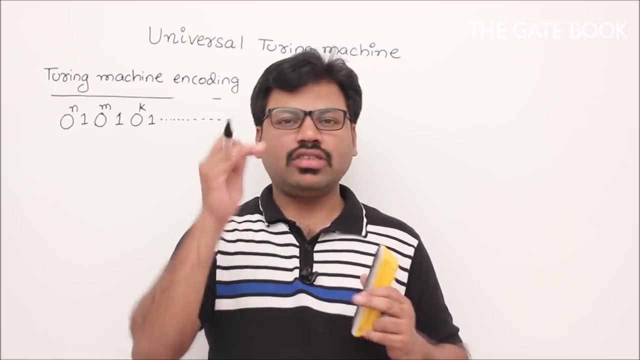 you should understand what is the encoding of Turing machine. I will tell you what is encoding of Turing machine. You have a Turing machine. Having Turing machine is nothing but having description of Turing machine. That means what is your set of states and what is start state, what is? 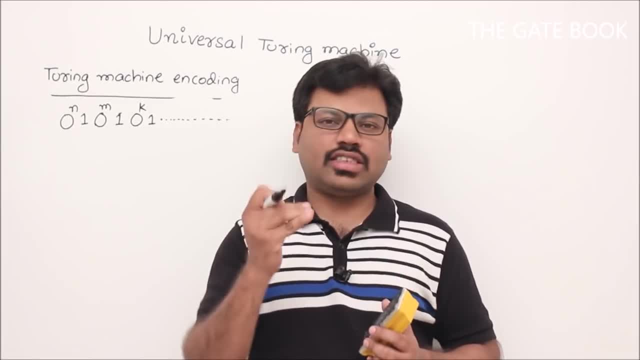 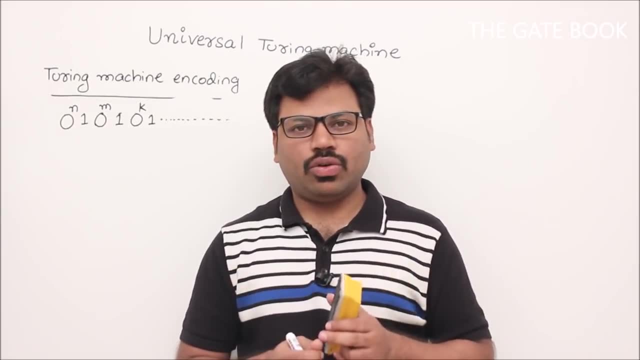 reject state in your machine and what is the transition function That details is called your description of the Turing machine. Now, given a description, we have to convert that into encoding. I will show you how to encoding. especially, let us focus on binary encoding. 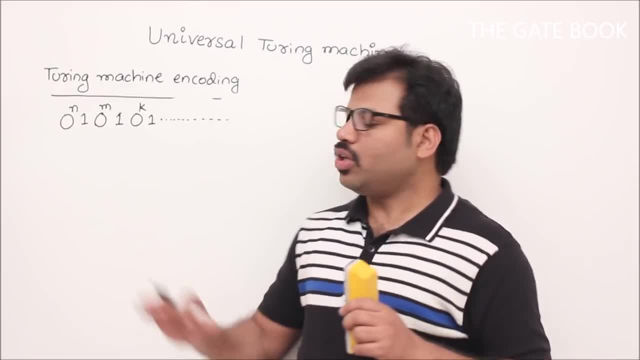 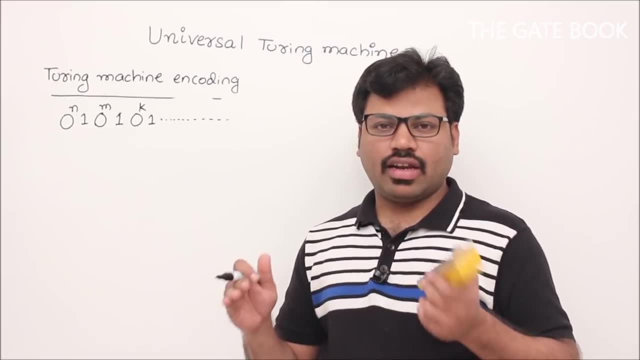 And one more thing: exact encoding scheme is not really important, but you should know that, yes, we can do binary encoding If you know that that is sufficient. So let me show details of encoding in a you know a ways way. That means you know, not in an unclear way, not in exact. 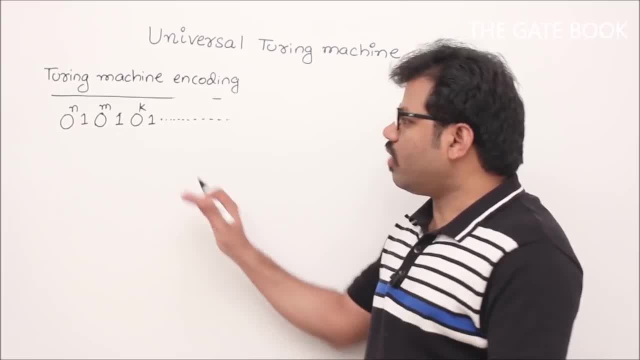 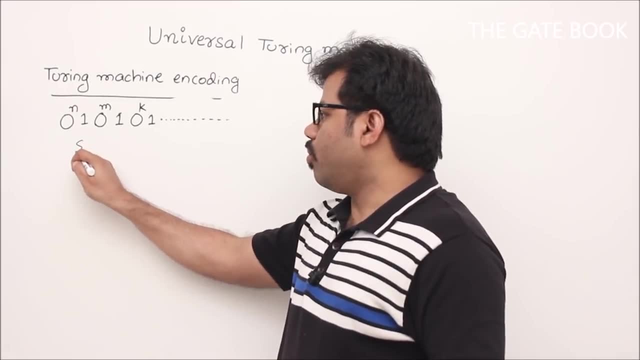 way, because exact details are not really required. So let us take one simple example. Let us say you have a Turing machine, Tell me some important details which I want to encode. So input alphabet correct. Let us say your input alphabet is A, comma, B and the states are: 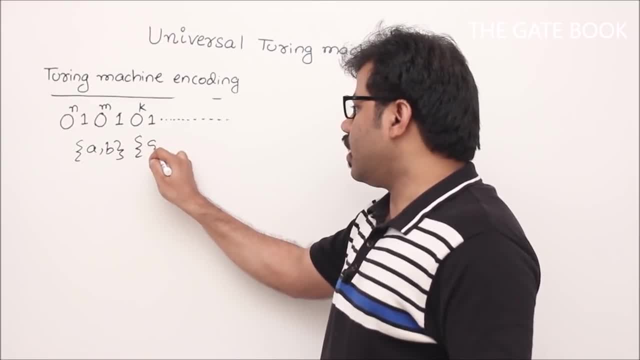 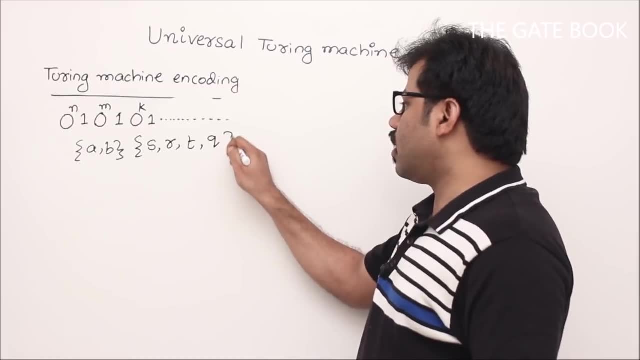 let us say there are four states. They are, let us say, start state, some reject state, some final state and some one more state. Let us take that state as Q. These are all the states. Now I am just representing your Turing machine. I am writing the. 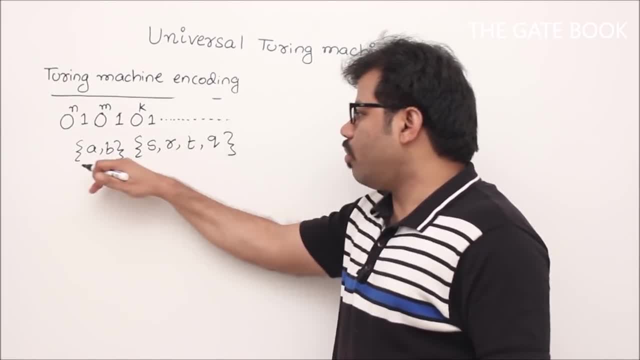 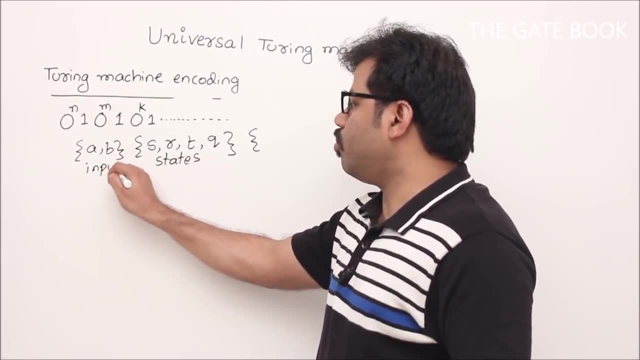 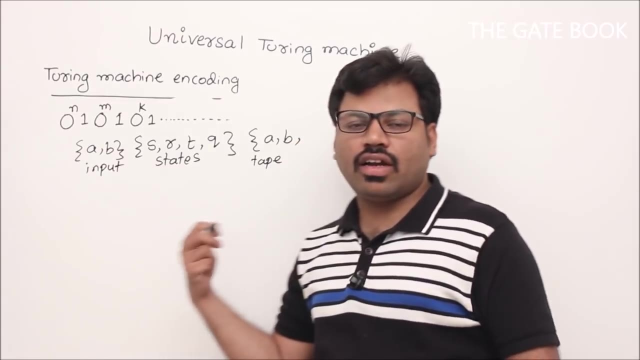 description of your Turing machine: States input alphabet. What is state alphabet? Let us say this is, you know, states Input Input symbols, Tape symbols. Let us say: tape symbols are A. that means tape symbols are symbols which you can write on tape. Input symbols are part of tape. 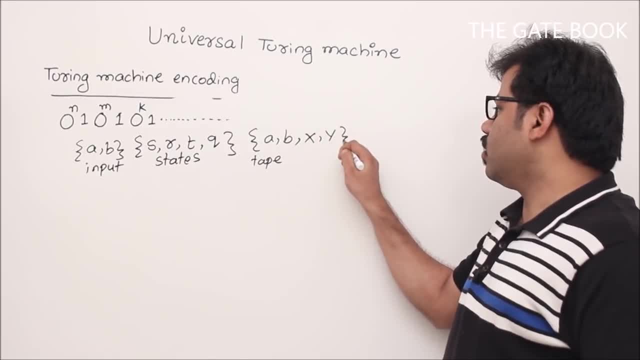 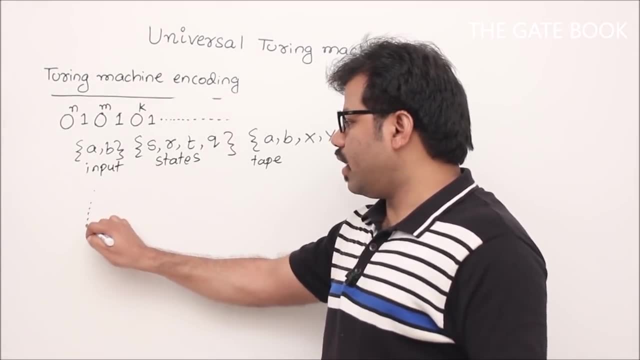 that you should understand: A comma, B comma X comma Y, let us say So. this is called description of your Turing machine And what else. Some transition function, correct? So you see transition function later and after that we know that there will be a left-hand marker. 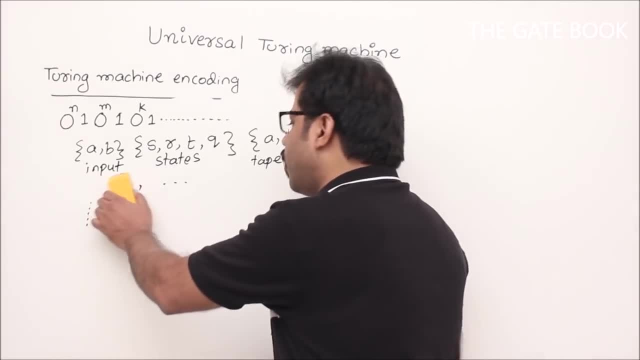 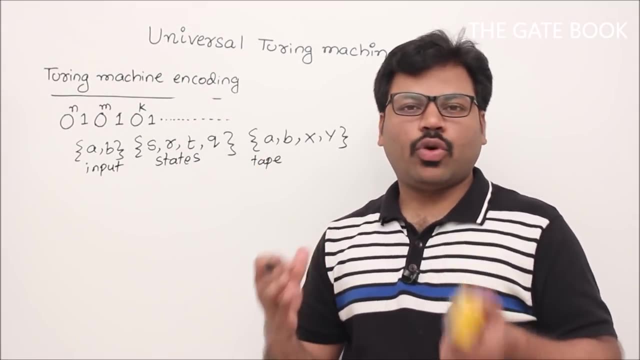 After that you know some extra stuff. right, They are all not so important because I would like to show only important details. Let us say these are all essential details of your Turing machine. I am going to encode them. Example: let us say your states are: S comma R, comma T, comma Q. 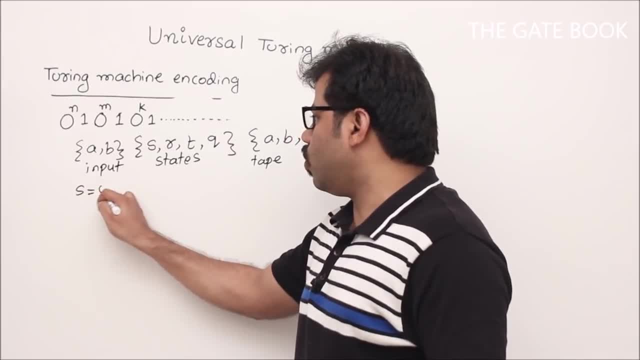 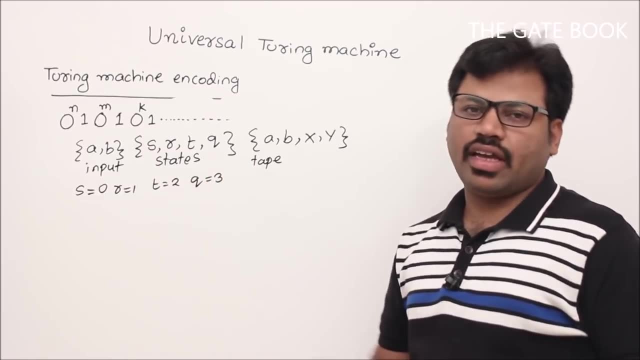 Let me number them. I give numbers like this: S means 0,, R means 1,, T means 2,, Q means 3.. It is an example. You can try any way. Next, you have you know tape symbols, right, Let me cover tape. 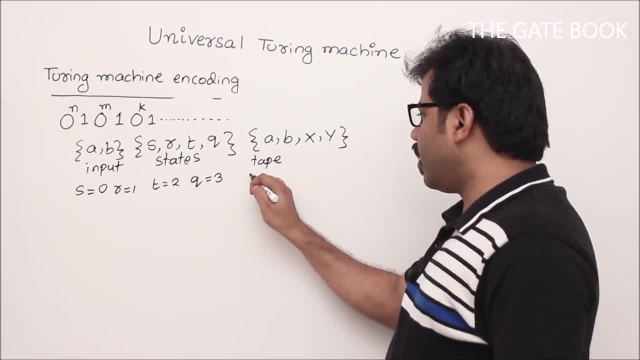 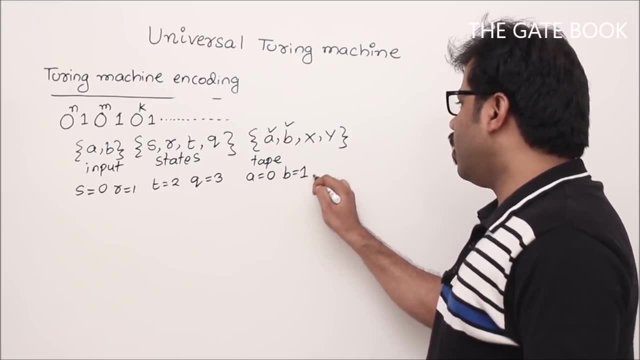 symbols. The tape symbols are A comma B, comma X, comma Y. For first two are, let us say, input symbols, right, For A, I give a number 0.. For B, I give a number 1.. And for X, I give a number 2.. 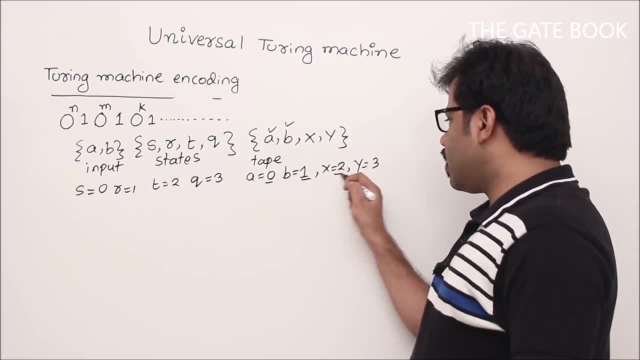 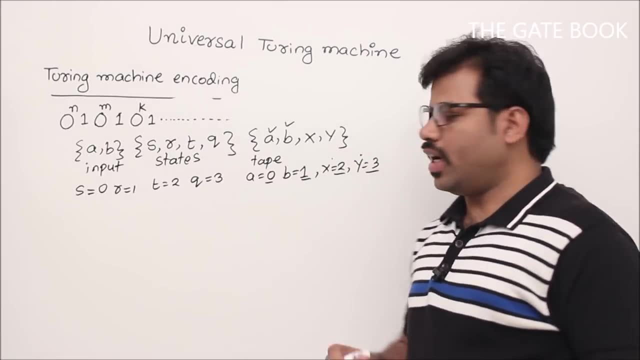 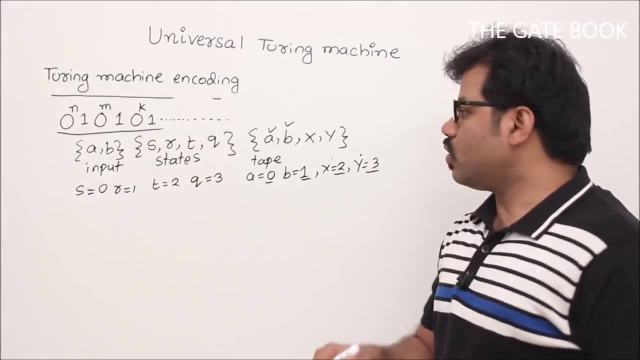 Y means 3.. In that way, so by these numbers, I can understand that this is one symbol. this is one symbol. 3 means one symbol. 2 means one symbol. You will understand slowly at this moment. let me number like that. Now I am going to write this kind of binary format that is going to: 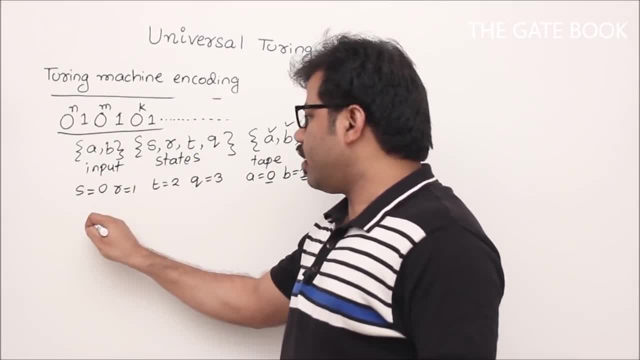 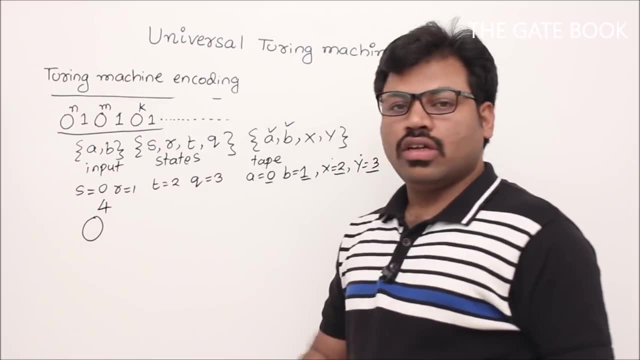 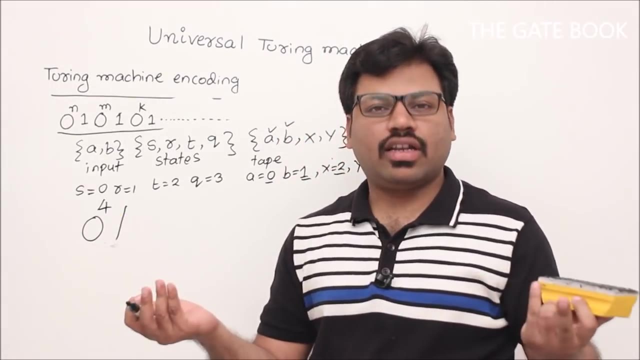 represent exactly the same thing, How you see. First I write number of states, How many states. you have 4, right. Then I write like this: 0 power 4.. So whenever someone reads this one, they understand that, oh, there are 4 states And what are they? Simple, that 4 are by default. 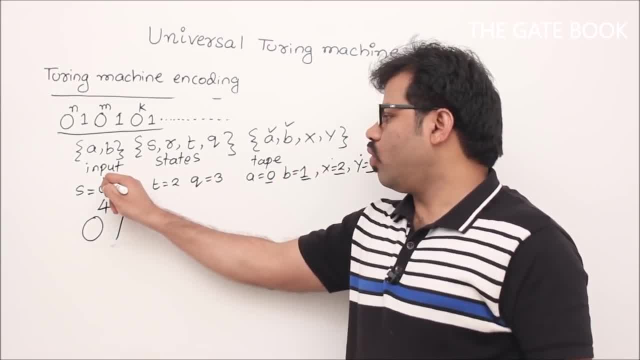 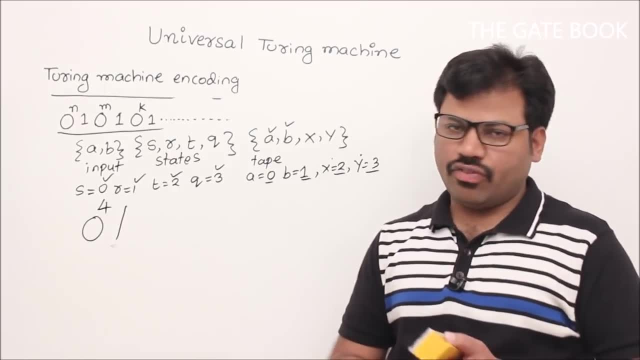 0,, 1,, 2, 3.. In my encoding you see that four states are 0,, 1,, 2, 3. Agree, In that way I can uniquely represent number of states and various state information. Now we represent tape symbols, So we have four symbols. 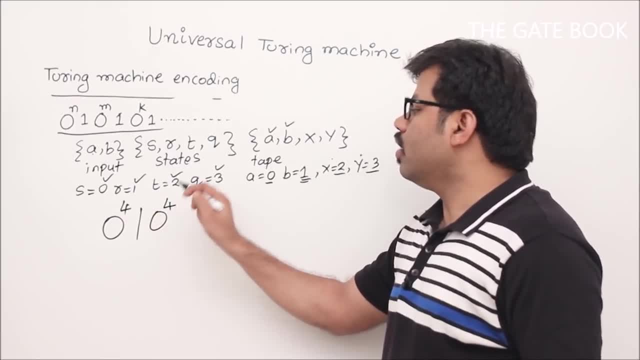 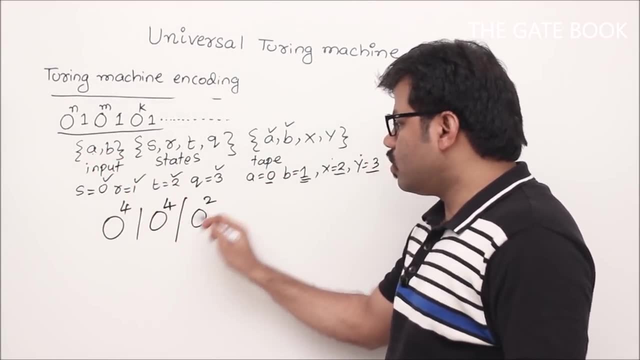 right. That is why we encode like this: 0 power 4, okay, Now out of them, how many are input symbols? Two, right, That is why we write 0 power 2 in that way. So this one is going to be working. 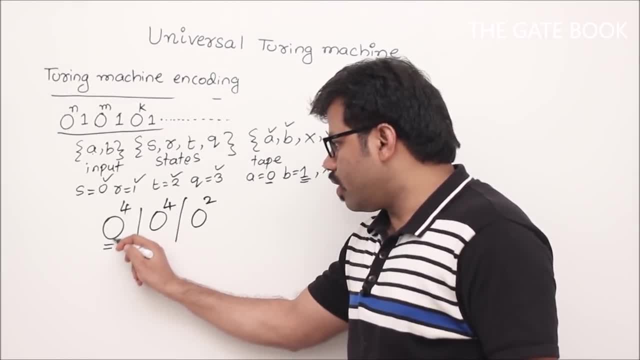 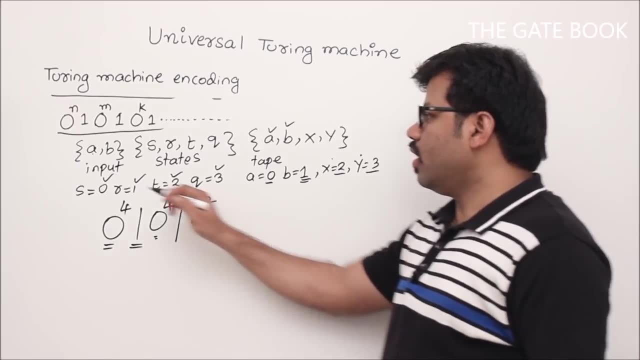 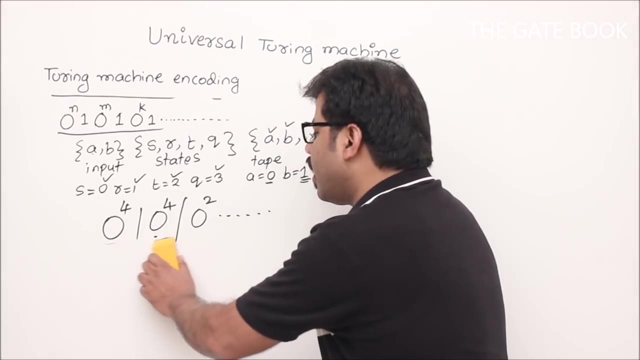 like a separation. So this number of zeros represents states. this number of zeros represents number of tape symbols. these number of zeros are going to represent your input, number of inputs, correct Now in that way, remaining stuff. So when you encode like this, everyone can understand. 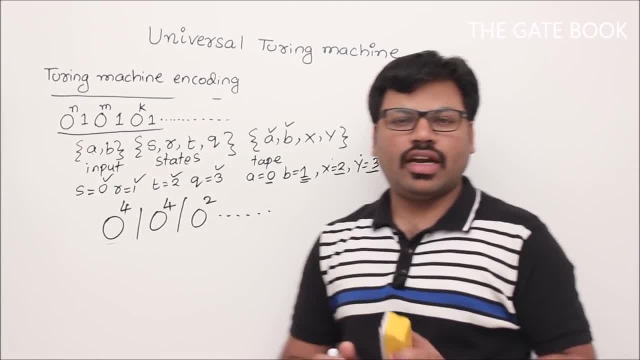 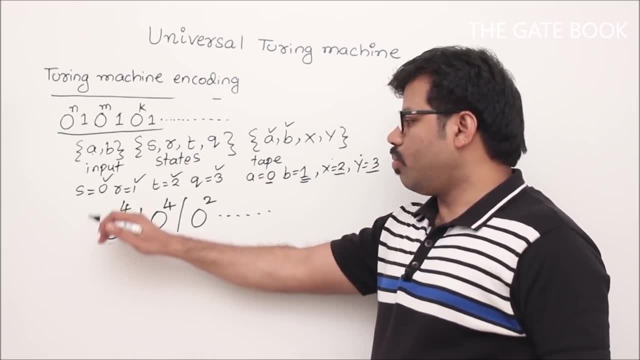 in a unique way. correct. If you fix the rules and if we have a common agreement, whatever the way I write in the same way, if you encode, then easily we can understand that. let us say 0 power 4, 4 is nothing but. 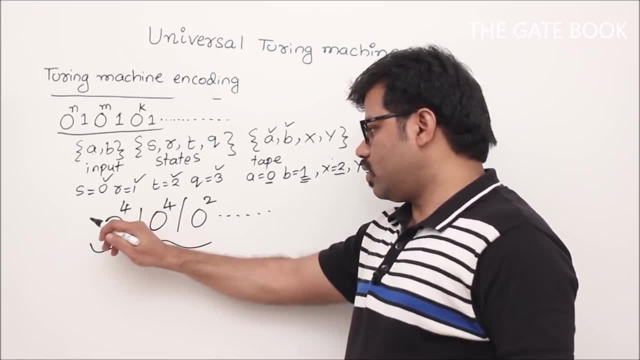 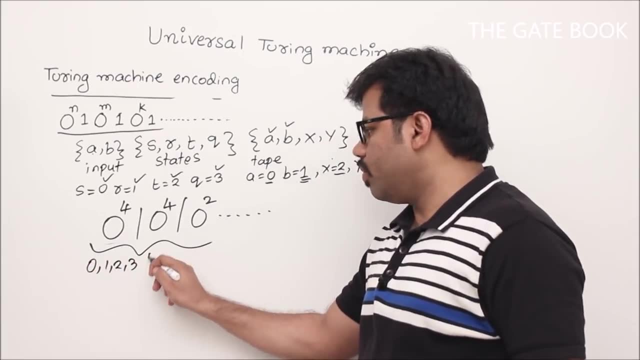 See now how I decode it. I will tell you: 4, first zeros represents number of states. 4. What are they? Automatically, they should be 0,, 1,, 2,, 3. Such a way I encoded them. 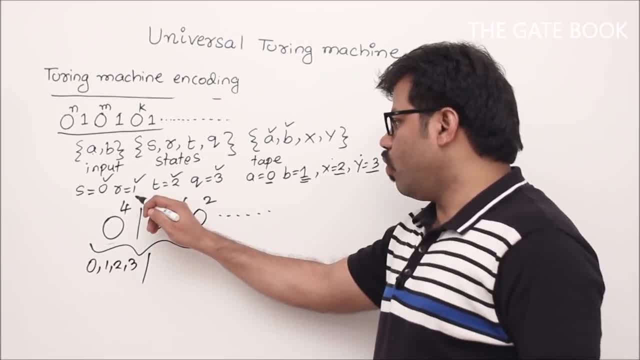 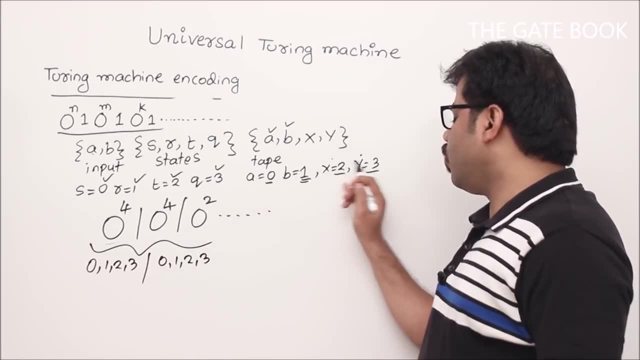 Next 0, power 4 indicates in tape symbols. We have four tape symbols. What are they? 0,, 1,, 2, 3, okay, See, that is why I gave a0, b1, x2, y3.. Now, next 0, power 2,. that means this represents: 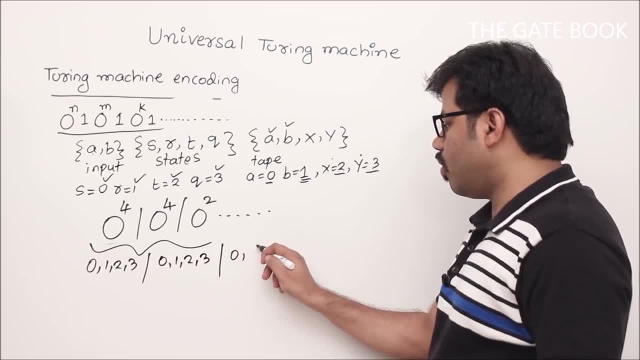 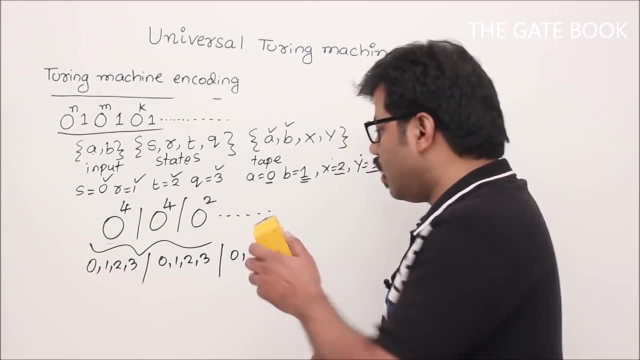 number of input symbols: 2. What are they? 0,, 1. Yes or no? We check it out. a0,, b1.. In that way we can uniquely encode it. That means Turing machine can be encoded. Now one more thing is how to represent otherwise, how to encode the transition. 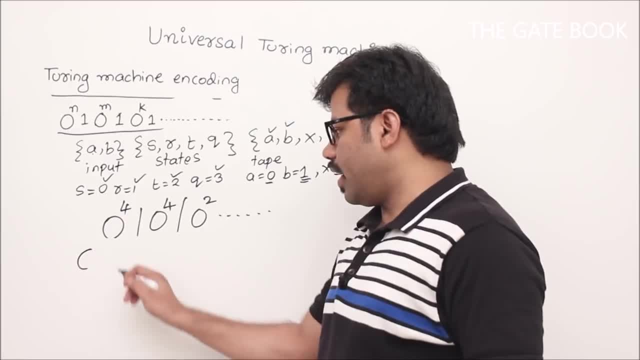 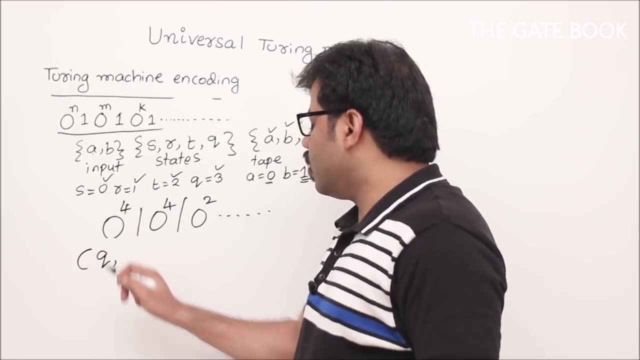 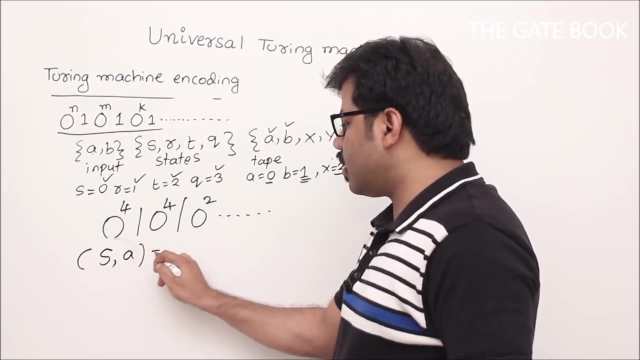 function. That is the final thing. right Example: you have a description like this transition function. Let me take one state: q, okay, q on something. otherwise I take start state. Start state on seeing input: a. Generally we write like this: right s on a. 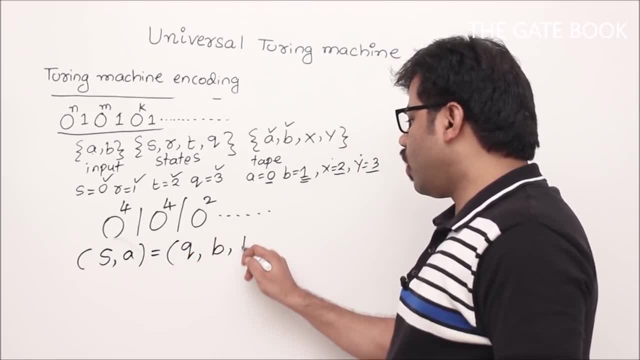 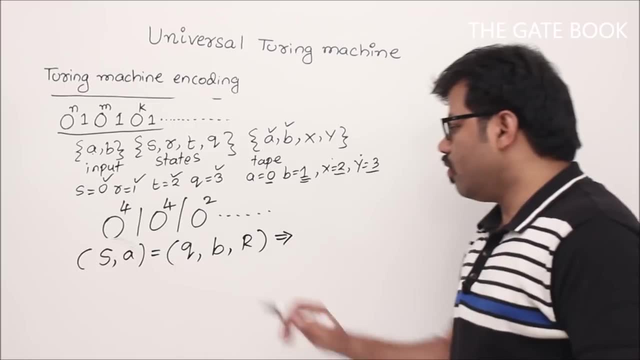 go to q and make it b and go to right side. How to encode it For that? what I do is I am going to use 0s and 1s and I am going to do the same thing. First of all, blindly write like this: 0 power s. 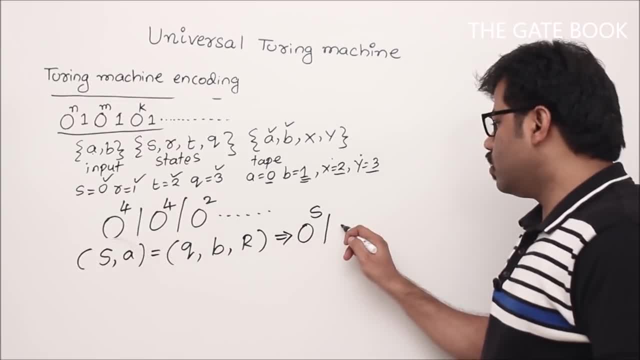 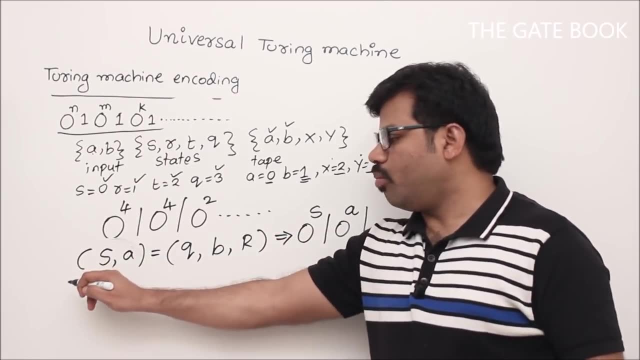 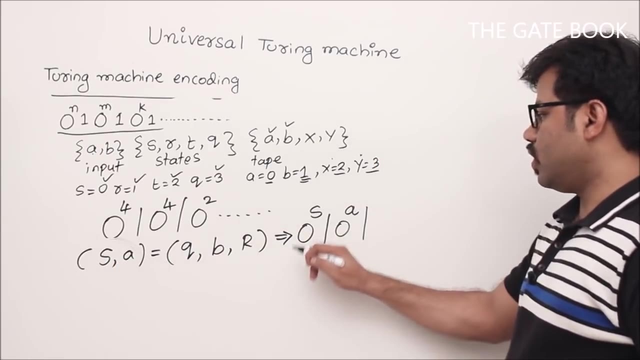 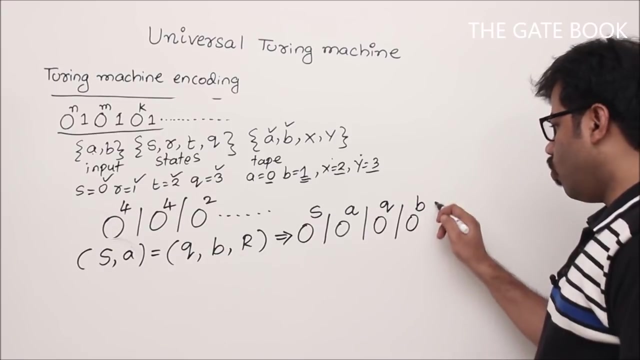 stop a, 0 power a, stop q, b r. We know that any transition function will have five components right: s a, b n, State symbol, state symbol direction. That is why 0 power s, 1, 0 power a, 0 power q. 1, 0 power b, 1, 0 power r. okay, So let me use: 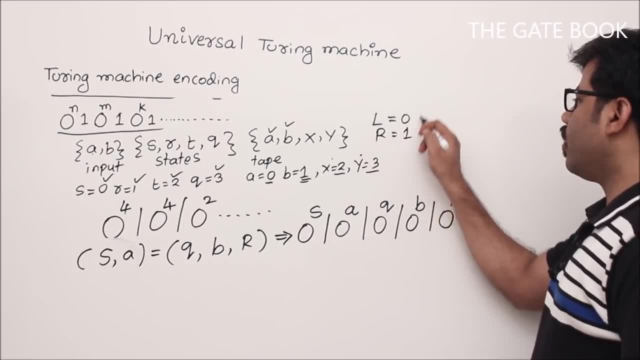 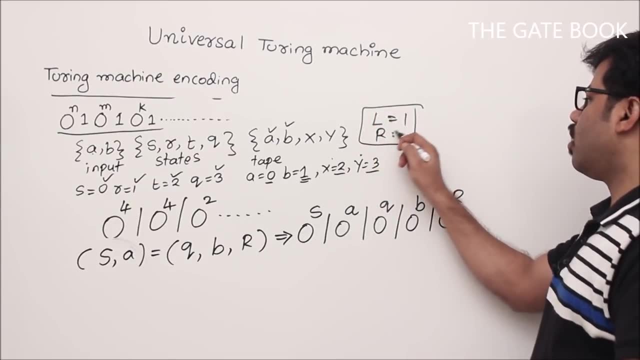 l means 0, r means 1.. This is the encoding for directions. okay, Let us do that. Otherwise I use: l means 1, r means 2.. Anything we can use, not a problem. Now you see. 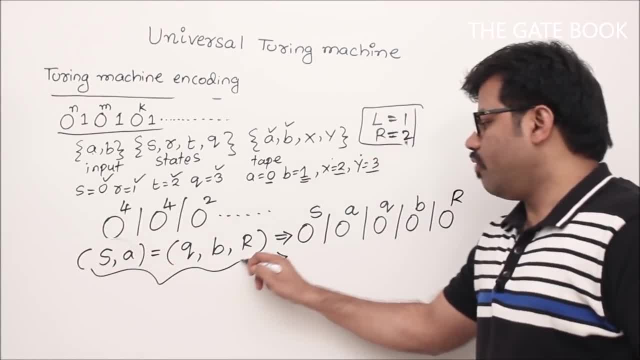 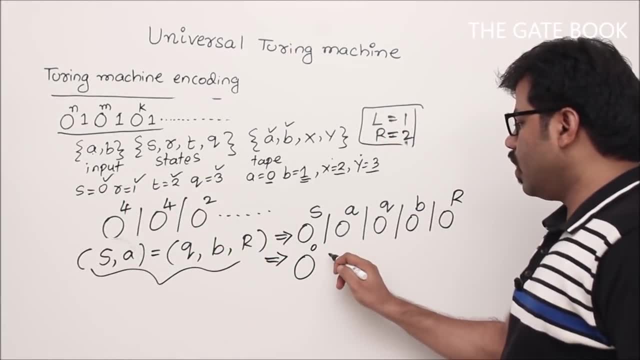 how we are going to encode this kind of descriptions. we will see. You have a description: right 0 power s s is what? 0, right 0, power 0,. okay, Now 1.. Next. 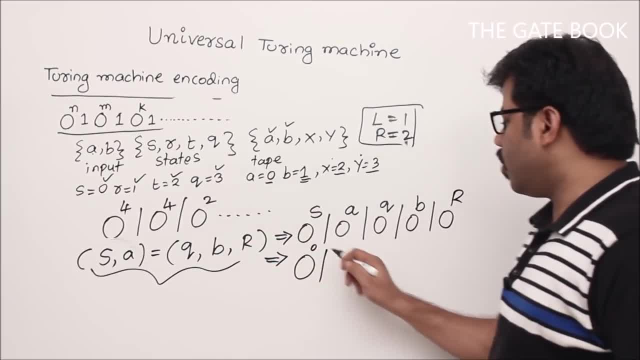 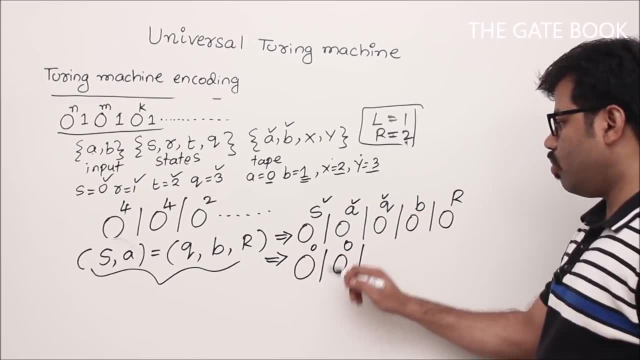 0 power a. What is a here? See, a is nothing but for us, 0 power 0.. This is for your convenience, But finally, end of the day, this will be converted like this: 0 power 0,. 1, 0 power 0,. 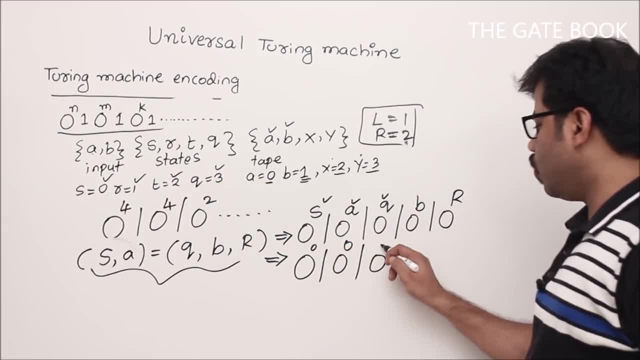 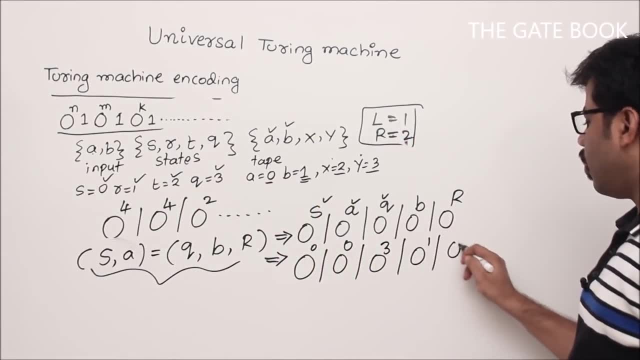 1, 0 power q. q means what? 3, 0 cube. 1, 0 power b. b means what See? 1, 1, 0 power r. r means 2, 0 square. In that way, I am going to encode all your description. 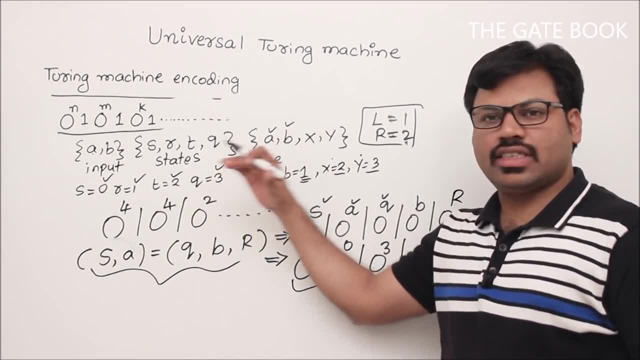 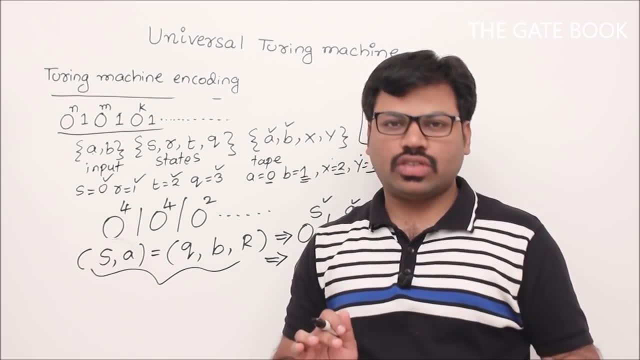 otherwise transition function. Finally, all your Turing machine description is converted to encoding binary format. So you realize that a Turing machine can be converted to 0s and 1s. Once you convert the Turing machine into 0s and 1s, if you properly, if you know the 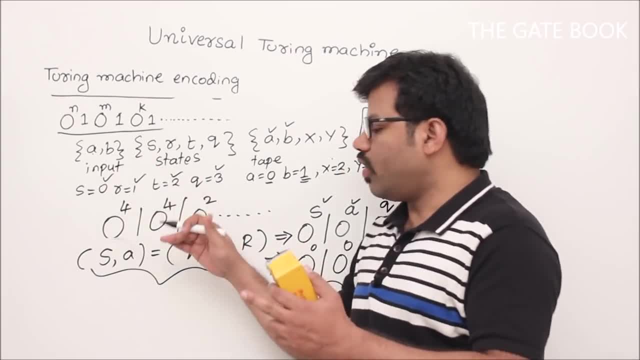 alignment. that means, if you know how this conversion, otherwise how this encoding happened, then exactly the same. So you can convert it to 0s and 1s. So you can convert it to 0s and 1s. 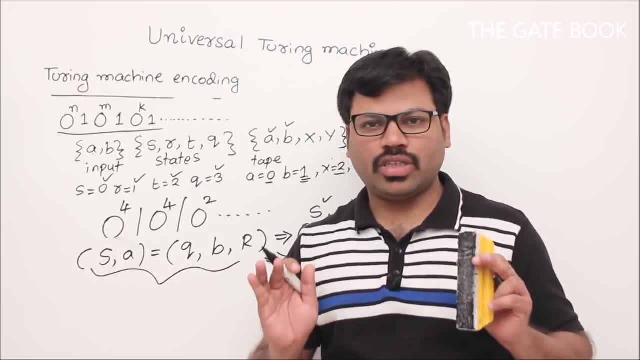 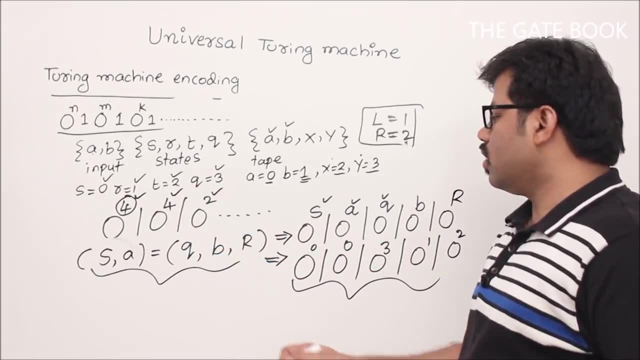 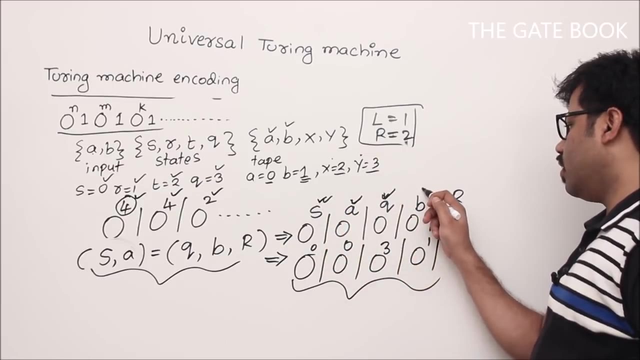 Same way, if you decode it, we can understand the functionality of the Turing machine. Agree, Now, if you see, by reading this one I understood that there are 4 states, 4 tape symbols and 2 input symbols. And by understanding, by seeing this one, 0 power sc s on a will go to q and 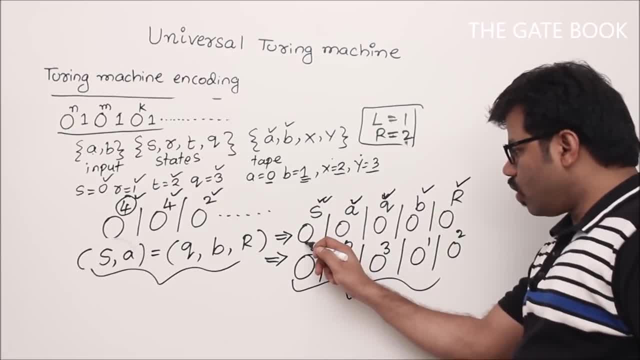 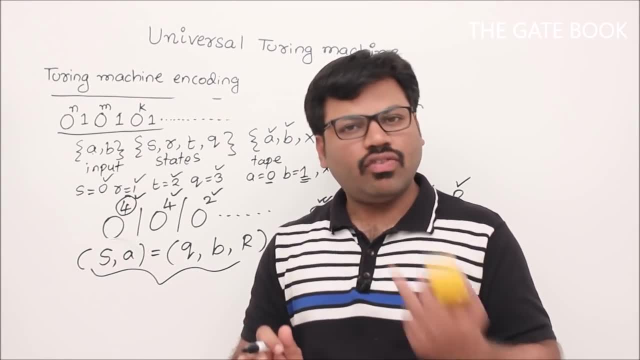 symbol modification is b and it will go to right Here also. I can understand the same with binary encoding also. Finally, we are not disturbing the meaning of the Turing machine and we are converting that Turing machine into 0s and 1s. So we are converting that Turing machine into 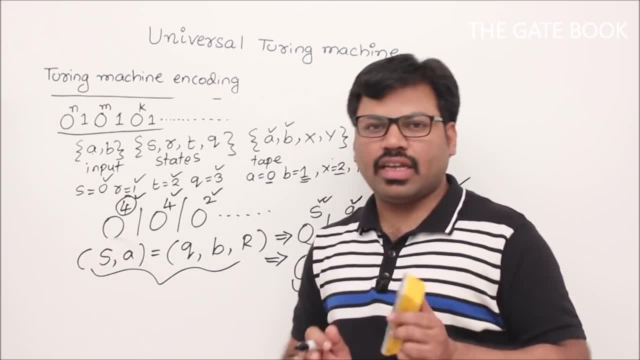 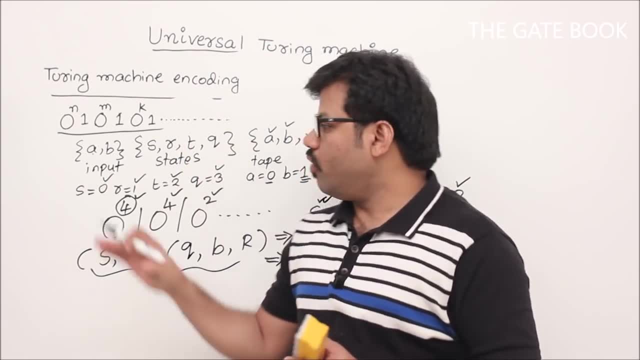 binary format. So once we have a binary format, then we are going to learn universal Turing machine. Okay, So let us try to understand universal Turing machine with this terminology, with Turing machine encodings- From now onwards, everyone who is watching my videos. 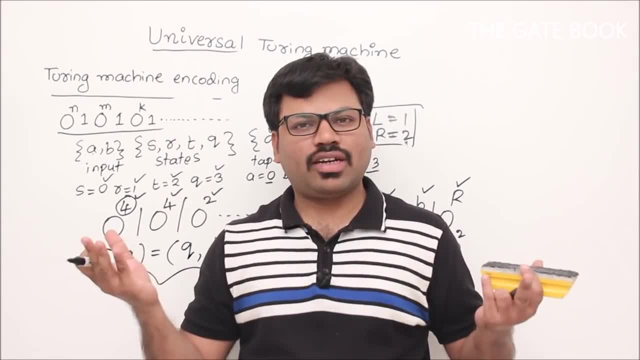 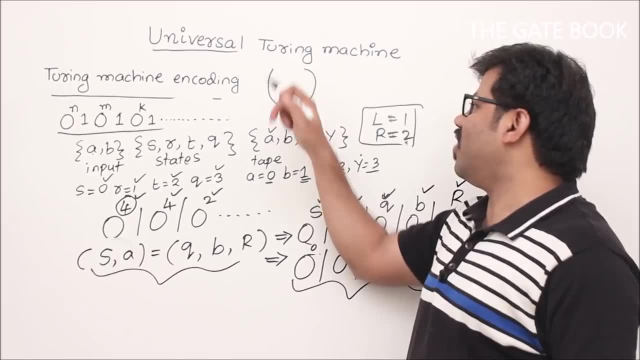 imagine that every Turing machine is nothing but a binary format, Correct 0s and 1s. Now, all collection of Turing machines is nothing but a language. Wonderful, isn't it? So every Turing machine is nothing but a language. Wonderful, isn't it? So every Turing machine. 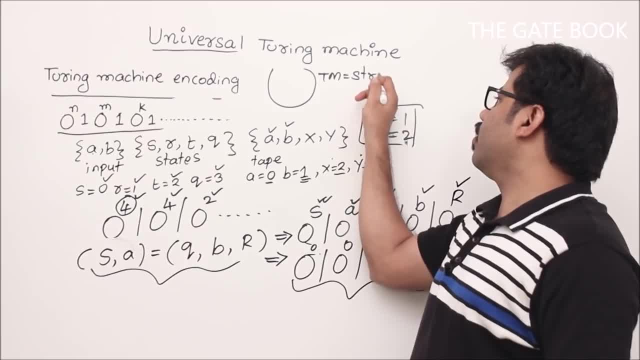 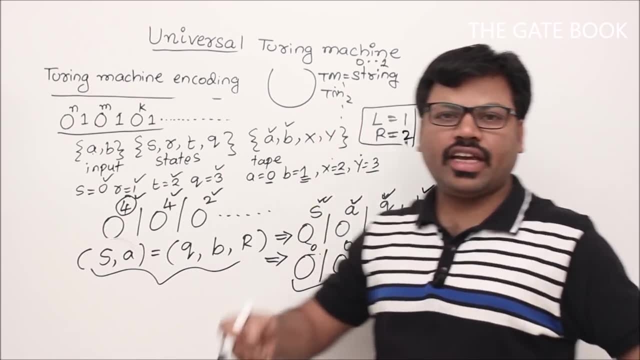 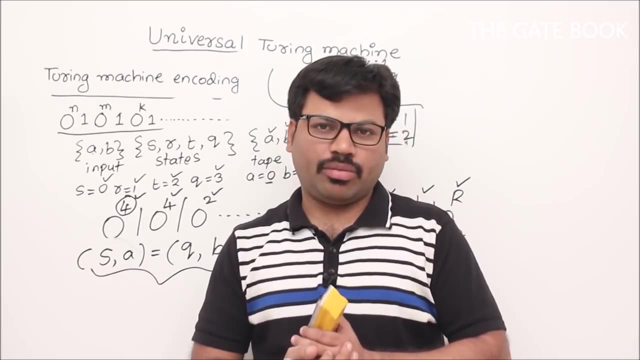 is nothing but what A string. Remember it: Turing machine is a string with 0s and 1s from now onwards. So all possible Turing machines in the world. if I take into a bag, that bag is nothing but collection of strings, Correct? So in that way we can understand about collection of Turing. 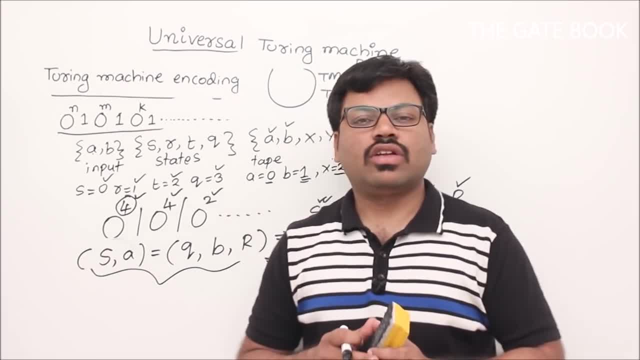 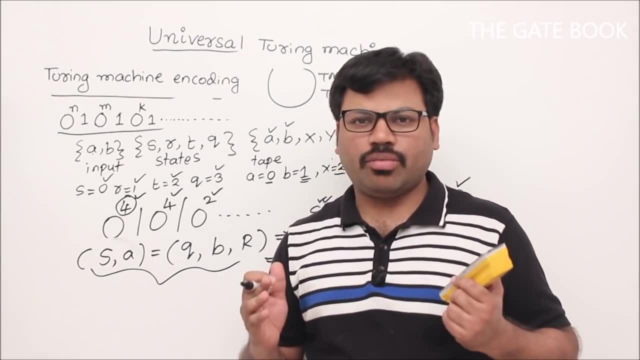 machines. Okay, That forms a language, Remember it. So now we will go to universal Turing machine. Sir, what is universal Turing machine? I am going to explain. That is one of the Turing machine. What is the functionality? The functionality of Turing machine we will see. So it is like a compiler kind of thing. Okay, 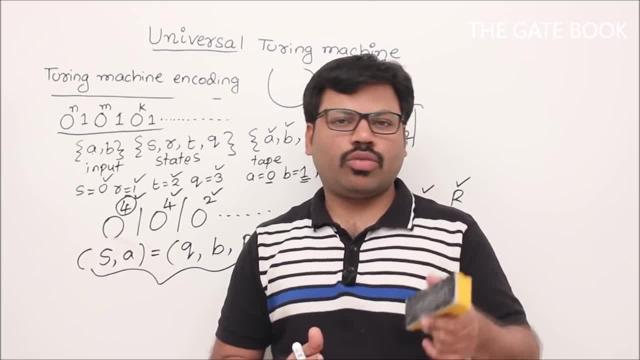 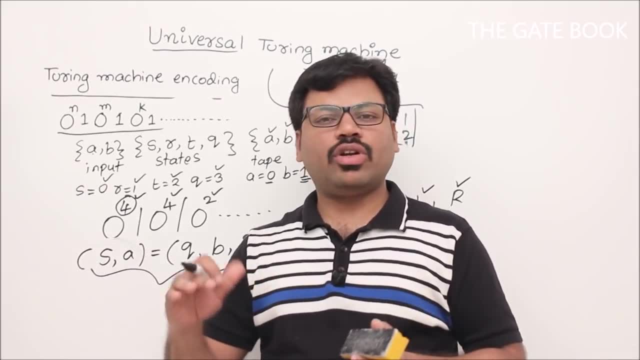 Generally your compiler, otherwise interpreter, does what. They take your program and they simulate it Right. That means they understand your program and exactly so they convert that program into another program. Of course that is a job of compiler or an interpreter In the same. 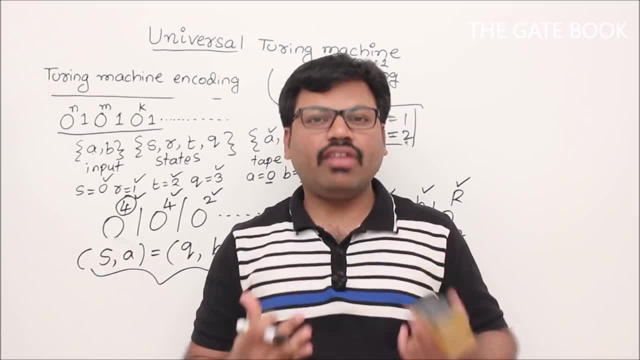 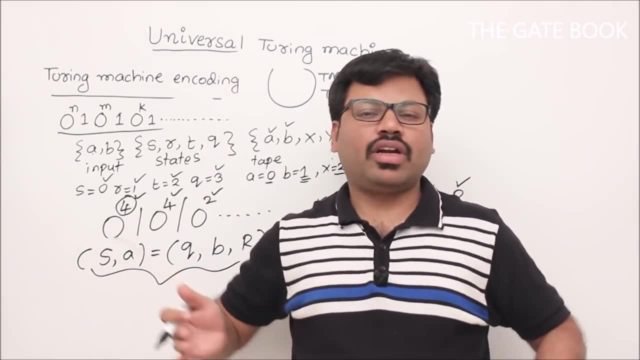 way this universal Turing machine is going to behave, like you know, exactly like any of the Turing machine. We will see the details At this moment within one line. I cannot tell that, But I will give complete description of your universal Turing machine and its functionality After that. 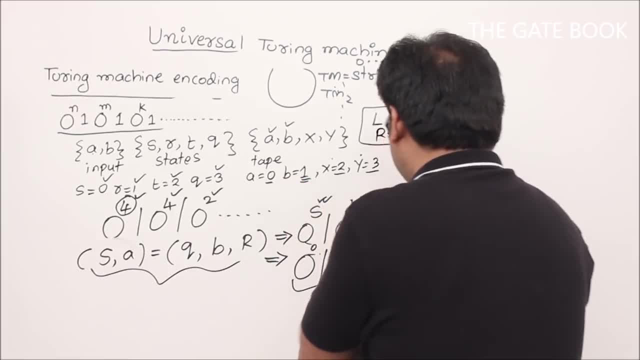 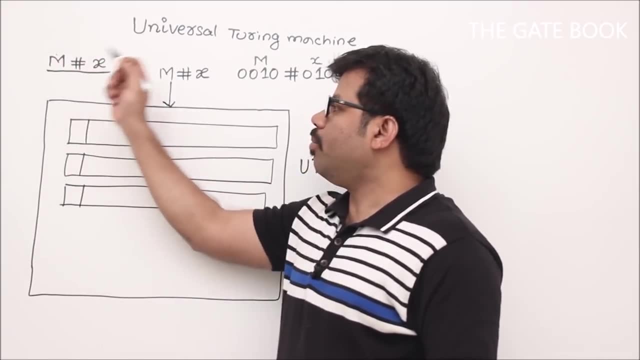 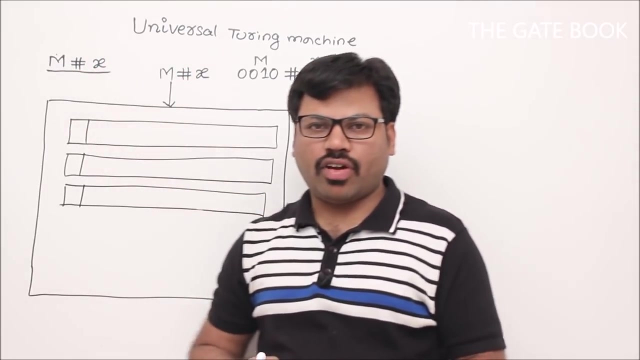 you can understand it. Let me begin with universal Turing machine. Let us see this Turing machine. So first of all, I take some pattern: m, hash, x. What is that, sir? m is nothing but a binary format. Okay, What is hash? Hash is a just symbol which separates m and x. What is x, sir x is a binary format, Can? 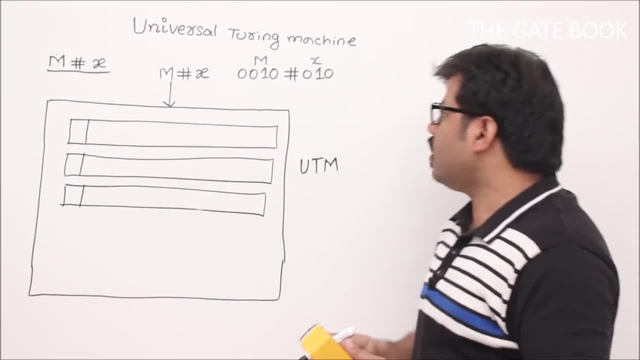 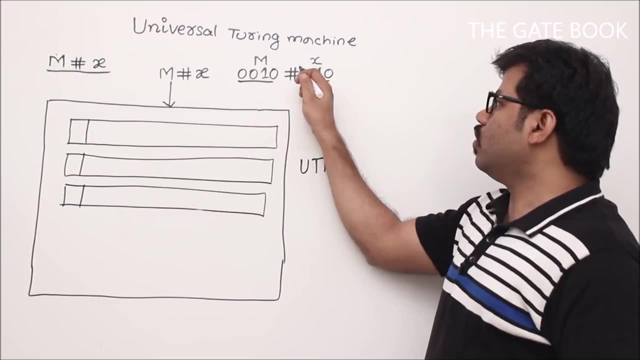 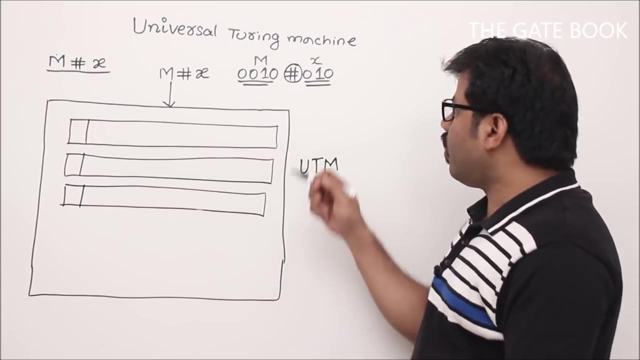 you explain us very clearly. what does it mean? m hash x. m hash x is nothing but this kind of you know binary formats: 0010, hash 010.. Hash is just used to separate one binary pattern with from another binary pattern. Sir, why are you doing that? So here, what we are going to assume is this: first, 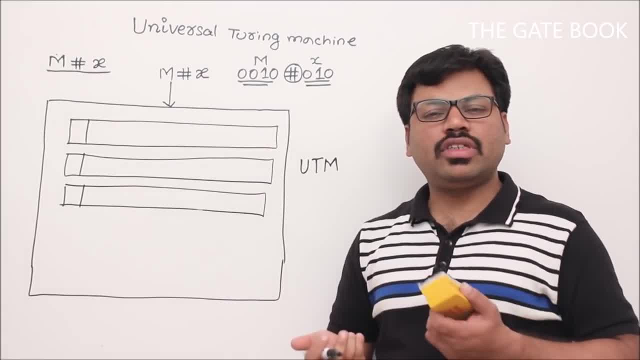 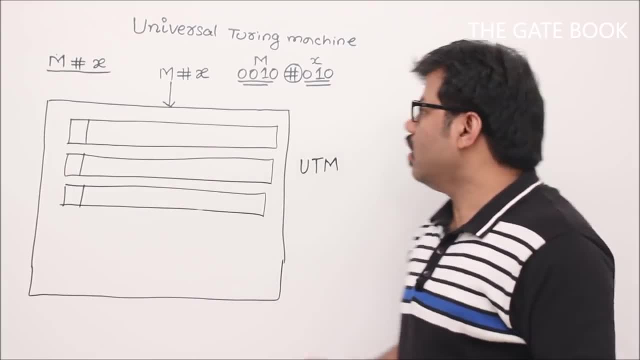 pattern is representing one Turing machine code. Sir, how Turing machine can be represented as binary format, Don't ask me, Because already I taught you how to encode a Turing machine into binary format. Assume that, for simplicity, this is one of the binary format of a Turing machine. 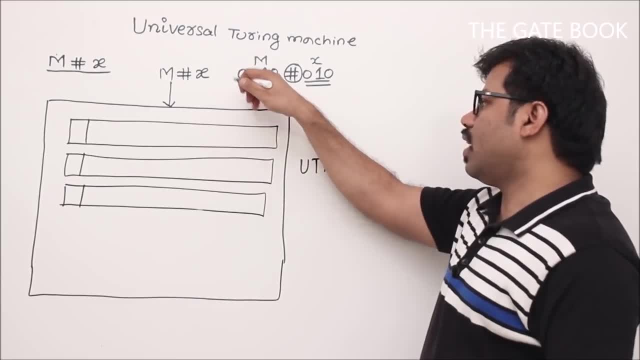 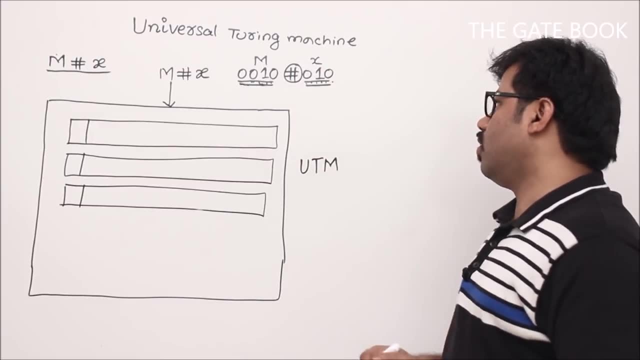 That means otherwise. it is a binary format of a Turing machine. That means otherwise. it is a Turing machine code in a binary format. one of the encoding- 010, is one of the input which we can give for a Turing machine. such an input it is- We know that Turing machine. 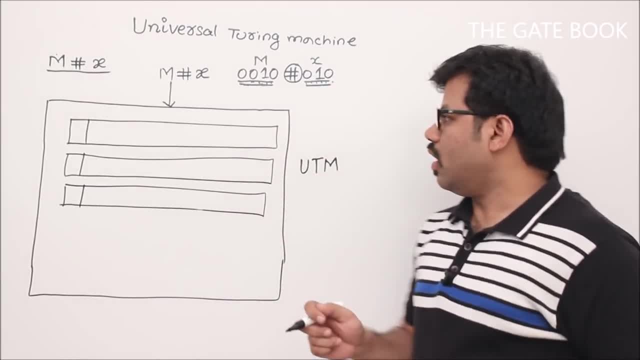 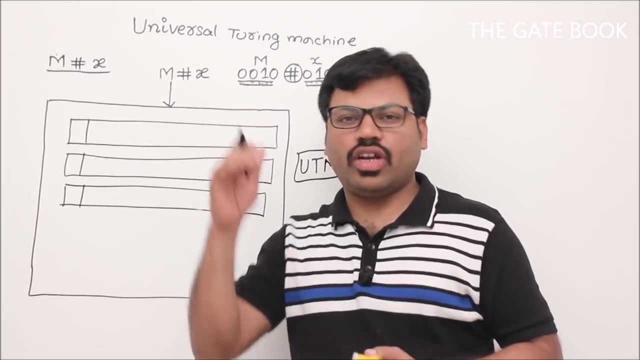 takes input right. So 010 is one of such an input. Now I am going to design a universal Turing machine. It is a very big Turing machine. That's why I can't give a code for it. Example: if you ask me, sir, please explain us operating system code. How can I explain In five minutes? 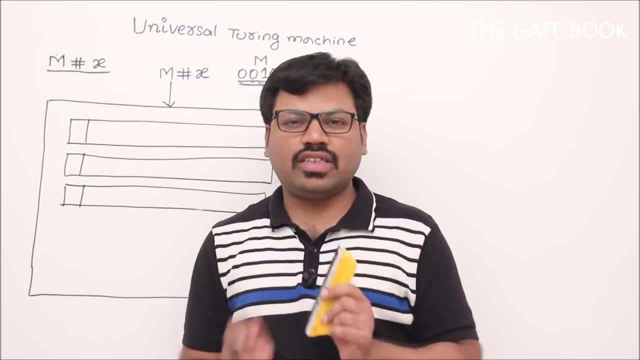 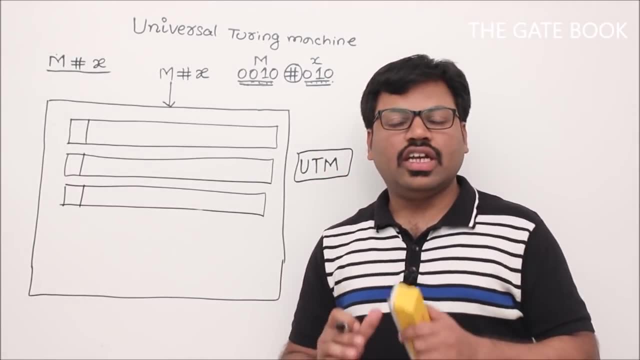 we generally discuss about functionalities of operating system and just ideas of operating system. right in the same way, here also i am going to teach you functionality of universal turing machine. it is very big turing machine, so that its code is very complex, rather than that we understand. 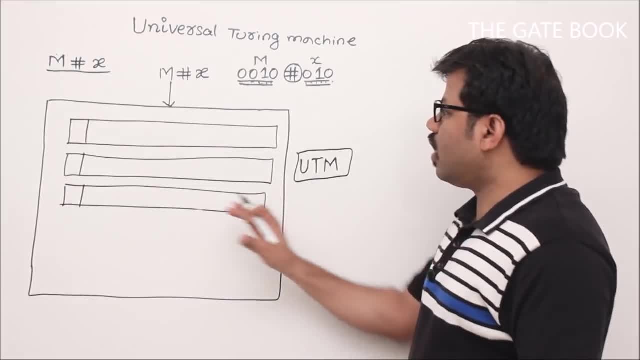 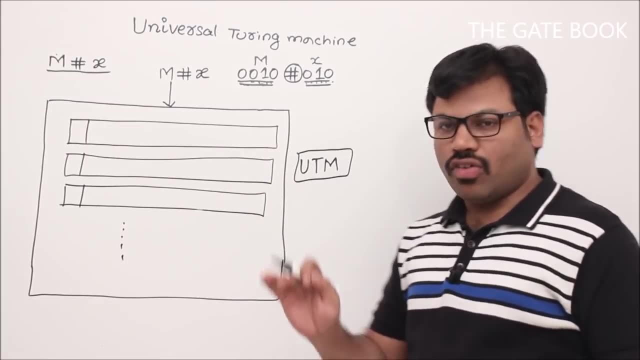 what? what that code will do. okay, now we will see. assume that, let's say, universal turing machine is having some code. because of that code it is going to do some functionality. what is that? i will tell you. for that universal turing machine, we are going to give input in this kind of format: 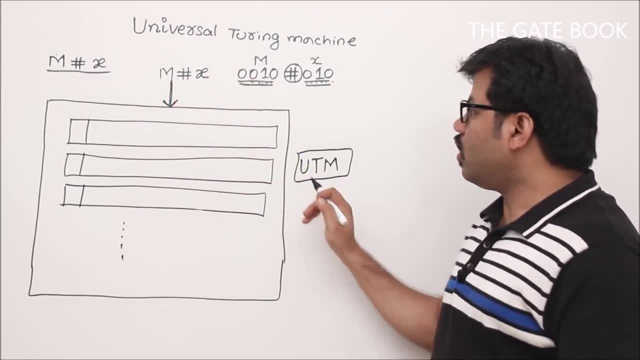 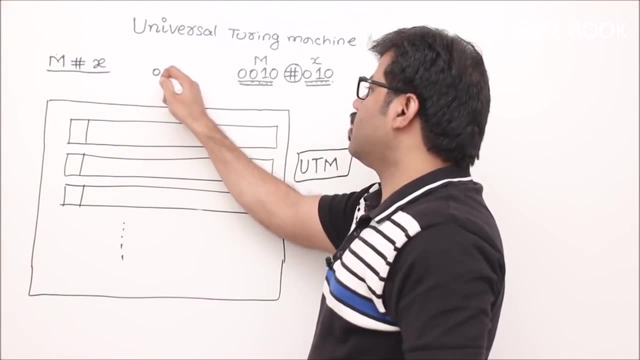 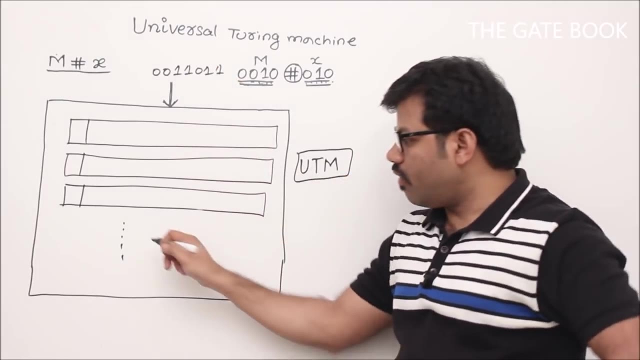 okay, what is that? m hash x universal turing machine accepts only this kind of code. sir, what if i give a different code? how you give like this, sir: zero one, zero, one, one, followed by zero, triple one. i don't give hash. so your universal turing machine is having a code, such a method, it will do one. 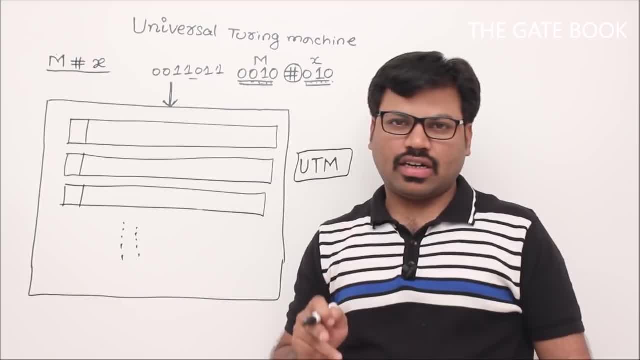 scan and it can find out whether there is a hash in between that or not. if there is a length in between, it can do: aah is the question. is that what? how does it reveal the problem? so these travails explain during the skill roll. is no hash in your input, it will simply reject it. okay, that means your universal turing machine is. 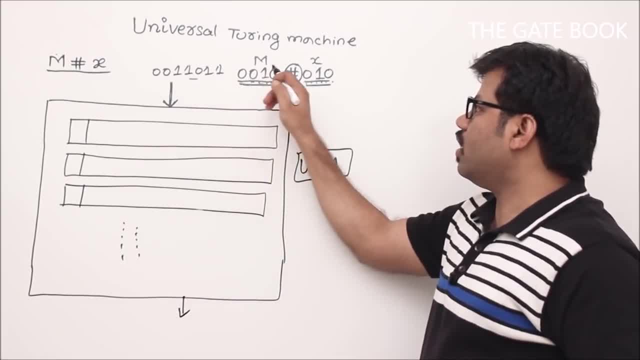 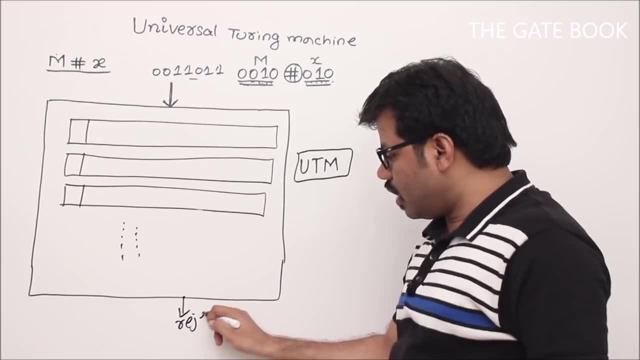 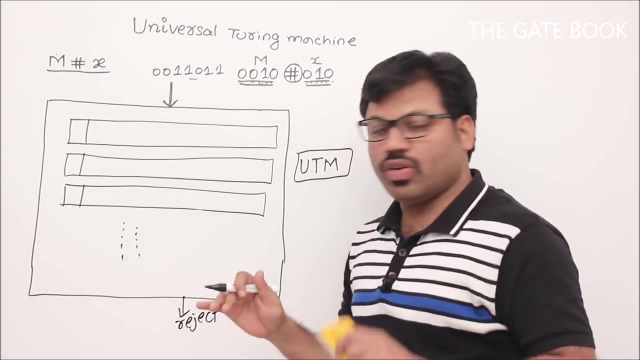 going to reject inputs in the form which are not in the form of m- hash x. okay, binary format, hash x. so that will be rejected, don't worry about it. that is one of the functionality of your universal turing machine. already i told you one thing: your turing machine can be designed. that means we know. 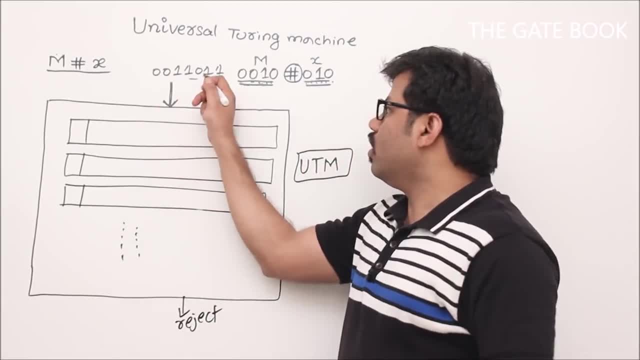 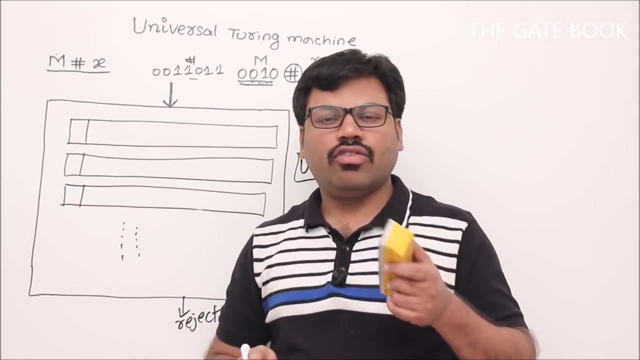 that turing machine can be designed such a way that, given input, whether that input contains hash or not, it can check it out correct. did you remember what were the functionalities you have seen for any turing machine? we have seen a turing machine which accepts a power n, b power n which. 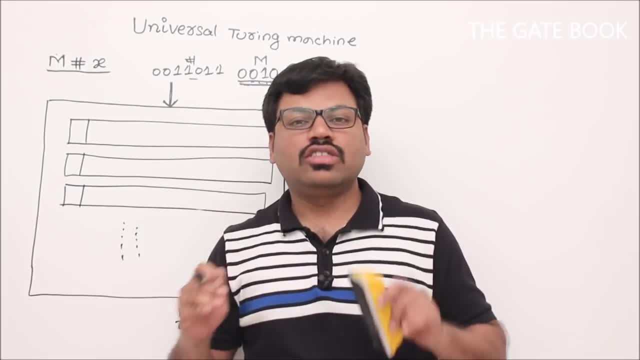 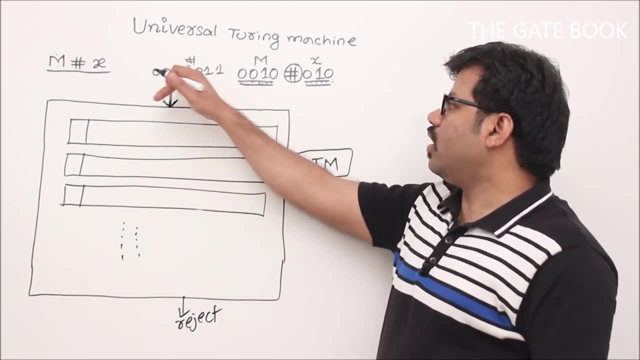 acts, which can copy the input from one place to another place. similarly, your turing machine can do lot more things. okay, remember it. similarly, one of the thing your turing machine can do is whether your input has hash or not. that's quite easy. so there will be a state. so i'm just telling. 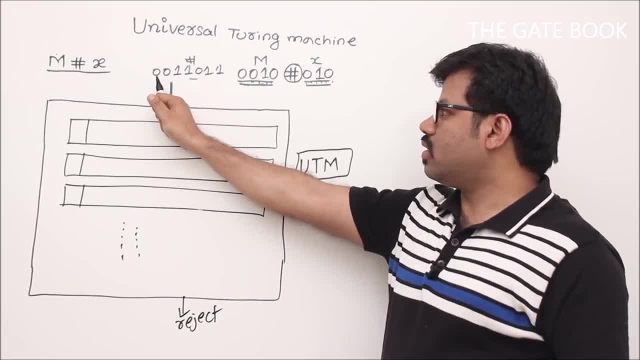 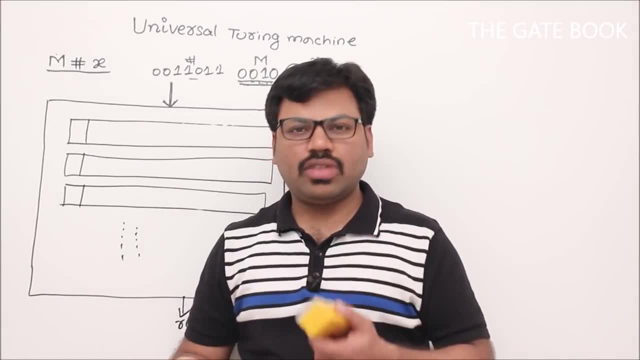 the functionality. how to do that? simply take every symbol. if it is not hash, go right. not hash, go right. in that way, if you don't see any hash, go to reject state. in that way easily we can develop that functionality. so universal turing machine is going to have very 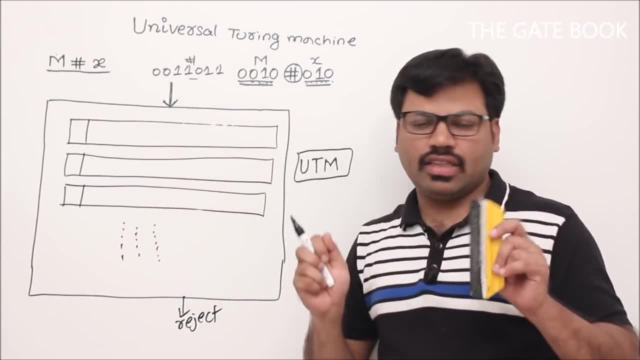 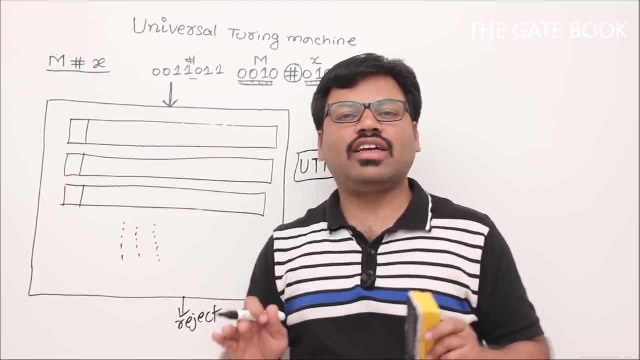 complex code first. it will check for hash. you should agree that things okay. so at this moment, whoever is watching my video, don't try to write a code for universal turing machine. it's like writing a operating system code while attending the os lecture. is it possible? no, right, it needs. 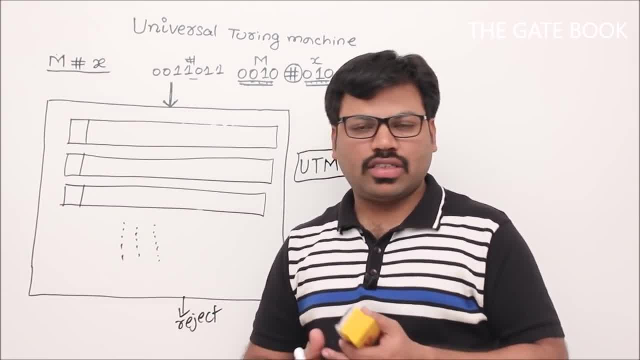 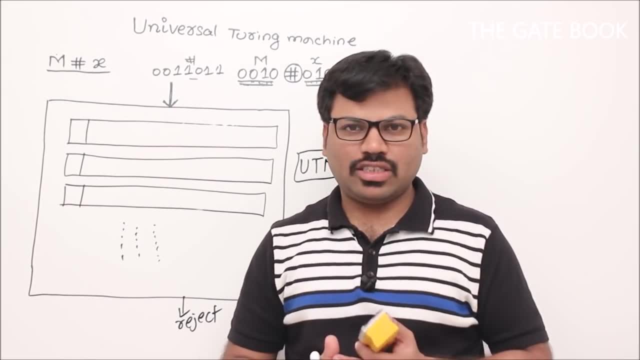 lot of patience and lot of details, but under the current system it is not possible to write a code. understanding operating system: everyone can do correct. so we can understand easily, but writing a rigorous code will be definitely difficult at this moment. similarly, understand the functionality of universal turing machine. just listen. one functionality is: first, it will check whether 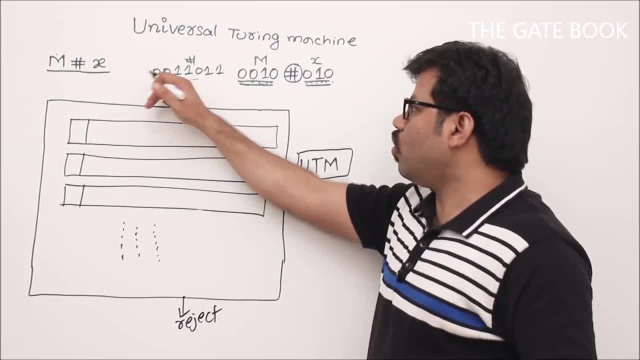 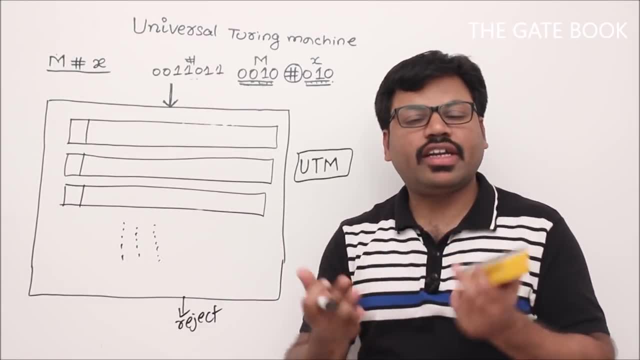 the binary pattern has hash or not. if there is no hash, then it will reject it, because i don't want that kind of inputs. okay, sir, please tell us what it accepts. i'm telling so, whatever the input, if you give right input, example, let's say a proper input, let's say a proper input, let's say a proper input. 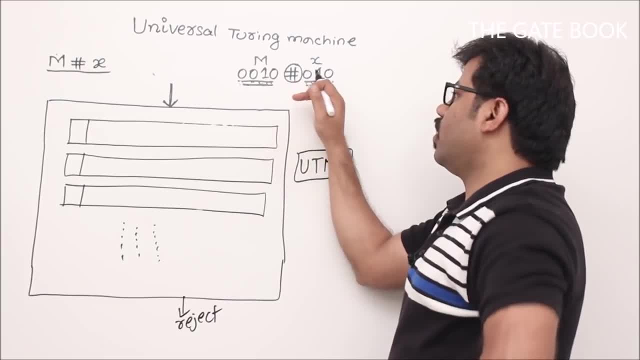 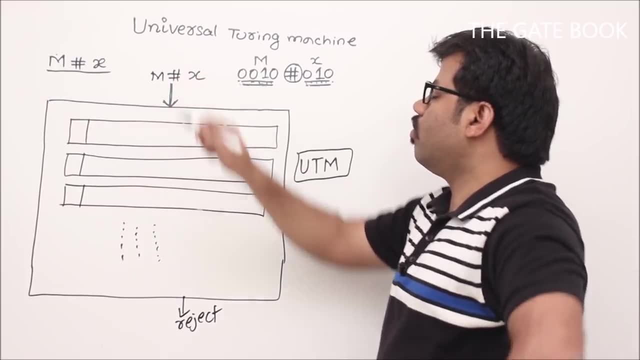 is given. okay, like 0 0, 1 0. hash 0, 1 0. rather than writing binary formats, we write like this: m, hash x. okay, now why, sir? why don't you write binary? because this binary format has a meaning. i will tell you. 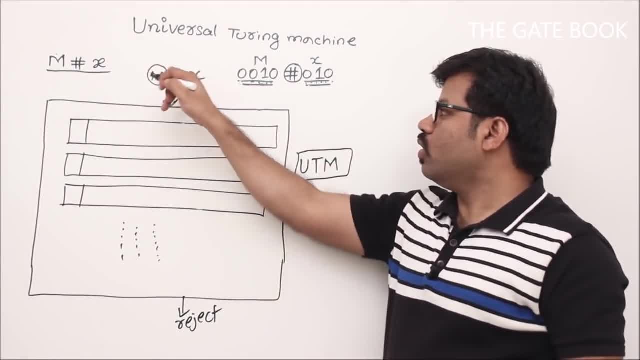 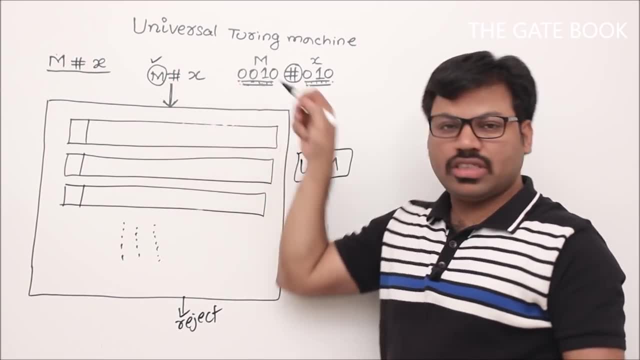 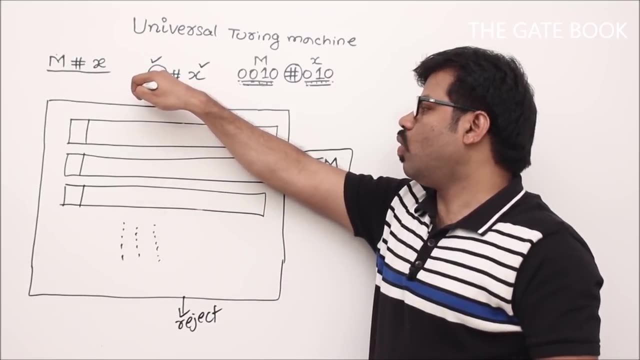 what is that? so, generally, your turing machine is going to check whether, if this first pattern is a turing machine code, really it is a turing machine code and if x is an input. so your universal turing machine is going to run this turing machine code on x. how it will do, i will tell you first of 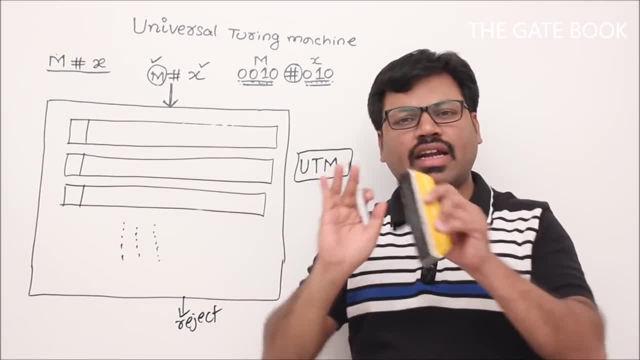 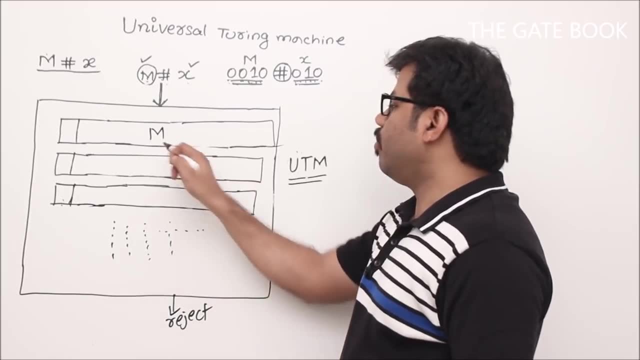 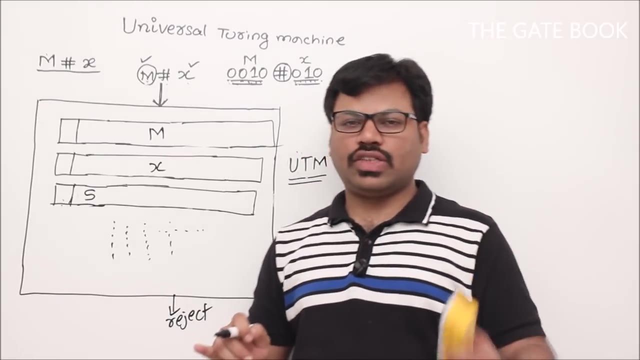 all assume that at this moment, m hash x is simple, random binary format. okay, now what happens? your universal turing machine copy m hash x here, m here, x here, and it will begin with starting state. okay, so yes, your universal turing machine will have a code such a way that input will be copied into. 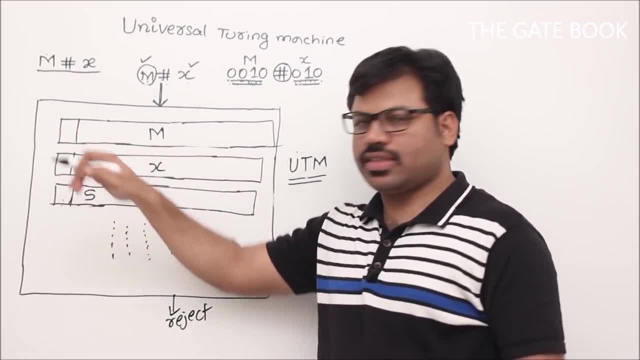 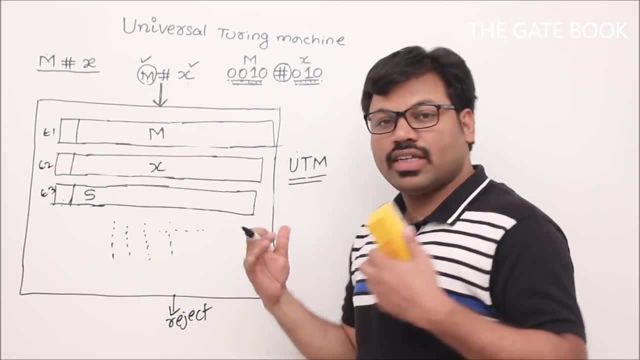 multiple tapes. okay, otherwise assume that these are all multiple tracks: track one, track two, track three. okay, for that you need a very lengthy code. i know right, but that's why understand the meaning of the code. your universal turing machine's code will be such a way. 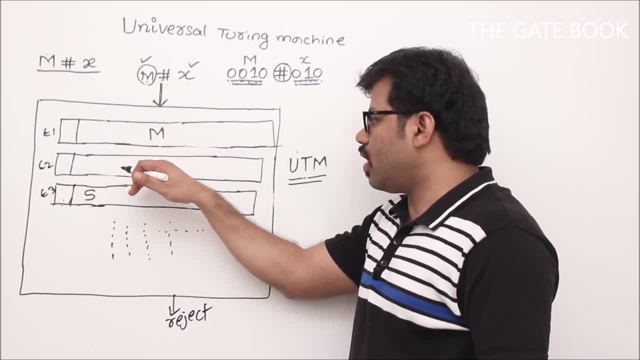 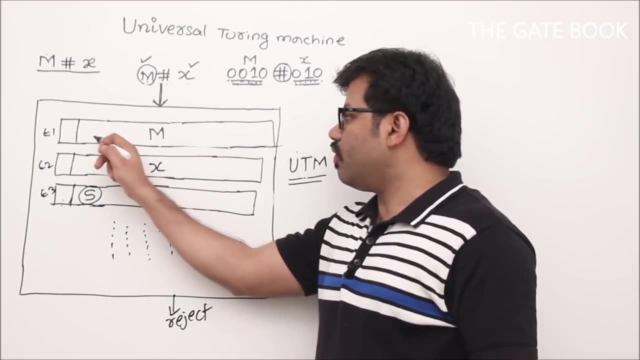 that your input will be copied here. m will be copied here, x will be copied here and it will start simulating with the starting state of your turing machine m. initially, your universal turing machine will read the code of turing machine m and because we know the code of m, we know the start. 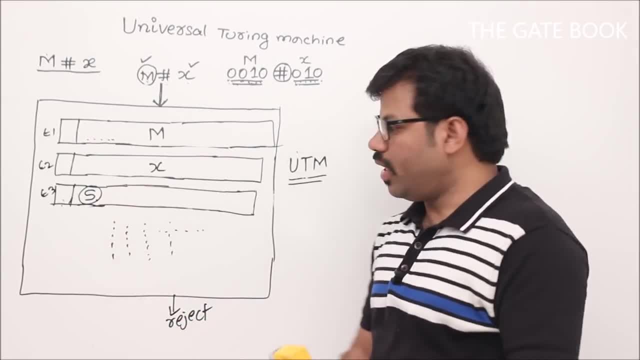 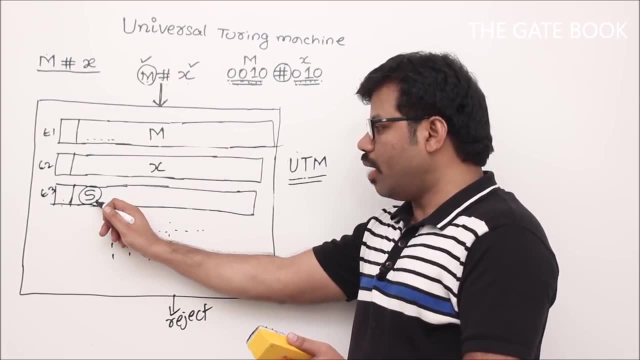 state of that one: okay, and we mark it. so we know the start state of that one. okay, and we mark it. so now, at this moment, so after some point of time, this will be the snapshot of your universal turing machine. universal turing machine is now about to simulate m on x. 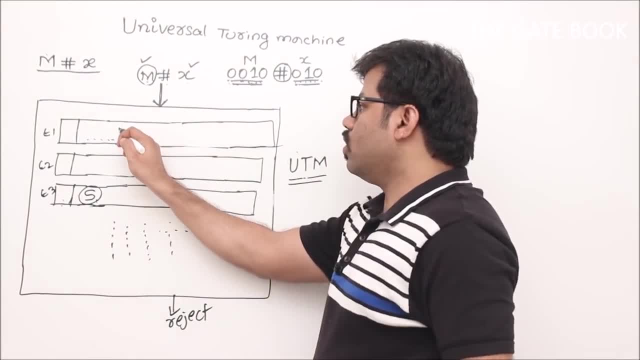 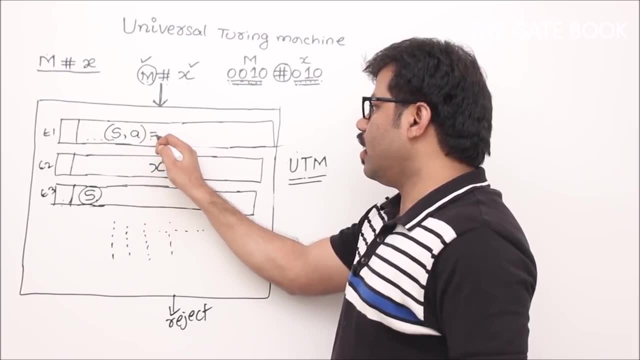 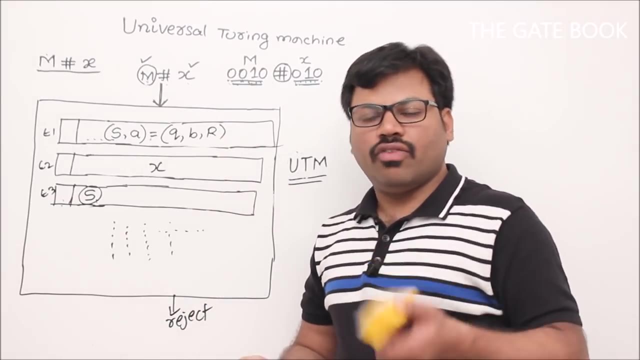 example how it simulates. i will tell you there will be definitely in your universal- i'm sorry, in your code m there will be an instruction like like this: right s and a go to q comma. b comma. right, okay, but in a binary format. assume that we know what is the structure of binary format. we know. 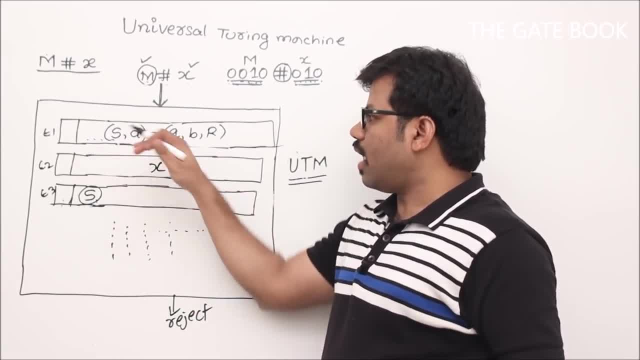 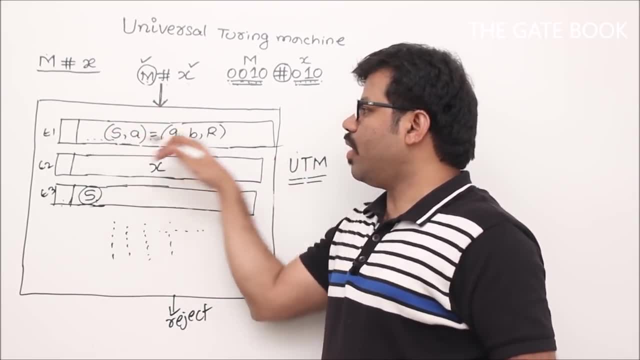 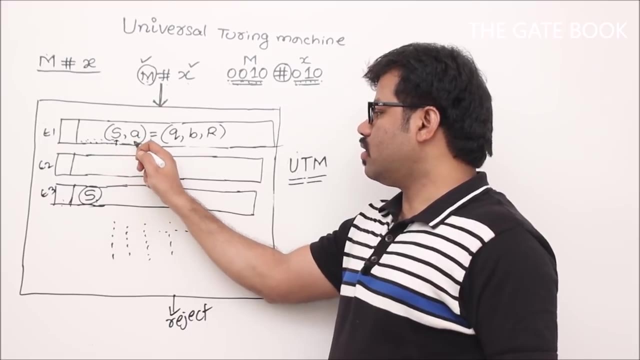 format easily. we can understand that. we can understand as a human being. you are understanding this right as a turing machine code, so this universal turing machine can understand the alignment and it can catch this point. it will read like this: so where is s yes, where is where? 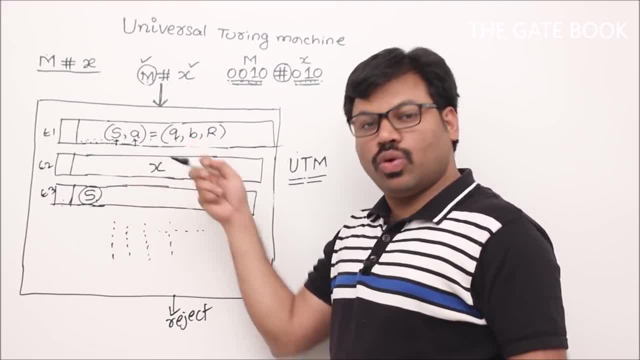 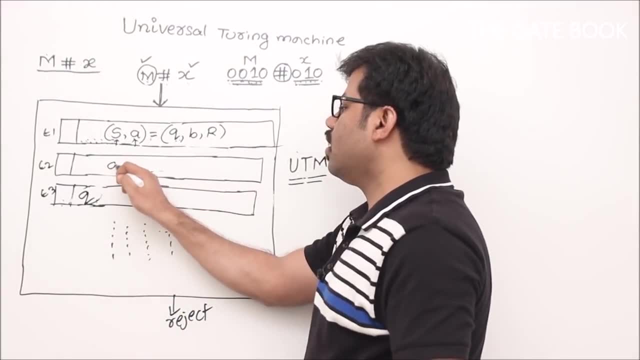 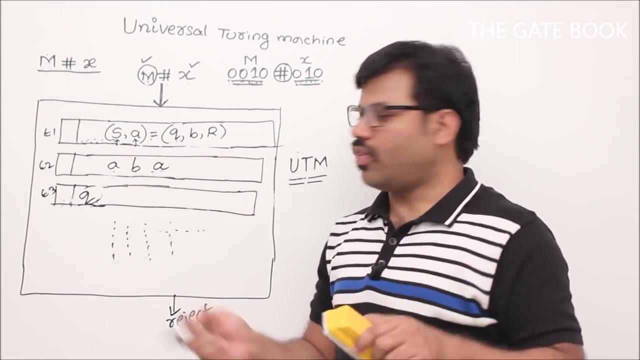 is the next symbol, a, s and a. what it is doing, q, through its code, it will understand that the next state is q. okay, now let me elaborate this: x. x is actually, let's say, aba input, though i am showing in english alphabet, but actually it is binary. don't ask me at any time, sir, why are you writing? 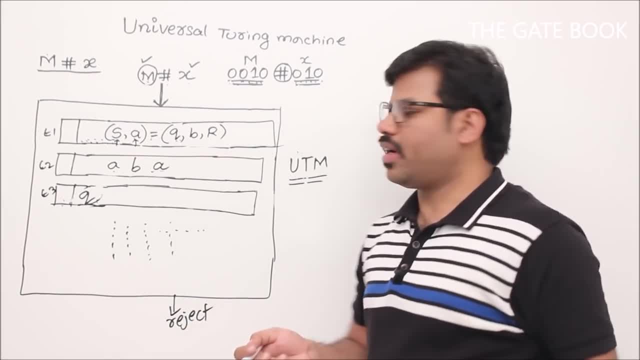 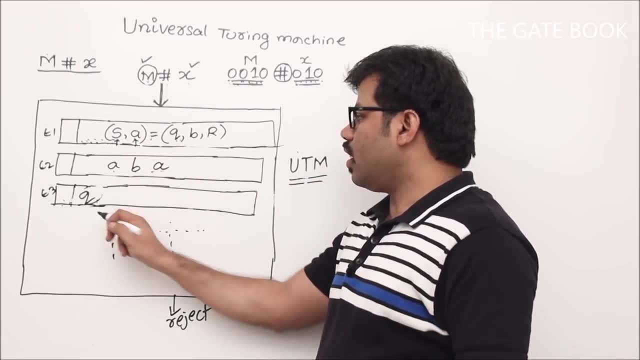 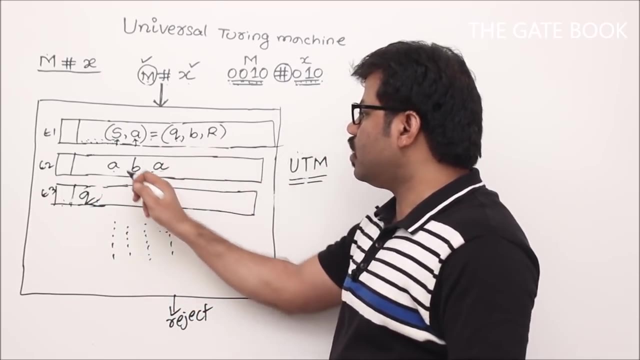 aba, it should be binary format, right? yes, let's say it's a binary format. but i'm just telling you the high level description of universal turing machine. now see s and a. it goes to q, then your universal turing machine finally remembers it. okay, then after that, what we have to do? we have to change. 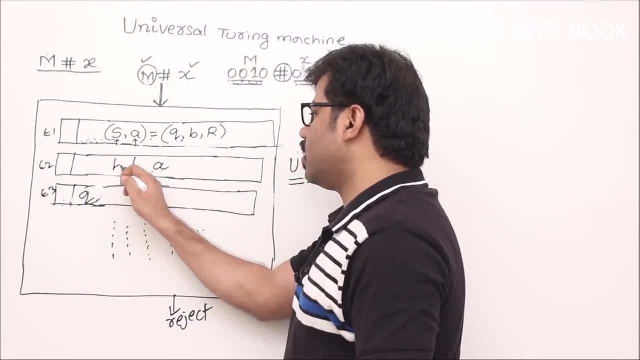 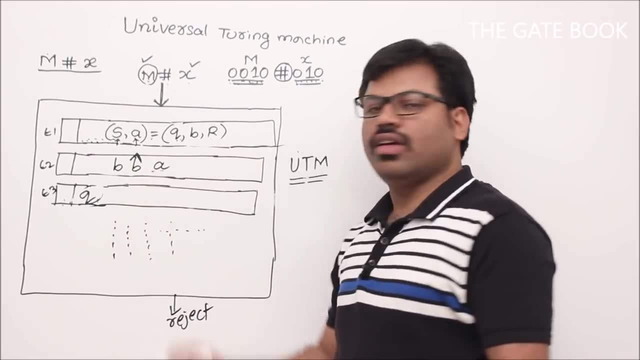 it to b, then what your turing machine will do is it will change like this: b. then after that we are going right. then your universal turing machine marks it. why? because next time we have to read this symbol: correct, we have read. we have read this symbol. next, we have to read this symbol: 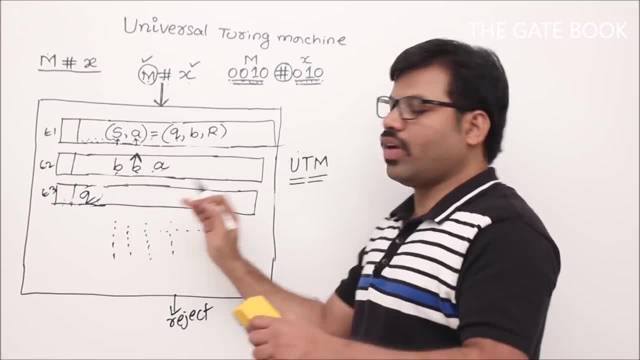 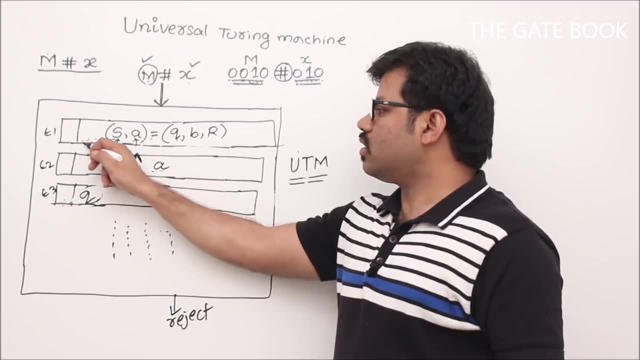 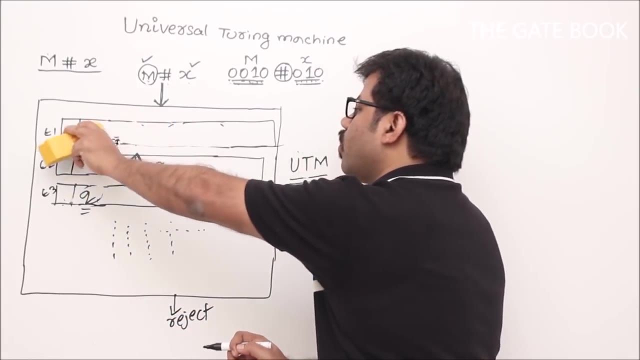 that's why it will mark it. after that it will keep quiet. then it will start simulating the next step of your turing machine m. how, sir? it will scan the turing machine code again. there we go, and it will look for a pattern q whenever there is a pattern q. okay, and whenever there is a pattern. 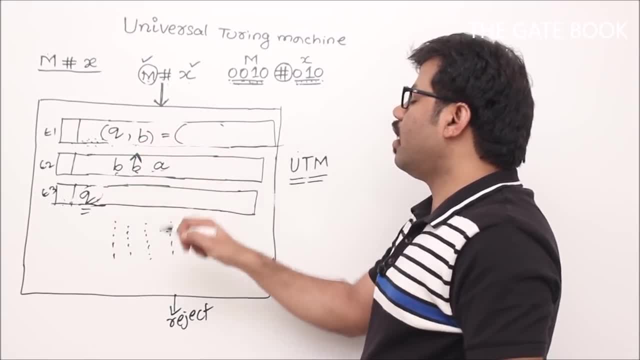 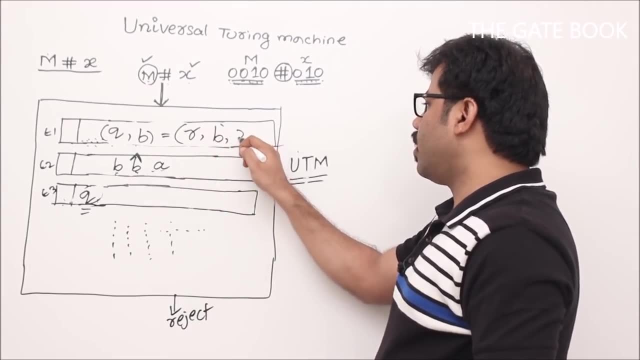 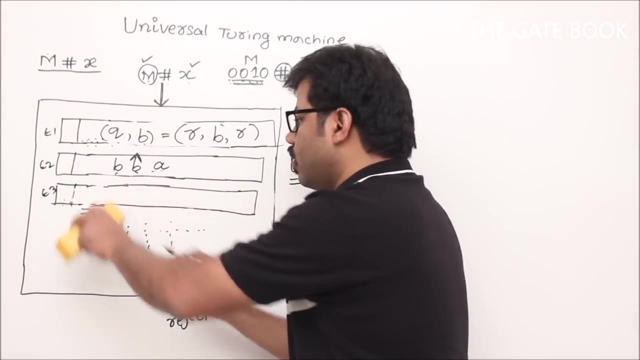 like b, then it will try to understand it and it will see the next state example. that is r and let's say symbol b is b and it is going to write then what your turing, universal turing, machine is doing. i will tell you q on b? r. it will note it through its code. understand okay. 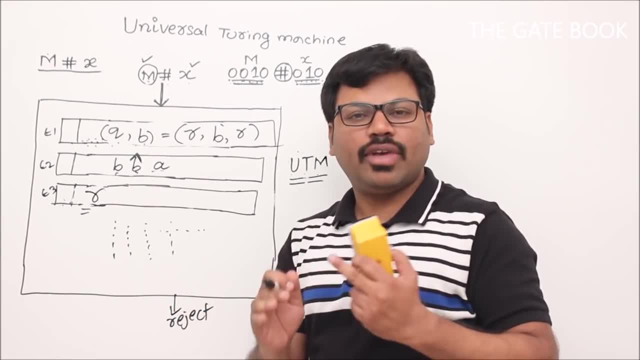 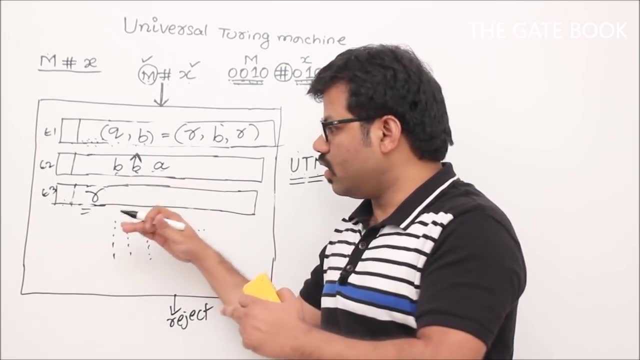 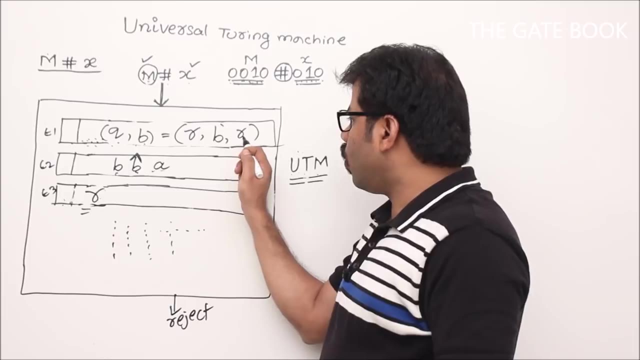 such a way universal turing machine's code is designed, though i am explaining in a very lengthy way, but because i'm going to teach you lot of details here, okay, but after you know end of the session, i will summarize everything, don't worry. so then, what to do after writing r. we have to go right. right, this is right symbol, sorry r. 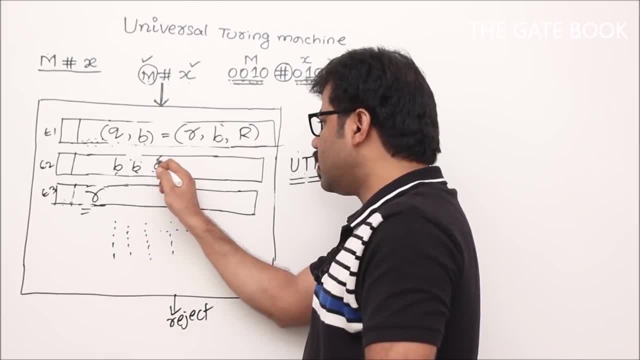 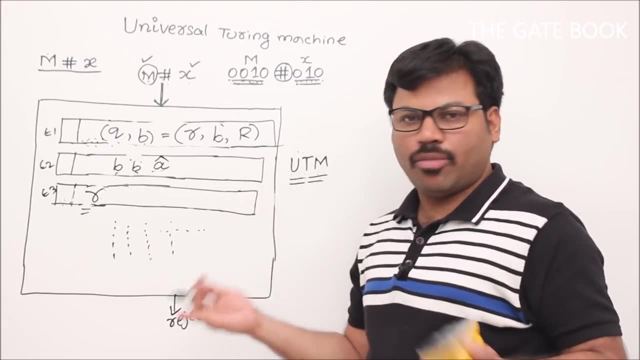 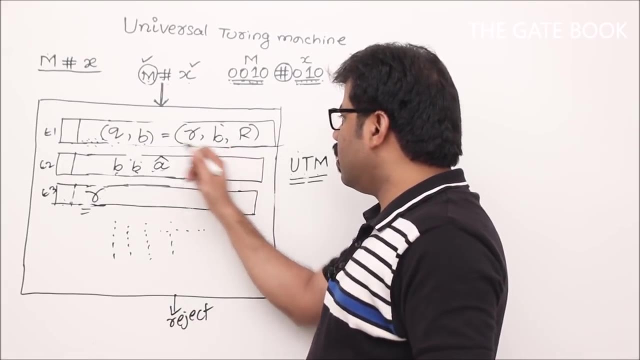 that means the next input we have to scan is this one. then put a mark like this, for that there will be very lengthy code. there is a lengthy code in universal turing machine. i'm not showing it, but i'm explaining how that. what is the functionality of that code? after that it will, you know. did it modify this? 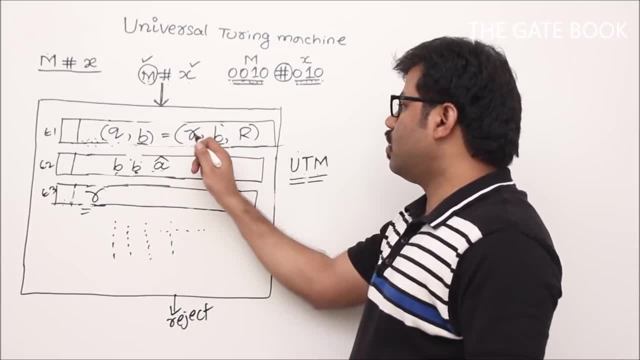 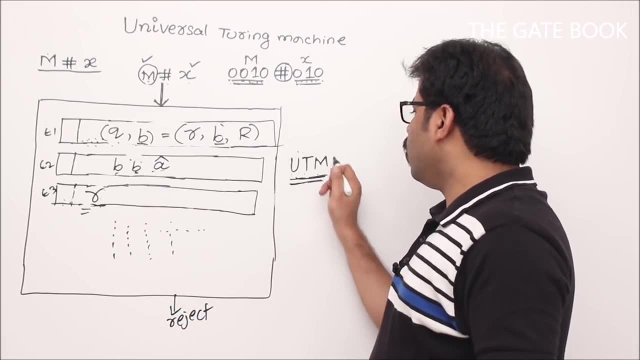 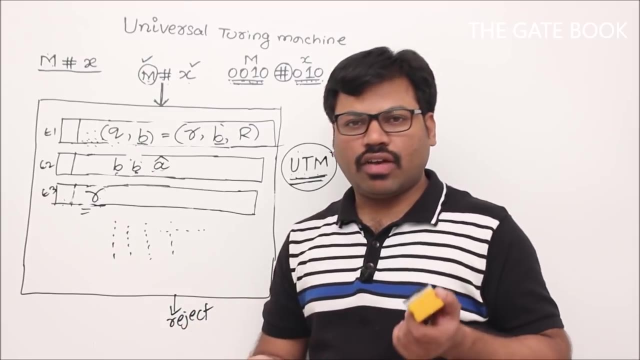 input symbol. no, that's why b is b, after that state is r, then it will go to the next step in that way. finally, what this universal turing machine is doing. universal turing machine is simulating the code of this turing machine, m. okay, sir. finally, what it will do, sir, after simulation: 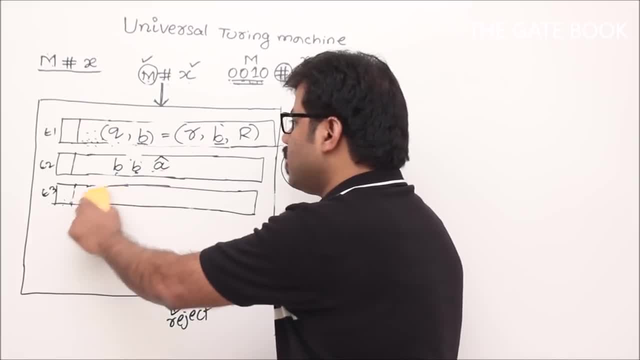 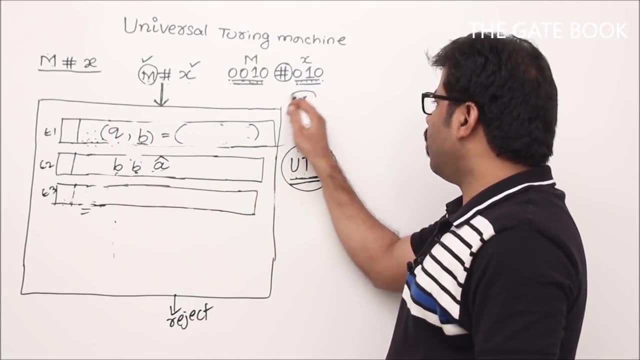 example, after you know, whenever this turing machine example, let's say after something happens at any point of time, let's say, your turing machine- i'm talking about m, your turing machine m comes to final state t, then your universal turing machine will, finally, will stop the. 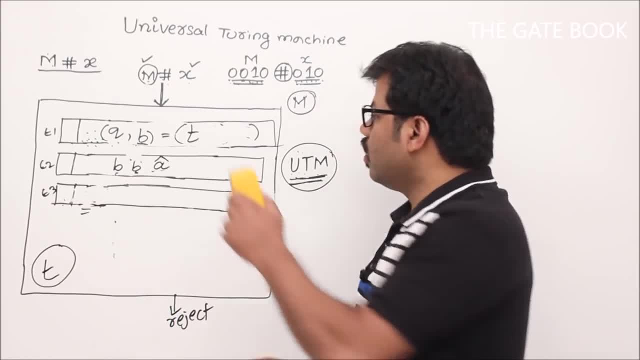 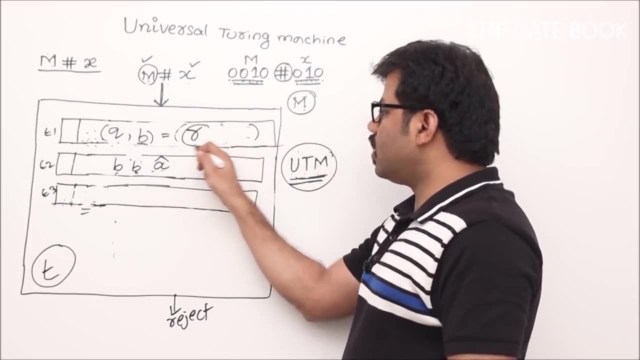 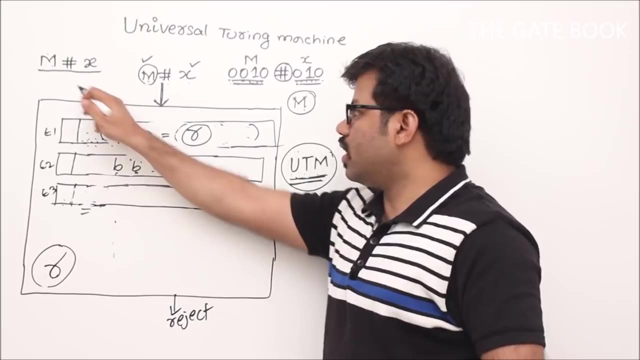 execution and it will say: i am also final. okay, at any point of time, if you are after simulation of your turing machine m, if the turing machine comes to reject state, then your final universal turing machine also comes to reject state. sir, what if your turing machine m, which you have binary form? 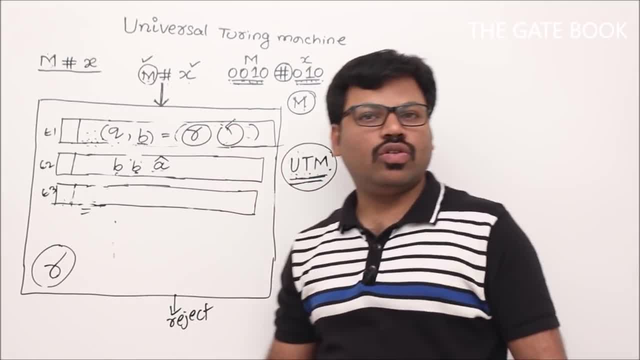 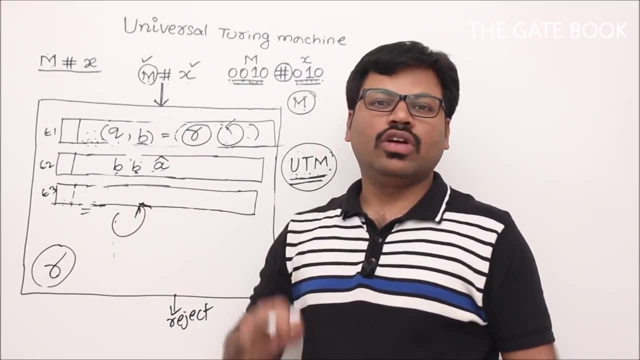 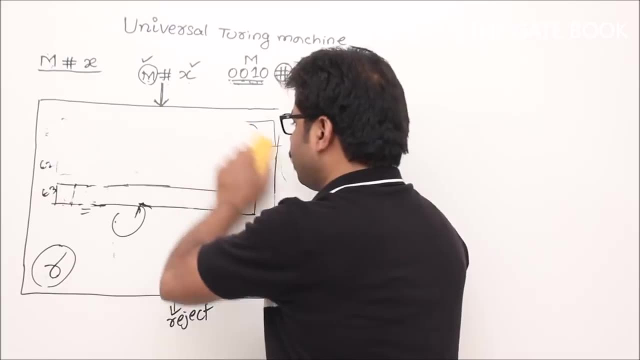 if that is in loop, what your universal turing machine is going to do, we don't have any clue. we also will be busy simulating that turing machine and we will be in loop. so let's try to understand the final behavior of universal turing machine. okay, let's summarize. so your universal turing. 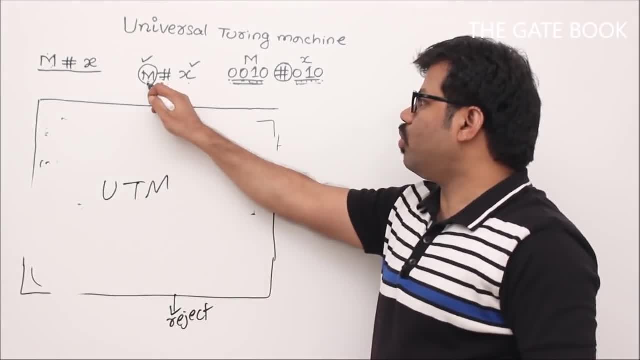 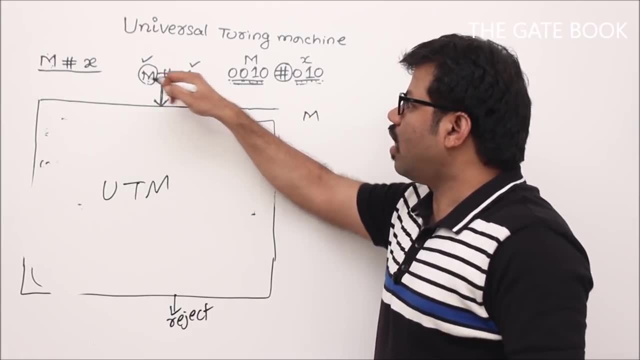 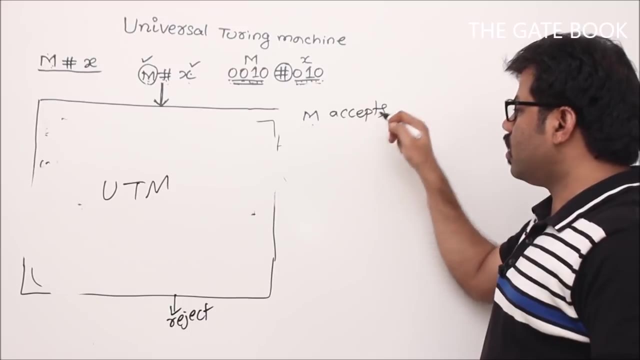 machine is having a functionality such a way that it will take input m hash x, correct. after that it is running m on x. sorry, it is running x on turing machine, m, correct. okay, if m accepts x after simulation, your universal turing machine is simulating m on x. if m accepts x, what your? 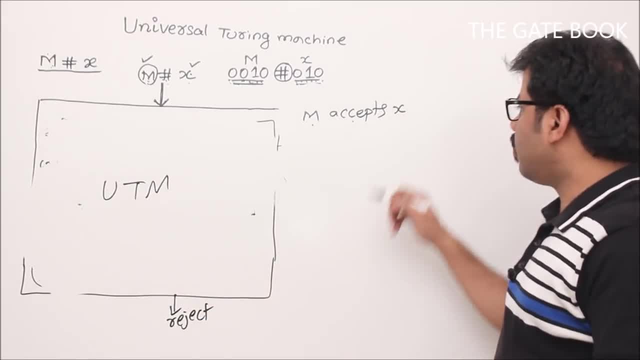 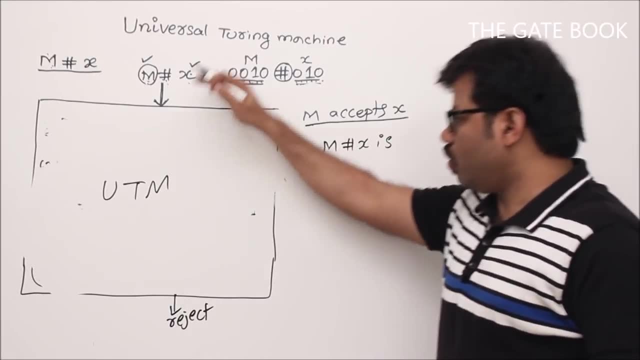 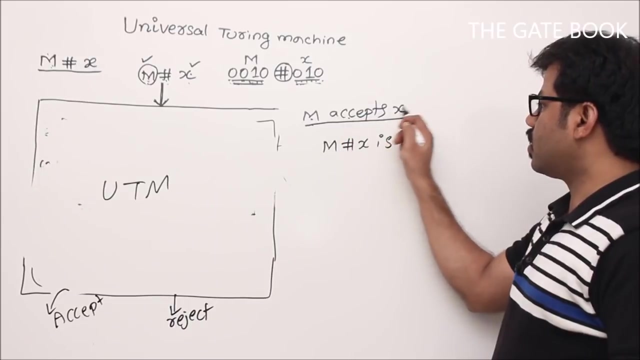 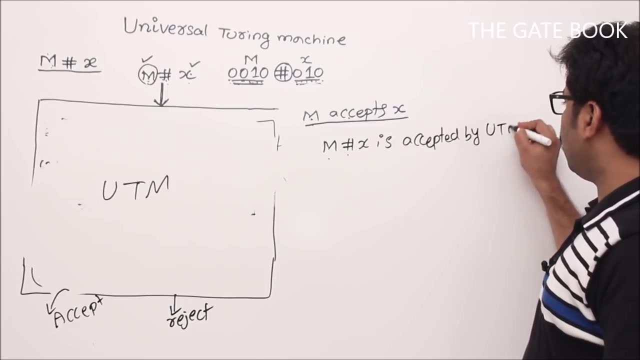 universal turing machine is doing. it is coming to final state. that means what? if m accepts x, then m the input for your universal turing machine. so your universal turing machine is going to accept okay, yes, m accepts x, then m hash x is accepted by, accepted by universal turing machine. remember it. 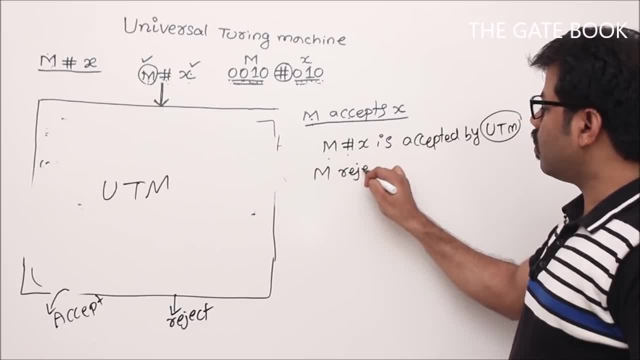 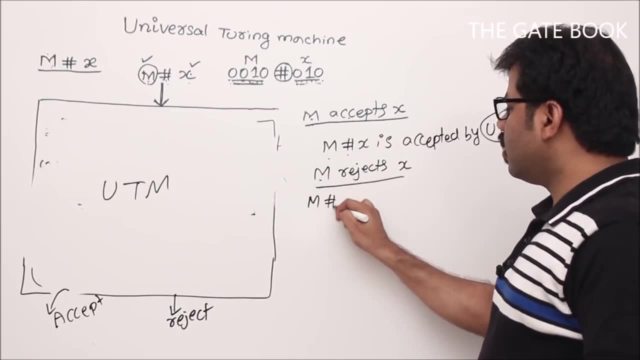 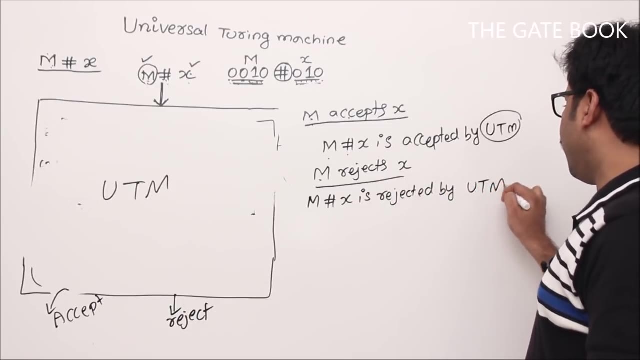 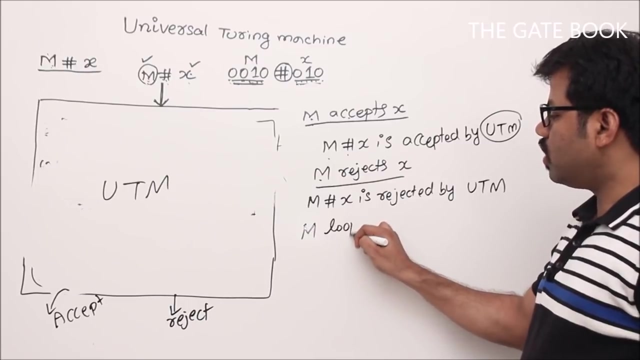 next, sir, if m rejects x, really m rejects x, such a turing machine is m. then m hash x is rejected by, rejected by your universal turing machine. that is the behavior of universal turing machine, sir. if m loops on x, m loops on x, then your universal turing machine are also going to loop, right then on m hash x. 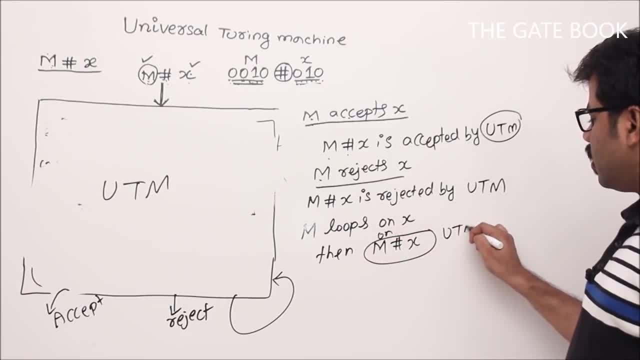 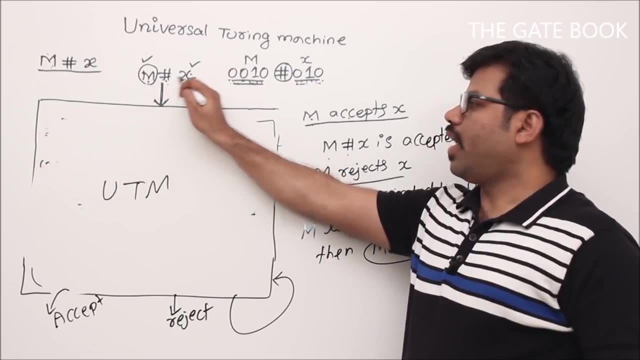 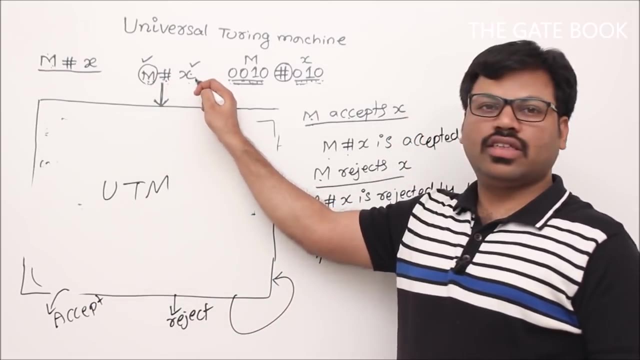 on m hash x, universal turing machine loops. that is the summary of universal turing machine. very simple: it takes input m, hash x. if m accepts x, universal turing machine accepts it. if m rejects x, then universal turing machine rejects m hash x. if m loops on x, then your universal turing machine. 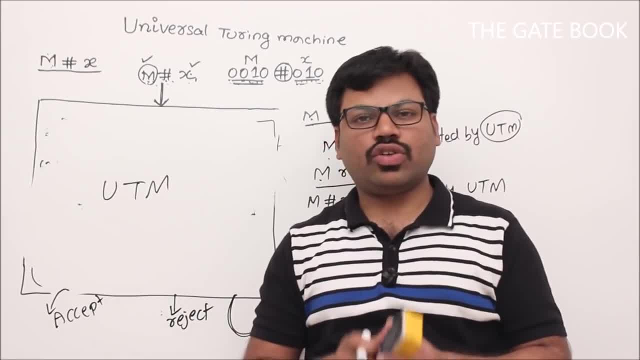 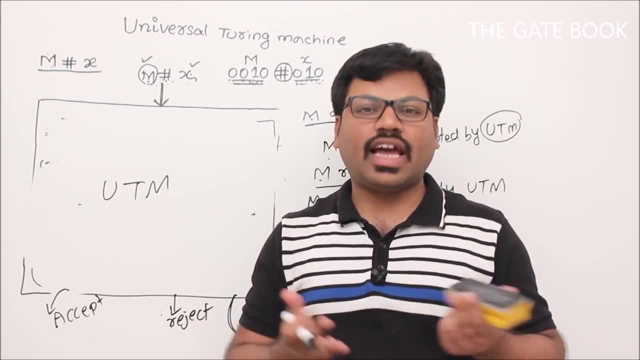 is going to loop. that is about functionality of universal turing machine. remember it. now question: what is the language accepted by universal turing machine? sir, i want to know the language accepted by universal turing machine. very simple: go to accept state when it is accepting this line. 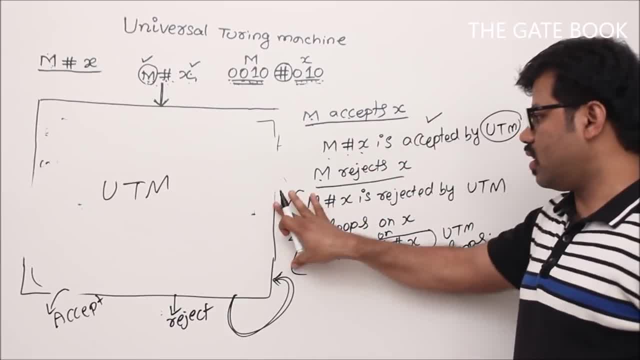 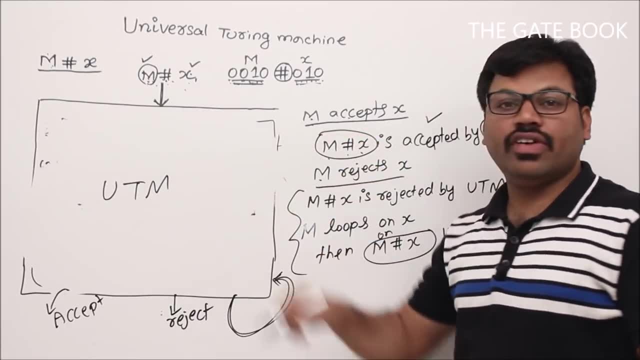 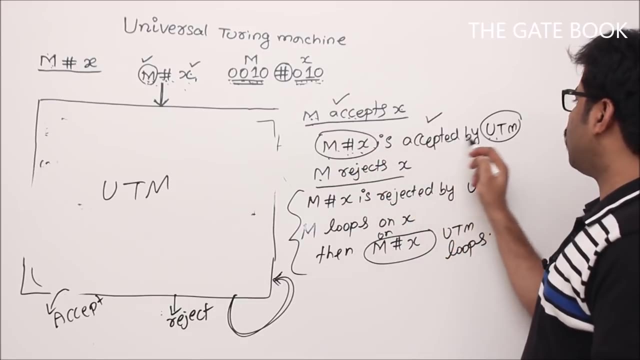 you read this line because this is about rejection. we don't bother about rejection. what it accepts. your universal turing machine accepts m hash x patents whenever m turing machine accepts xc. if m accepts x, then m hash x is accepted by universal turing machine. now let me show a bag. this is the bag of strings: all m hash x. 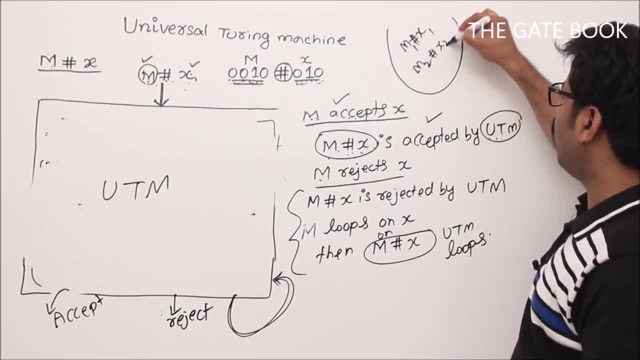 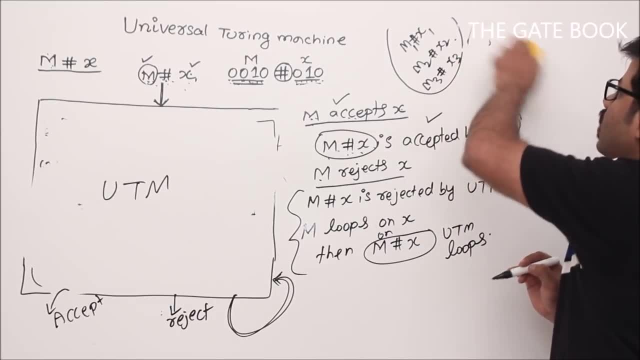 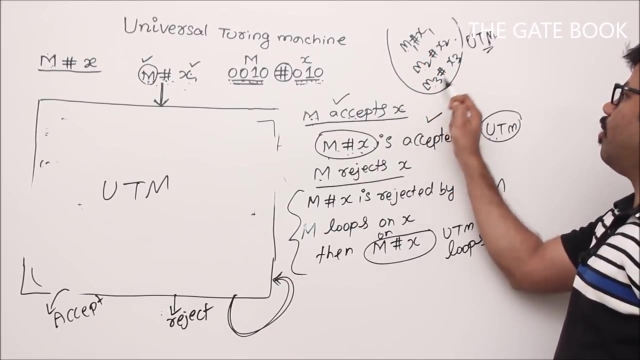 m1 hash x1, m2 hash x2, this kind of all these patterns forms a bag. So this bag is accepted by all. these strings are accepted by universal Turing machine If, and only if, m1 accepts x1, m2 accepts x2, m3 accepts x3. Such a language is universal Turing machine. Now let me write. 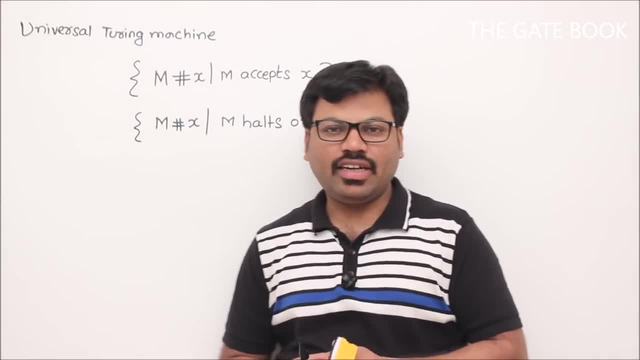 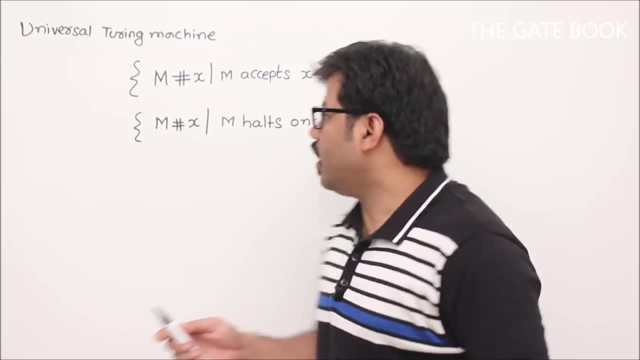 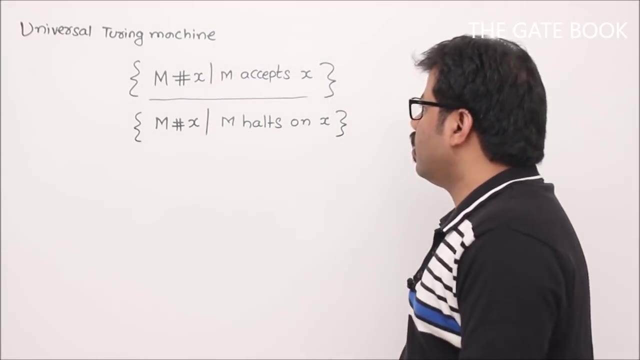 in a clear form. We have seen universal Turing machine. Now what we do is we do the same thing. We try to understand the things with language form. Example: this is a language. Now, generally we describe a language like this. What kind of language it is? First we see It is nothing. but. 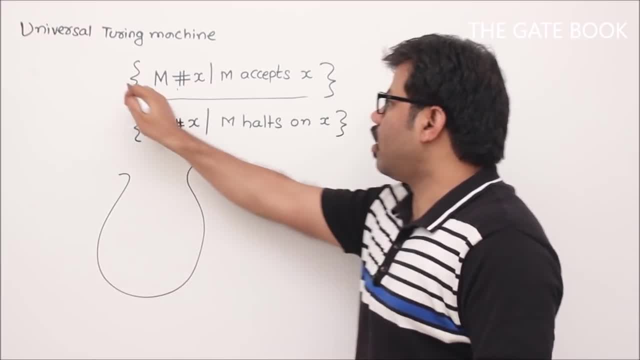 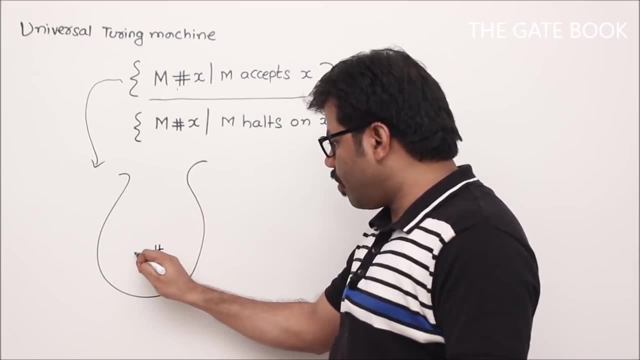 it is a collection of strings, So I am talking about this one. What kind of strings? Any strings. they should have: hash and some binary format m, some binary format x. Is it enough? No, there is a condition. What is? 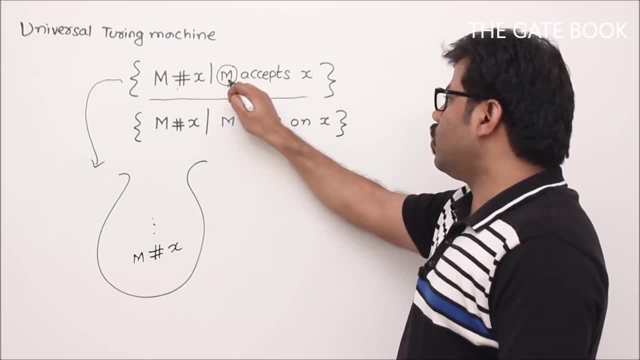 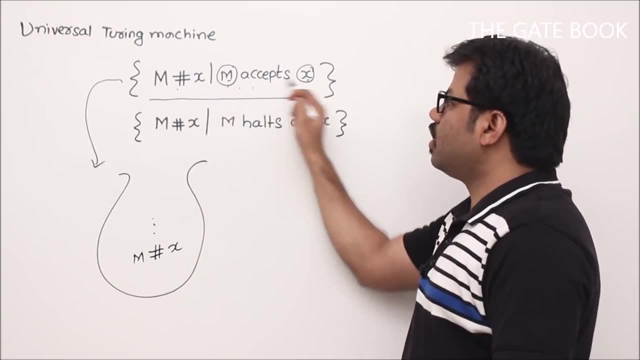 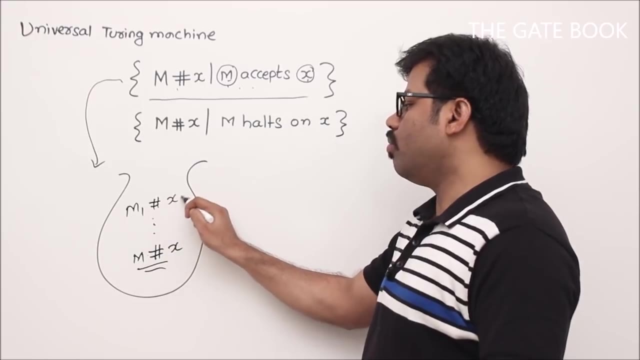 that If it is a Turing machine code, m and m is a Turing machine code and x is input on this Turing machine. if this input x is accepted, that means m accepts x, only such patterns we are taking Example. let us say there is a pattern called m1, hash x1, but 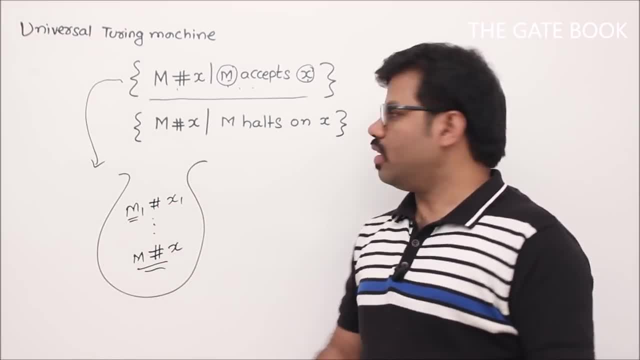 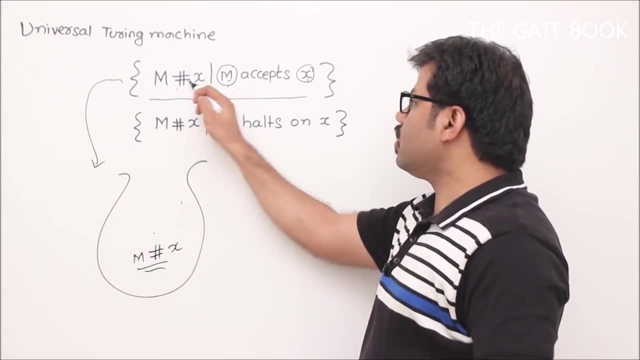 m1 is not at all a Turing machine code, Then you are. I mean then definitely this language is not having that string as a member- correct, Because we need patterns where this m should be: The first component should be Turing machine, second component should be input, and that. 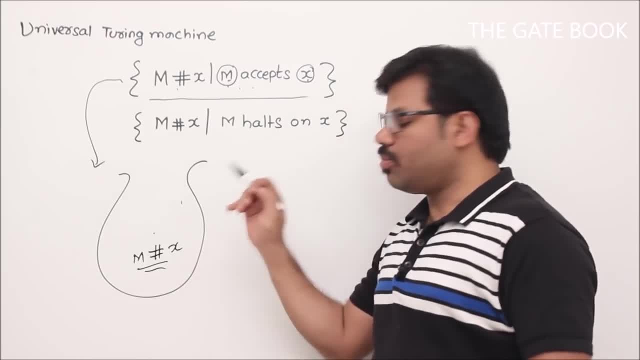 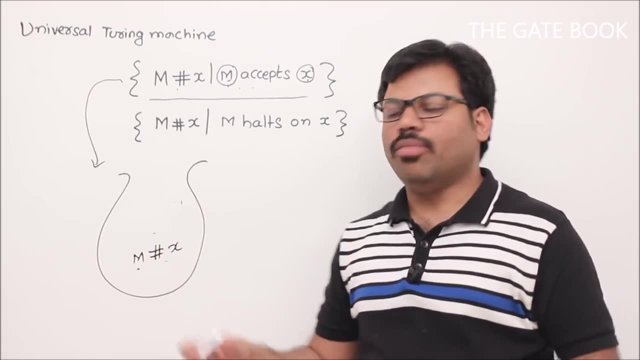 input should be accepted by the Turing machine, Then only such patterns we are taking. okay, It looks like we have only one pattern. It is not one pattern. It is covering infinite patterns, Who knows. But every pattern should have a property. What is that property? It. 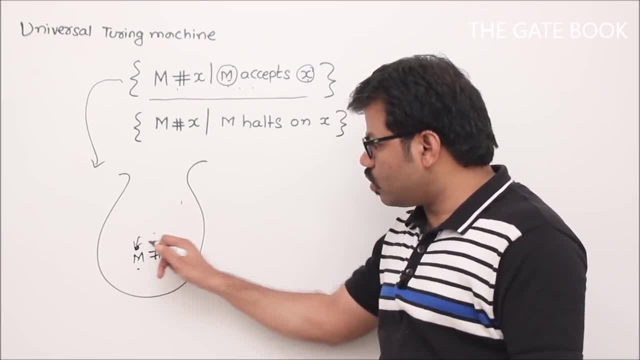 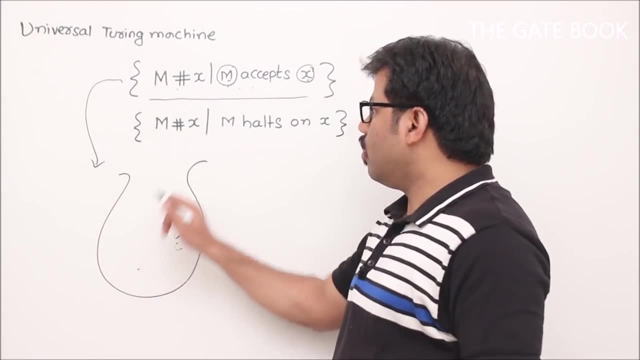 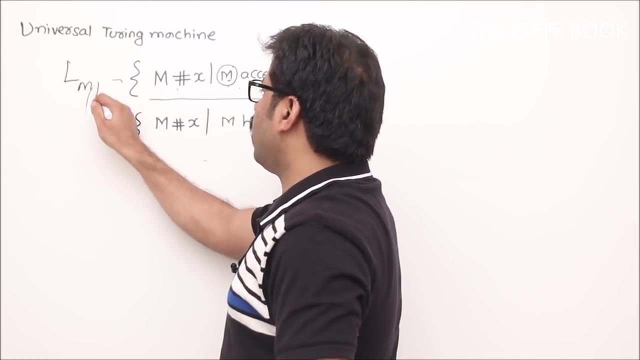 should be a Turing machine code and such Turing machine code should accept x, Then this is a language. right Now, the question is: Finally, you understood that this is a language, correct? Let's assume that this language's name is membership problem. okay, Because we are checking whether M accepts X or not. This is. 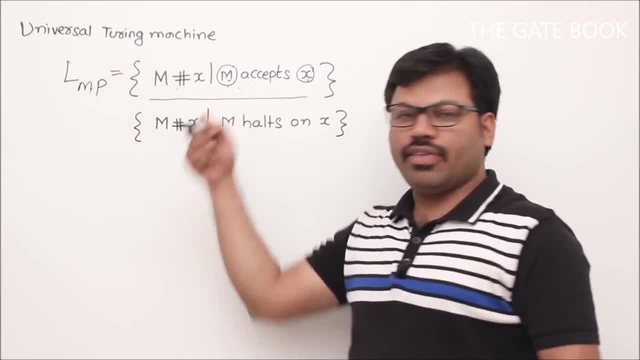 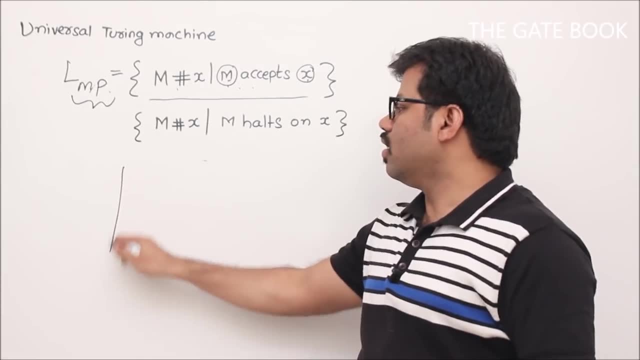 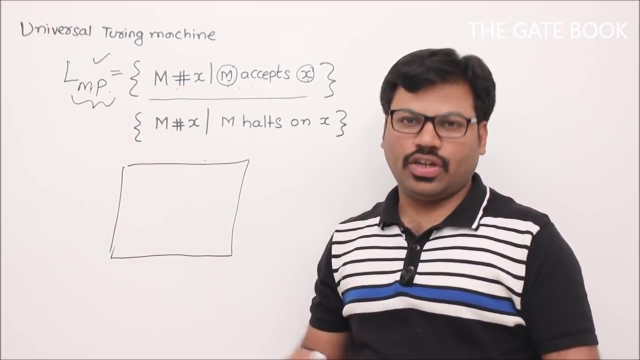 also known as membership problem. Let me ask a question in a different way. Is there any Turing machine for this membership problem? Obvious, yes. How you design, That is what universal Turing machine does, correct. So, yes, I can say that this language has a Turing machine, universal. 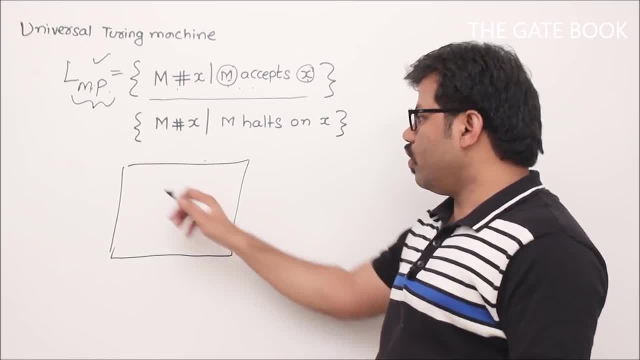 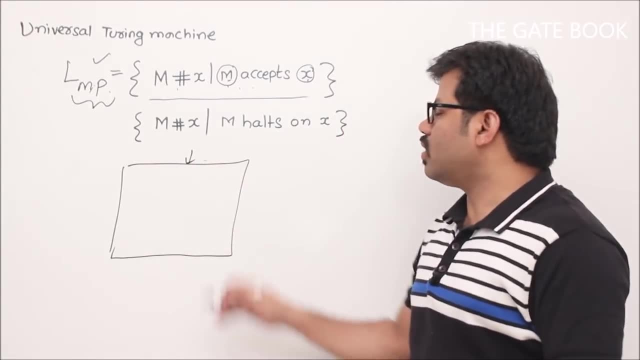 Turing machine. Well, let's recall what it did. What we do is how to design a Turing machine we do from scratch. Forget about universal Turing machine. start from fresh Example. someone asked: can you design a Turing machine for it? Yes, I can design. How Simple You give. 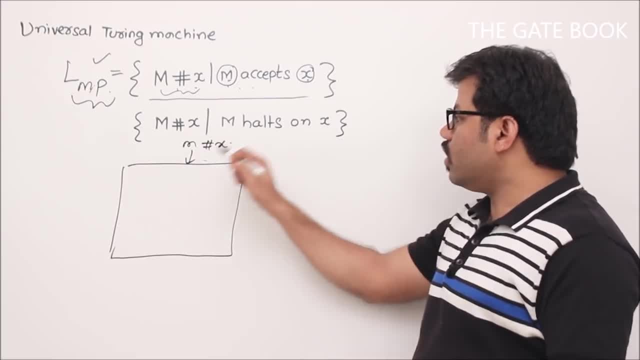 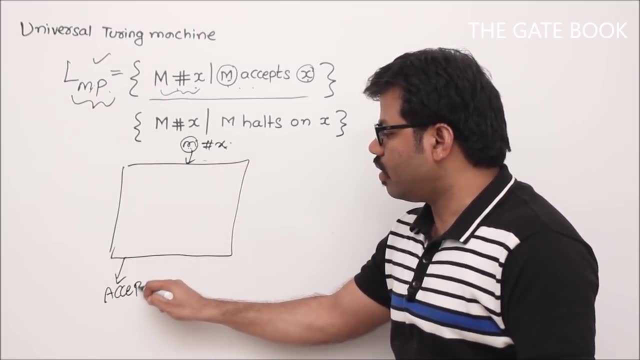 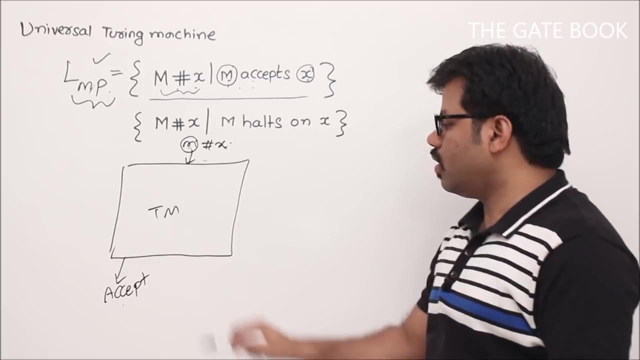 me input: M hash X. What is the question? If this Turing, if M is, if M accepts X, you should accept, correct. First I am writing the requirement, correct What kind of Turing machine you want. M accepts X, then M hash X should be accepted, And other thing: anything Then for remaining. 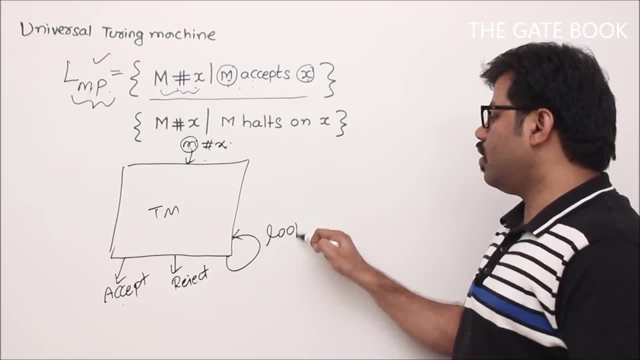 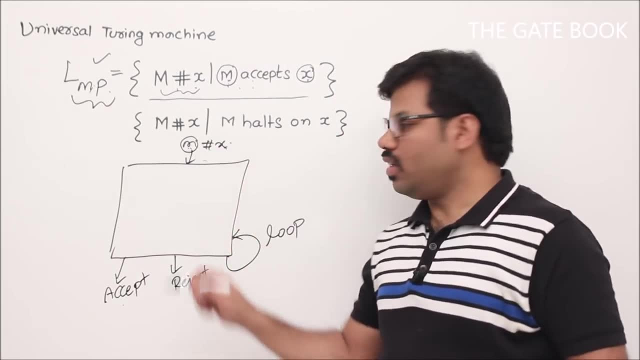 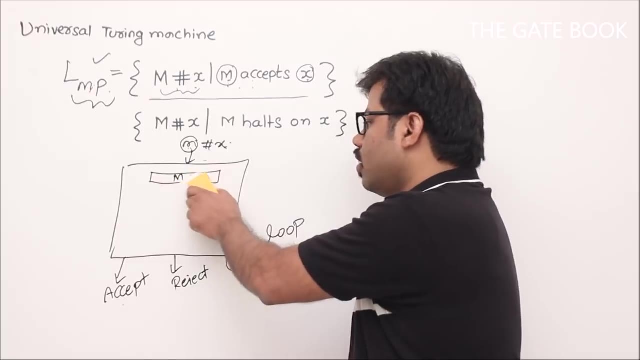 inputs you can reject, otherwise loop. okay, That is a property of Turing machine. Can we design it? Yes, How you design it, I will tell you. Whatever the input is given, I take it into one of the tracks. okay, M, hash, X. Then after that, slowly, that means I am explaining my Turing machine code. 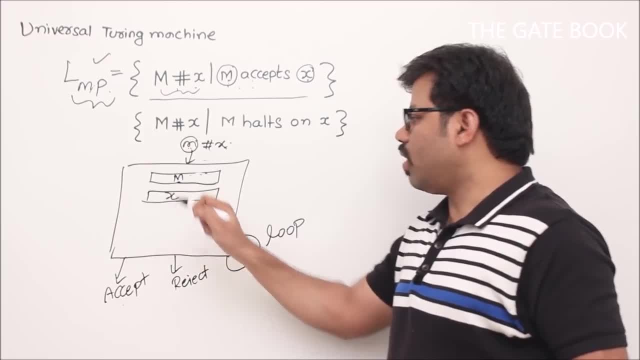 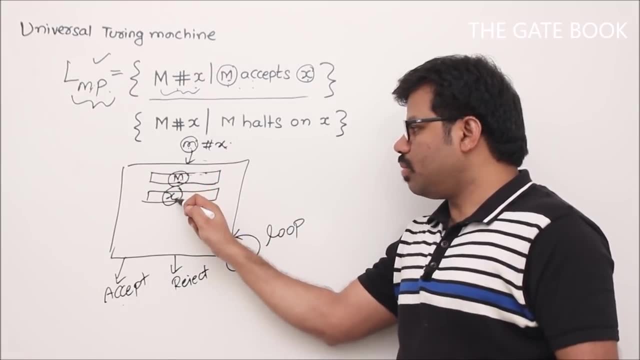 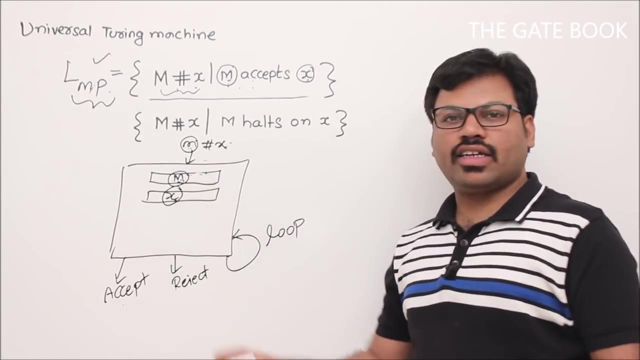 I take M here, X here. Now, from now onwards, I don't go into details, I say simply: I simulate M on X. If M accepts X, definitely that code. by understanding the code, I can understand. If M goes to final state on X. 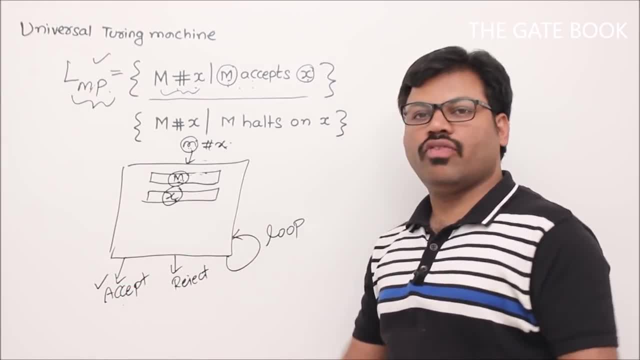 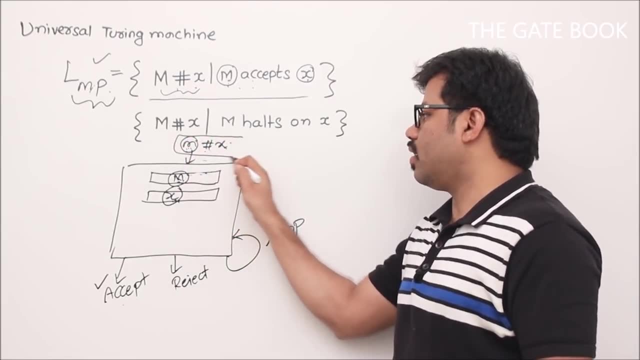 then I go to final state and I accept the string. Which string you are accepting X? No, If M accepts X, I am accepting M hash X, this entire pattern, So that I am designing a code for otherwise a Turing machine. So I am designing a code for otherwise a Turing machine. So 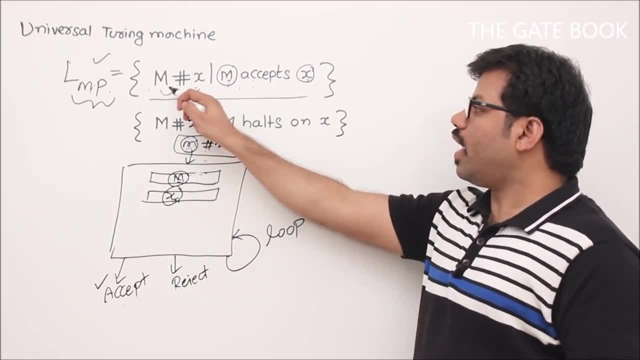 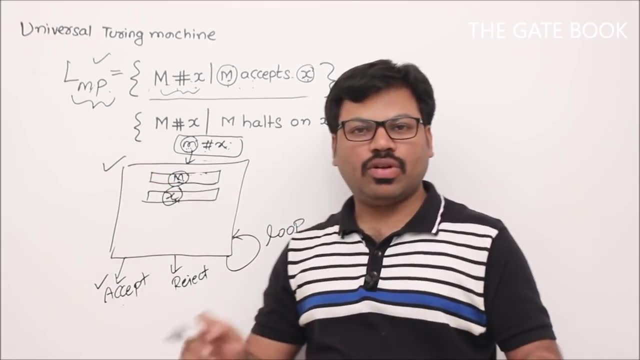 I am designing a Turing machine for this problem. correct, When you should accept. Whenever M accepts X, I should accept M hash X. That is what I am doing. So, yes, such a Turing machine is possible if you carefully plan it. Also, this Turing machine is nothing but universal Turing. 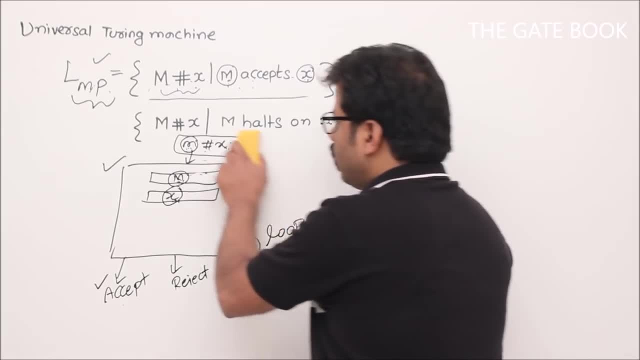 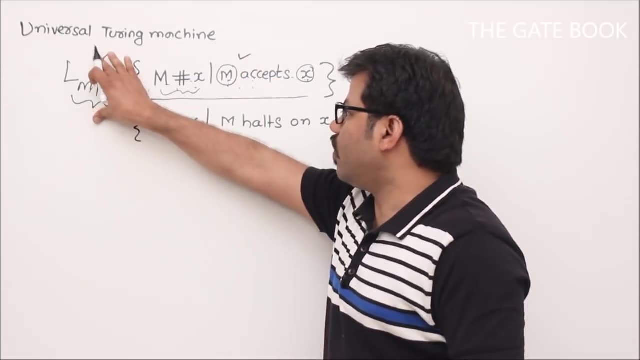 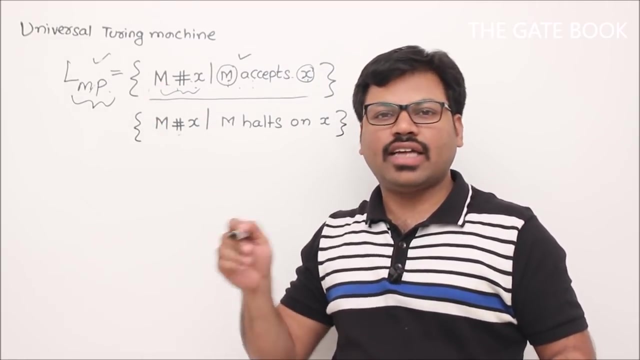 machine which we designed. Now forget about this. now That means finally you realize that for this problem there is a Turing machine. Then this language, if you see this as a language, this language is dash language- then recall: any turing- sorry, any language has a turing machine. then we say: that is a recursively. 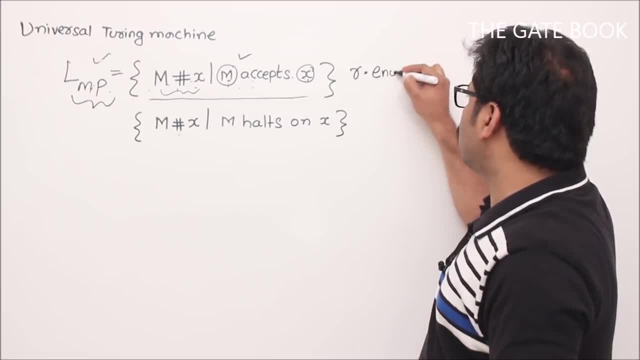 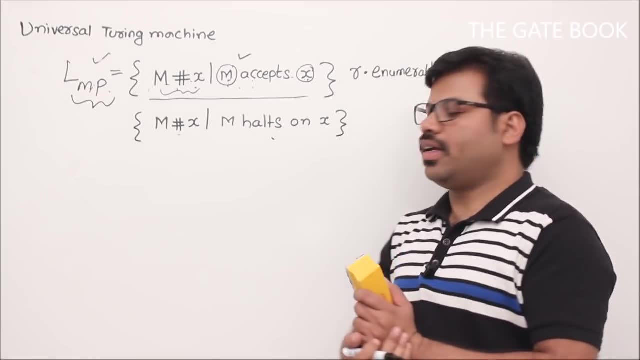 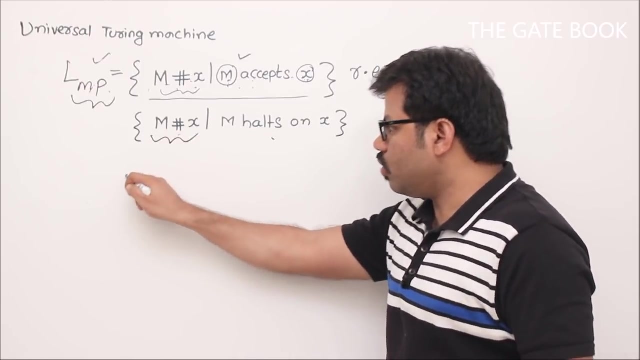 enumerable language. so that's why this language is now recursively enumerable. remember it. now come to this problem. understand this problem and check whether it is recursively enumerable or not. what is the problem? we have to, first of all, i explain you the language here. this language is nothing but collection of strings. any language is collection of strings. what kind of strings? 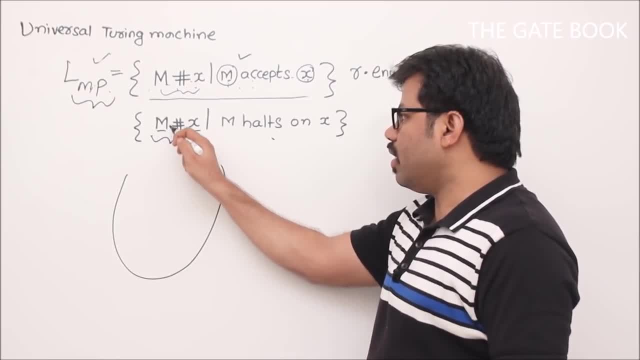 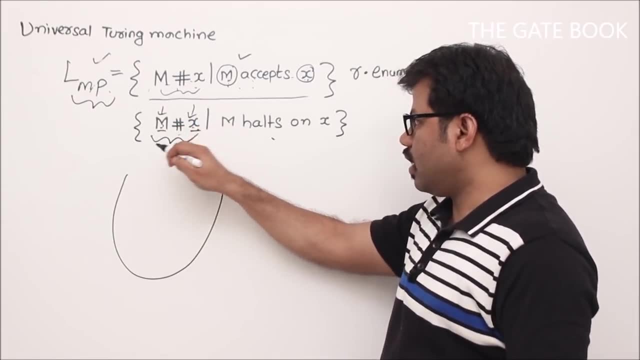 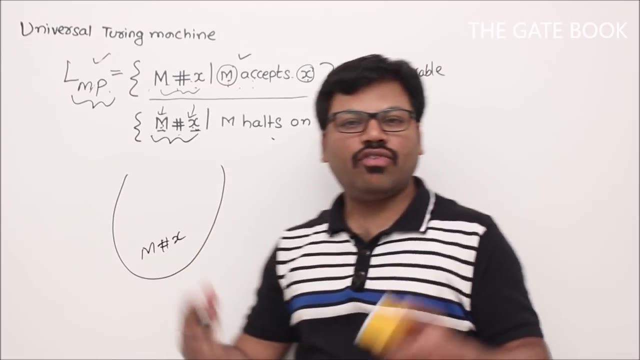 if the pattern is treated as m, i mean component 1 and component 2, and component 1 is turing machine and x is input on input x. if turing machine m halts, then such m hash x you should collect. try to understand in the world there are infinite patterns. any pattern, right like this, m1 hash x1. 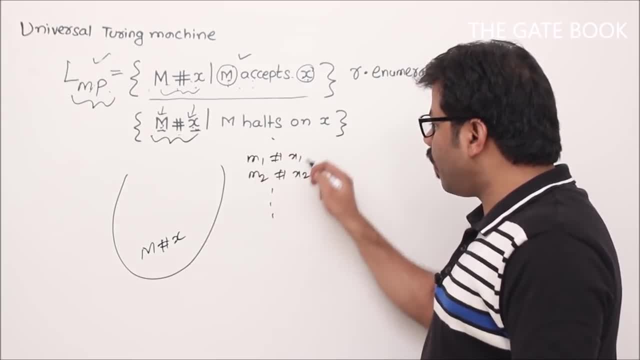 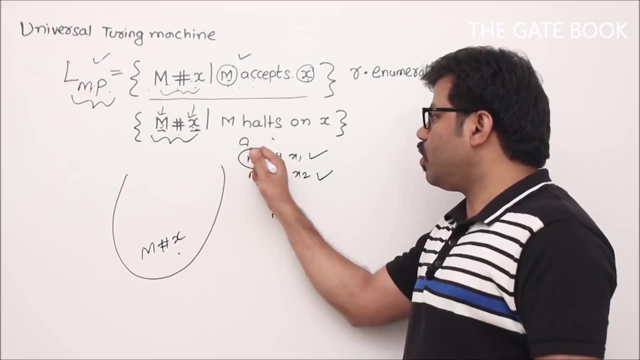 m2 hash x2 in that way. but what kind of pattern is this? patterns we should select in our language. if this turing machine, sir, first of all you tell me why it should be turing machine, what if it is not a valid turing machine code? reject this string. we don't. 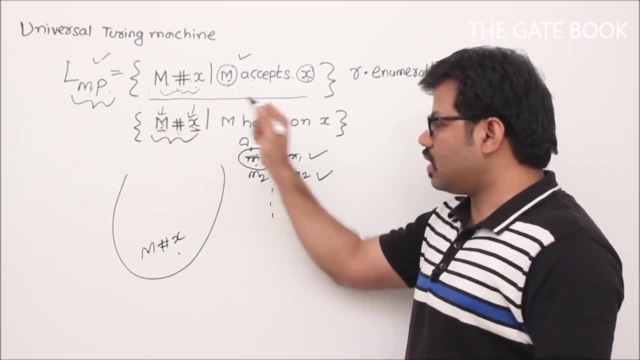 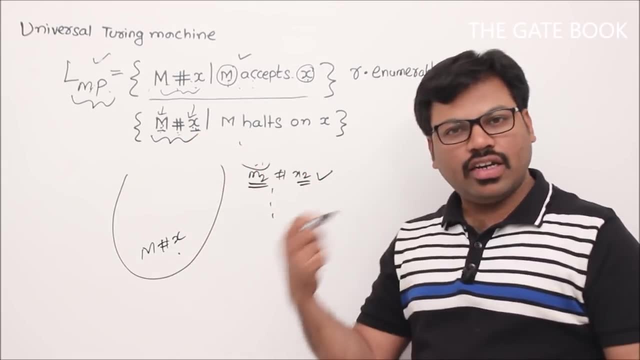 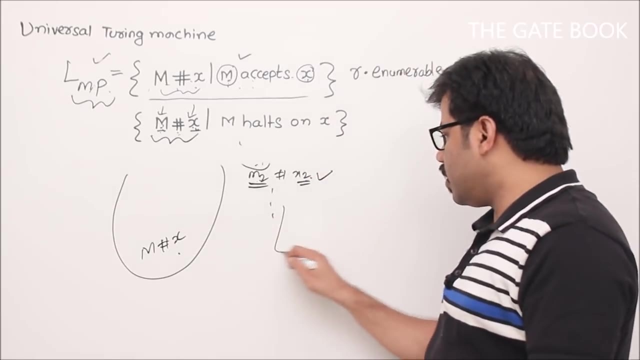 want it. we want a pattern: m hash x, such a way that that should be a valid turing machine code example. let's say this is valid turing machine code and x2 is a valid input, but m2 is not halting on x2. sir, what is the meaning of halting? i have forgotten to tell you any turing machine. 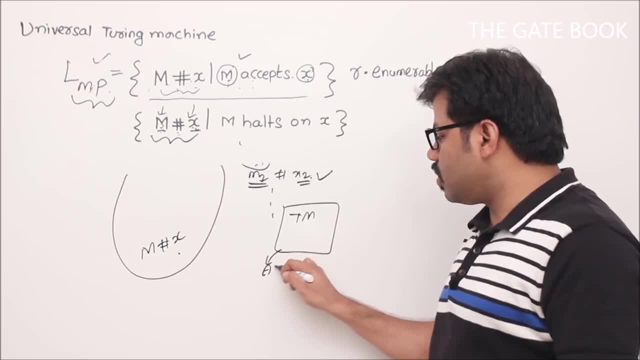 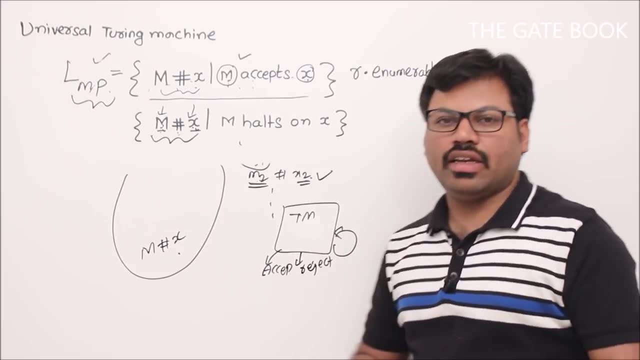 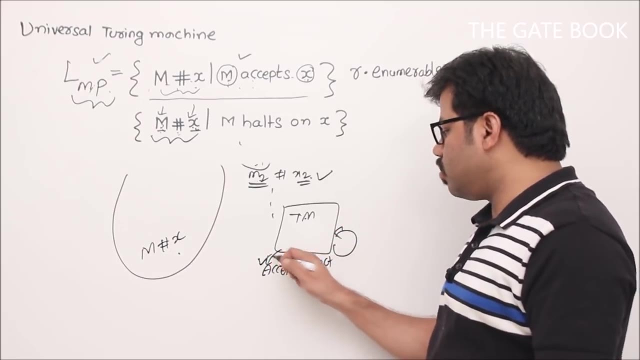 we know what is the behavior, recall: it sometimes accepts a string- general turing machine i'm talking about. otherwise, it rejects. sometimes it goes to loop, isn't it? then we say that if any turing machine accepts or rejects a string, i mean, yes, accepts or rejects a string, rather than loop. 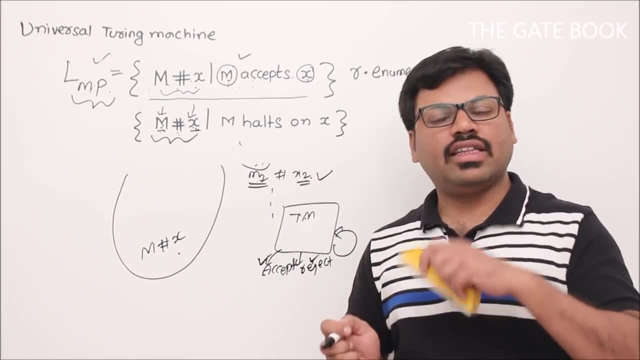 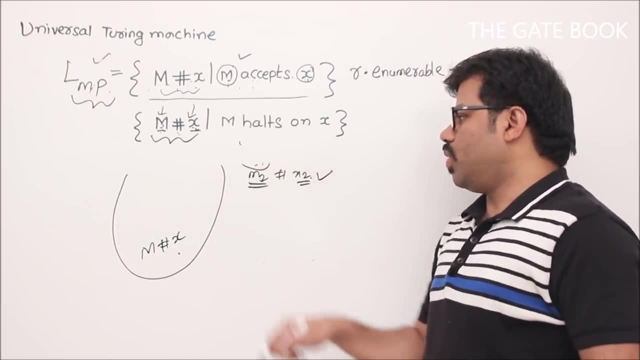 then we say that turing machine halts. halting means either it accepts or rejects. okay, so such state is called halting. now come back to this problem example. let's say you have a turing machine code. valid turing machine code x2 is a valid input one. 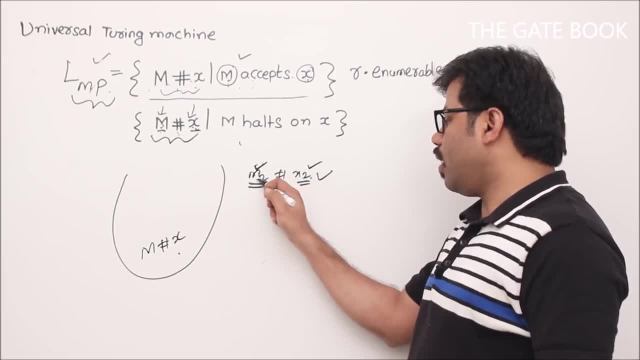 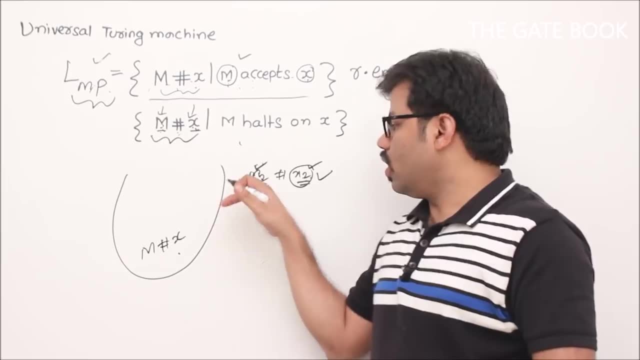 input. now, if you simulate m2 on x2, if you run m2 on x2, then m2 is halting on x2. okay, we have really constructed a turing machine m2 and we gave a input x2. let's give like this: this is turing. 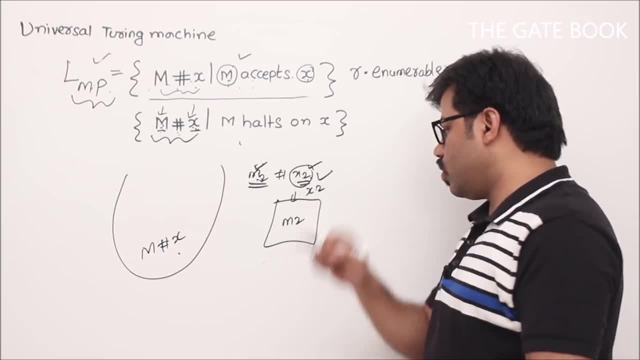 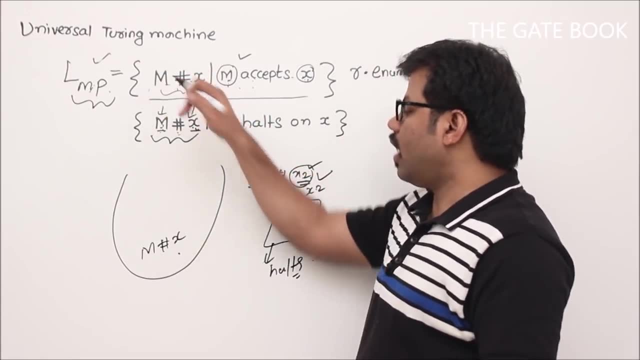 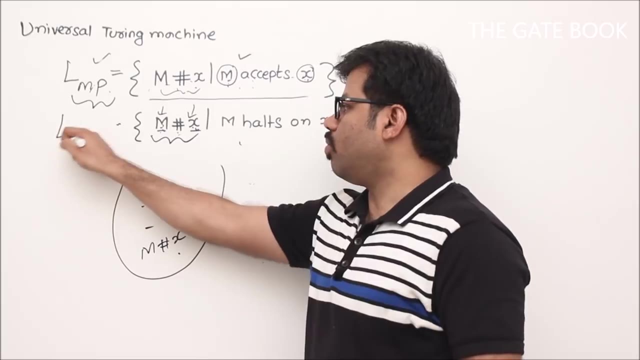 machine m2 and we are in giving input x2 to this one. if really m2 halts, okay, then we have to collect it. m hash x. so tell me finally what kind of strings you are collecting in this problem. second problem, also known as halting problem. in halting problem we are collecting: 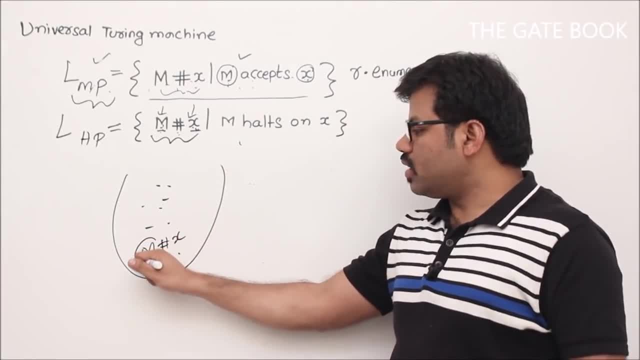 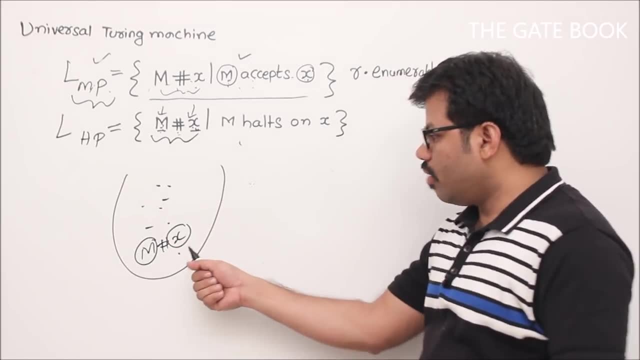 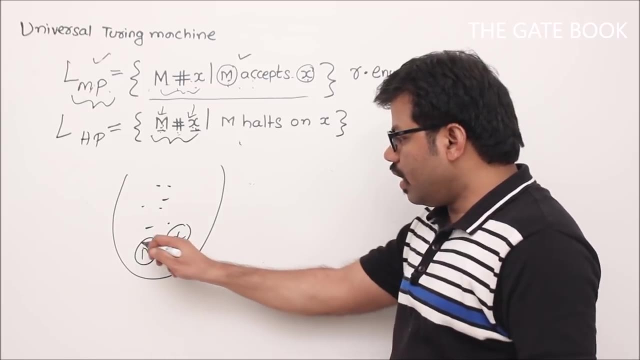 all possible strings where a turing machine m halts an x. okay, so first of all, we'll ask, we'll take interview of one string, my dear string, why are you in this bag? i am, i am a member of this halting problem. what is halting problem really? 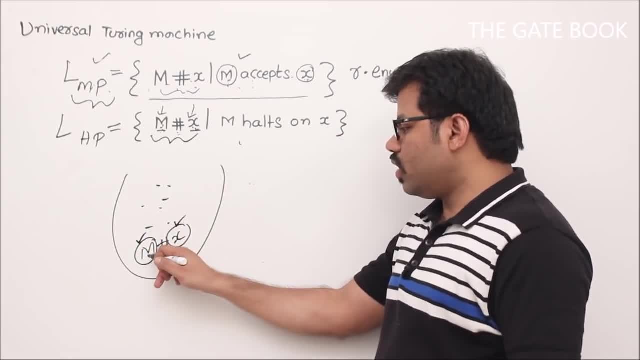 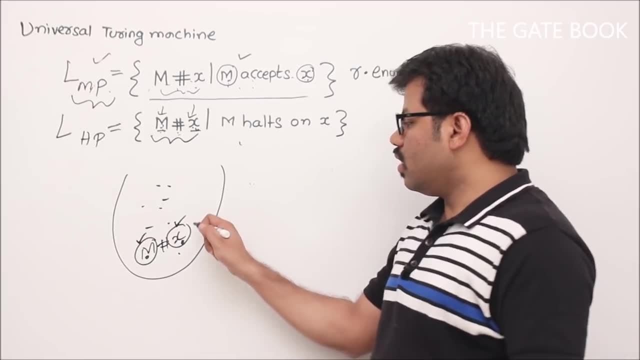 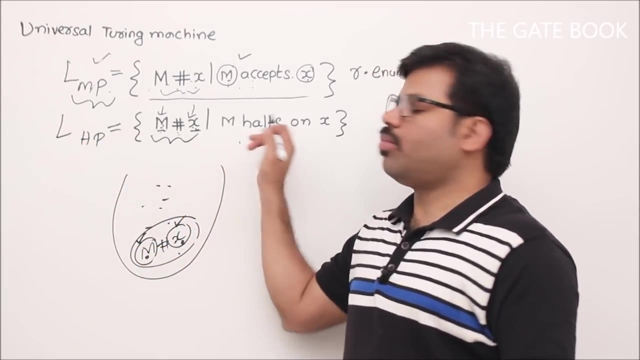 one Turing machine code. this is one input. If this Turing machine halts on this input x, then this bag takes it. That means this: m hash x is a member of this bag if, and only if, this Turing machine m halts on x. That is called halting problem. Now read it: m hash x is a. 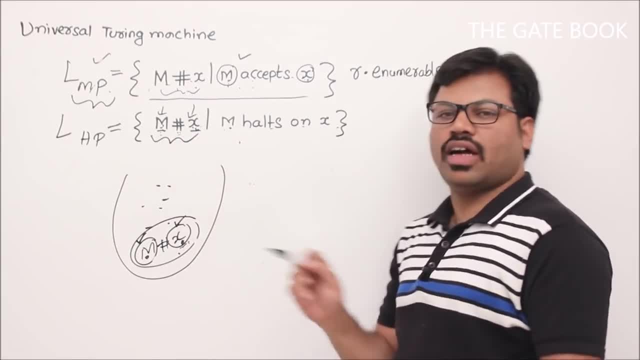 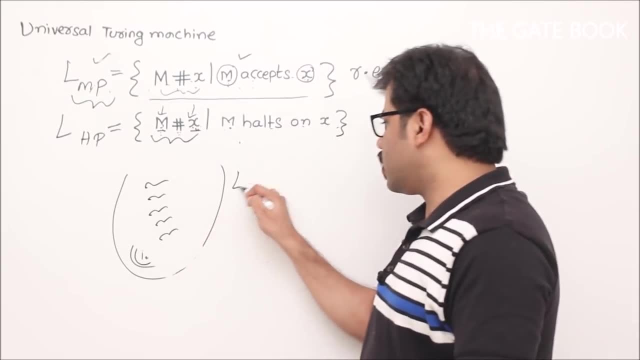 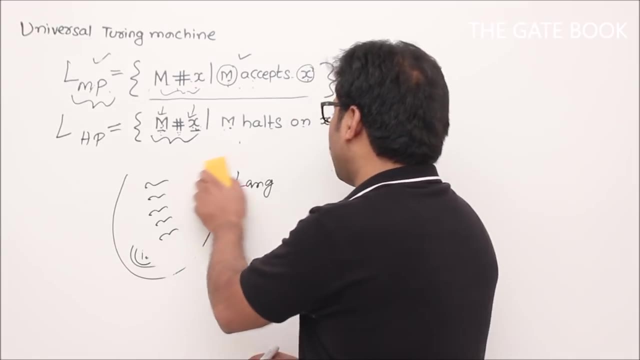 collection in your bag. if, and only if, m halts on x. Understand Now, in that way we collected lot of strings in halting problem, So it forms a language, correct? Now my question is: such a language is recursively enumerable or not? is your question. How to answer it. I will tell you. 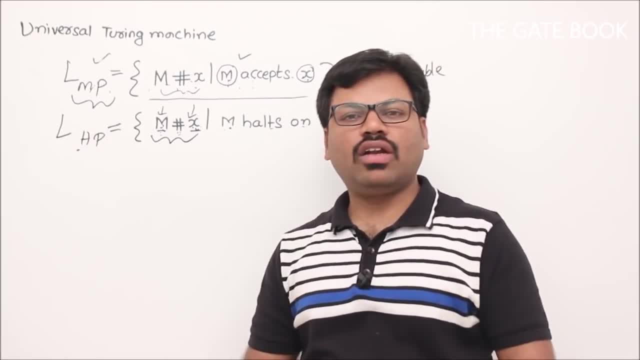 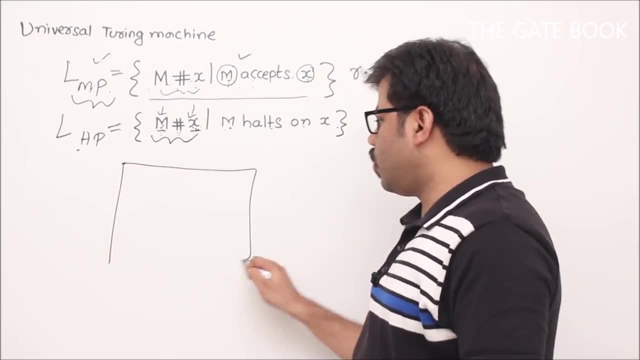 Simple If you want to know whether this language is recursively enumerable or not. only one mantra that is constructed Turing machine. Yes, we will try to do that How I am going to construct a Turing machine for halting problem. you see, Simple. What is the input for? 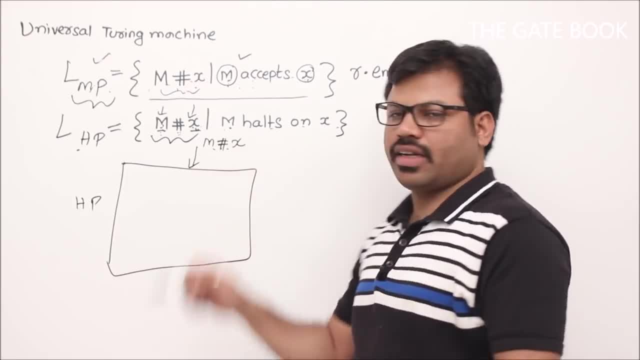 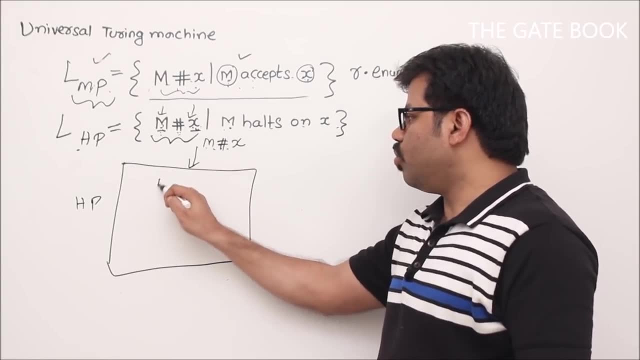 halting problem. Maybe some m hash x kind of pattern correct. Okay, What I do is just read this story, Listen to this story. So I simulate m on x. If really it is a valid Turing machine code, it is a valid. 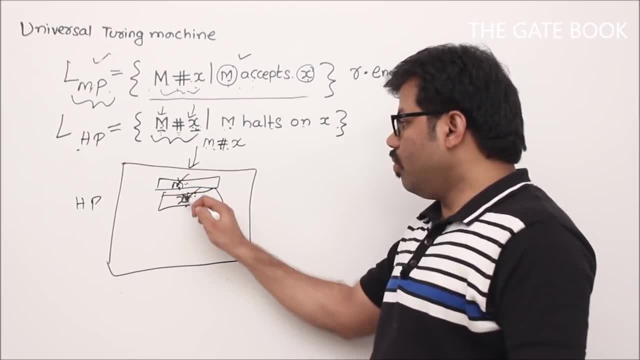 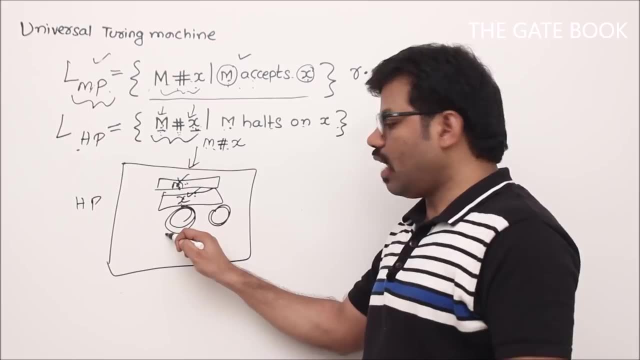 input. I simulate m on x. If m now, while simulating m, either will halt on x, otherwise it will be in loop Whenever m halts on x, then I will know that because the Turing machine m will go to t state. 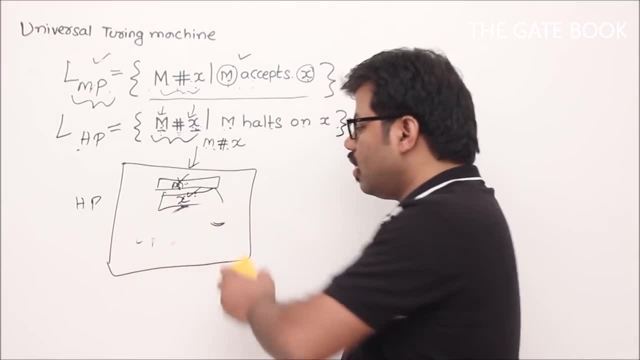 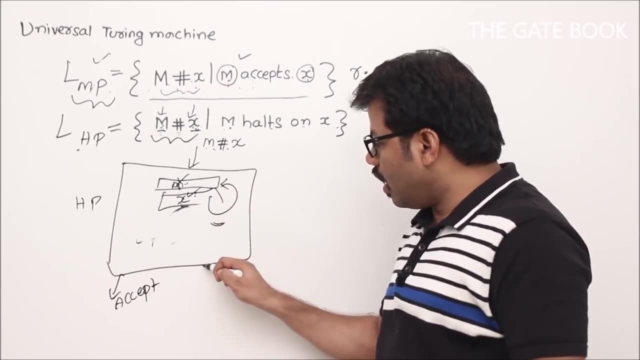 t state or r state. Whenever it goes to t state or r state, then I will accept Such a way. I design my Turing machine. If it is on loop, then I also will be in loop. Okay Now. so see, this one Is it? 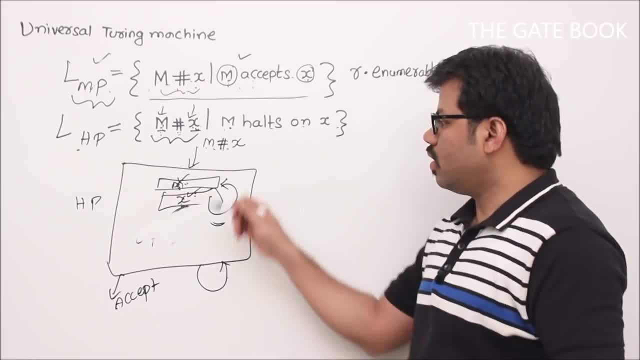 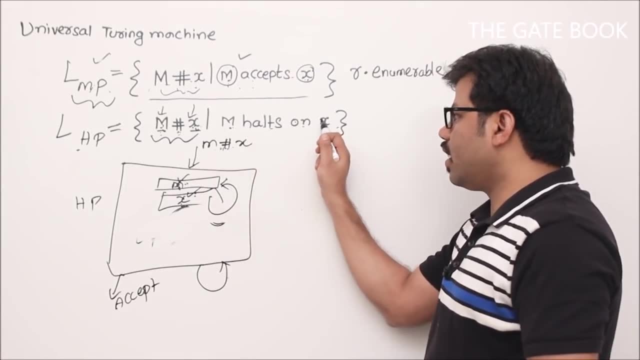 not a Turing machine I have constructed. See Now really why it accepts this kind of patterns. you see, Give a valid pattern: m hash x. Really, m halts on x. we should accept it. correct Now see. 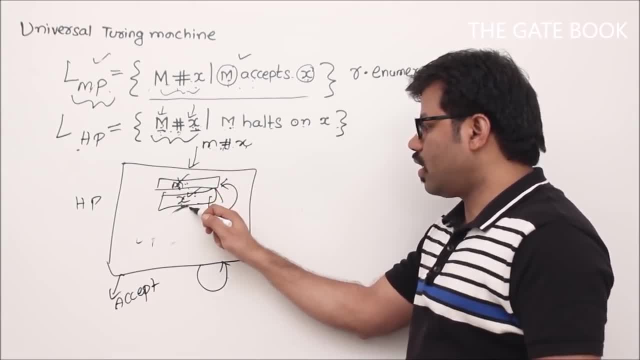 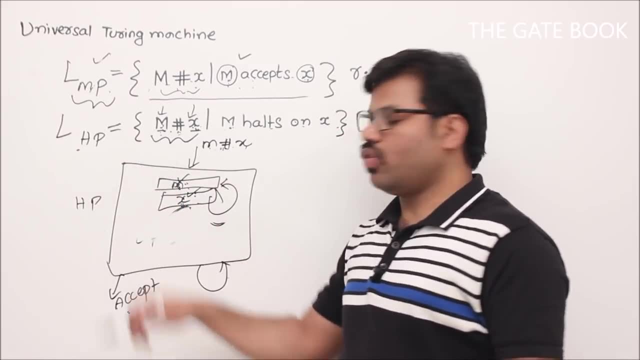 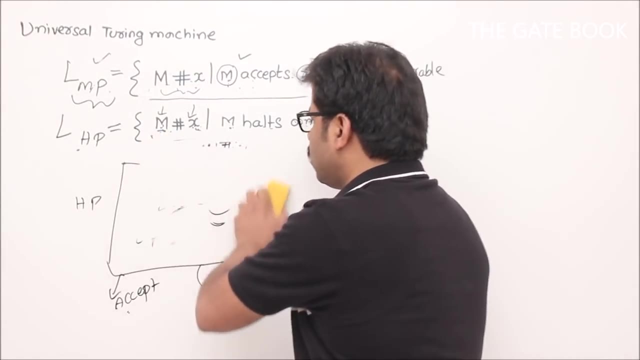 What we are doing actually. we are running m on x, correct? If m halts on x, we are accepting. That means what? Definitely? we are designing a Turing machine which halts on all these possible patterns. Let me focus on this Turing machine one more time to understand it clearly: I am designing a Turing 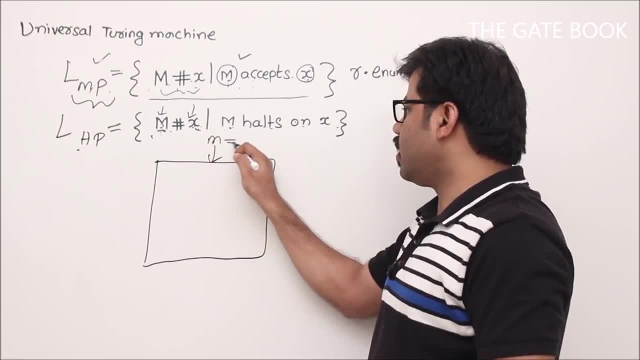 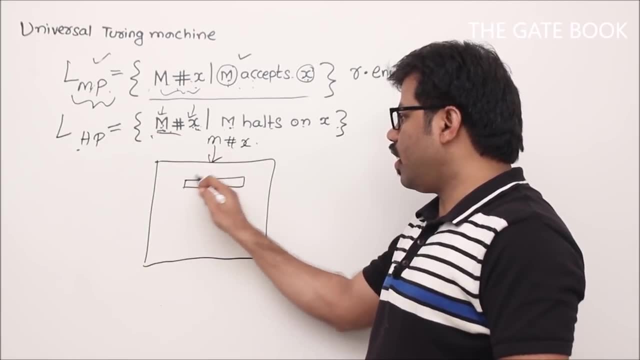 machine such a way that, whatever the input you give, m hash x. see, my goal is, I have to construct a Turing machine for this. So I am designing a Turing machine for this. So I am designing a Turing machine for this language. How I do you see? First of all, I simulate m on x, Like I ask. 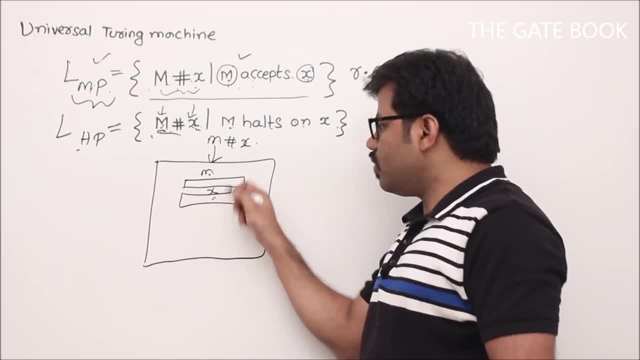 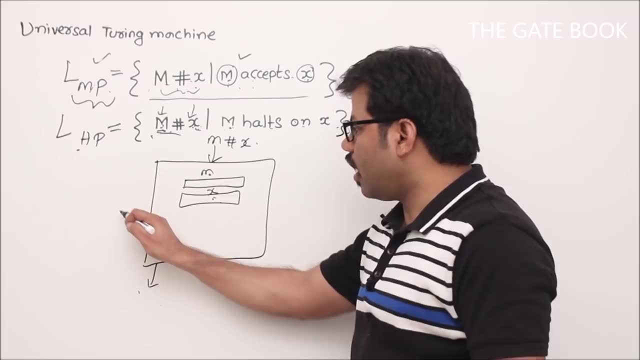 Mr m, do you halt on x? Because if you simulate you will understand that Really m says that, yes, I halt on x, Then I will go to final state. I means halting Turing machine. Okay, Let us say, 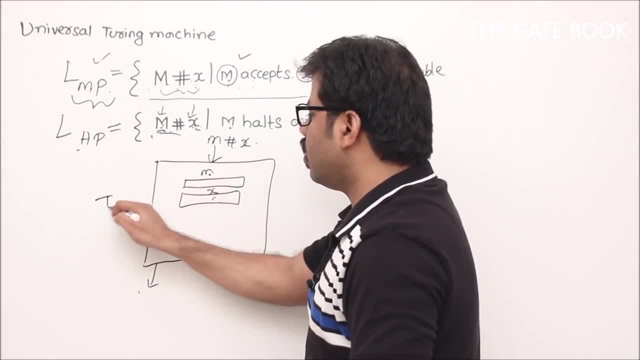 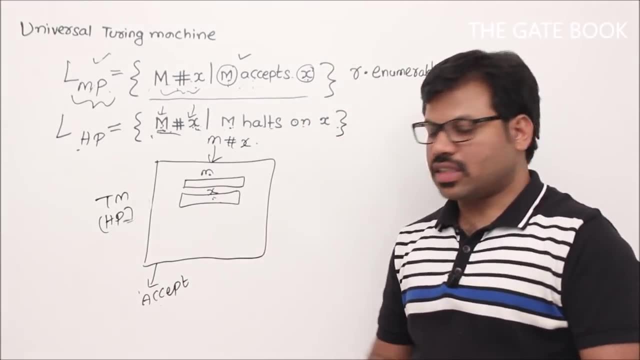 this is halting Turing machine. Otherwise, let us say Turing machine for halting problem. So it will go to accept state. To get the clarity, ask a question: When are you going to accept state if m halts on x? Remember it, Okay. Otherwise, 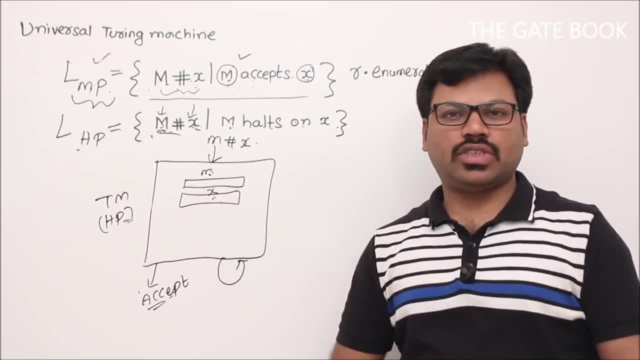 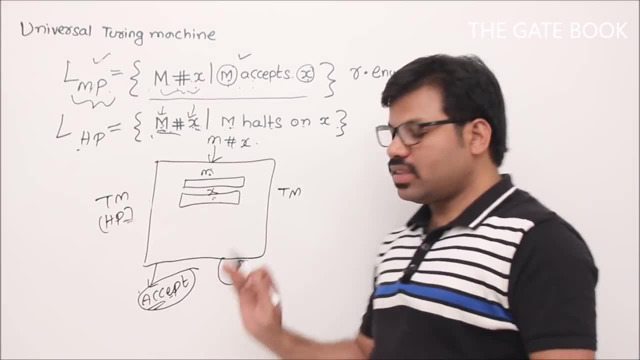 what you do. I will be in loop because I do not go to accept state. Now, this is a Turing machine because there is an accept button. It is not compulsory to reject something. If you have any accept state, that is automatically a Turing machine. Okay, Even you do not require accept. 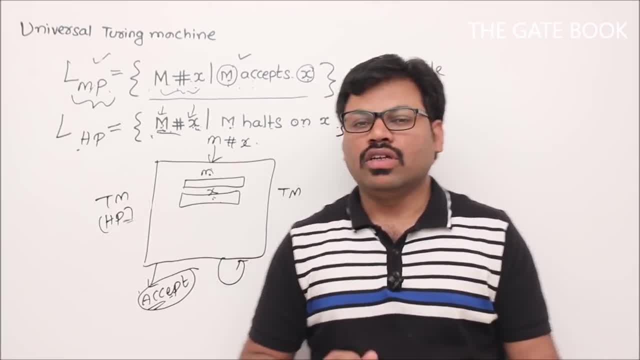 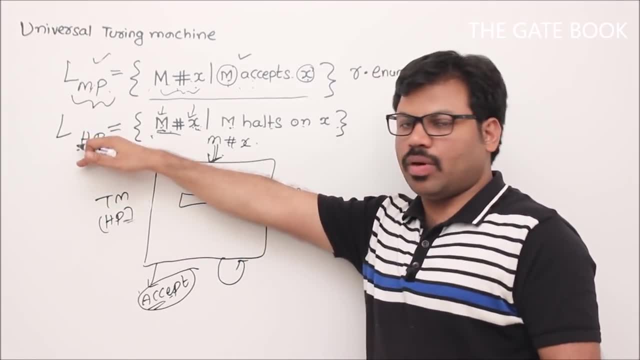 state also: Okay, You know what is a Turing machine, right? So let us begin Why this Turing machine is going to x Exactly, accept this language of halting problem or halting problem. we will see You give any.